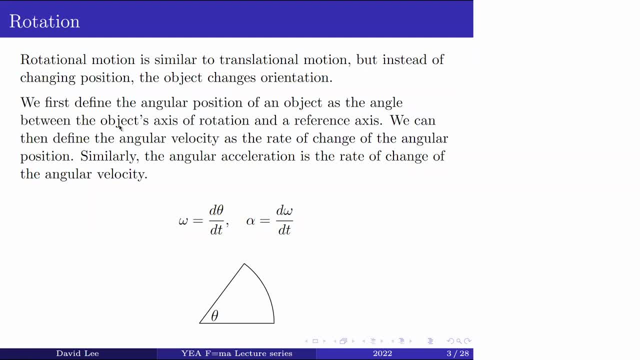 So rotational motion is similar to translational motion, but instead of changing your position coordinate, you're changing an angular coordinate. So in translational motion you might have like go from point A to point B. This is a distance of x. 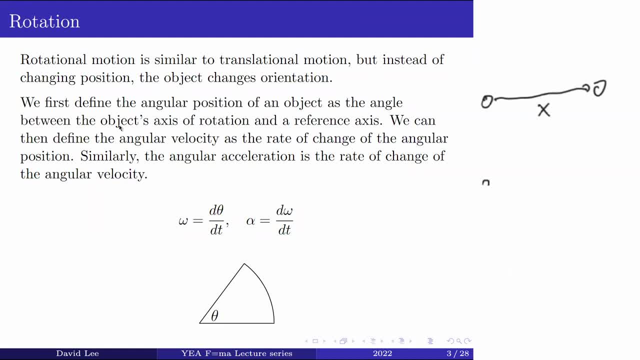 In rotational motion, like, instead of moving, you will rotate. So this would be, say, a rotation of 90 degrees, and or this would be pi over two radians. So how many radians that you moved? This is your angular distance. 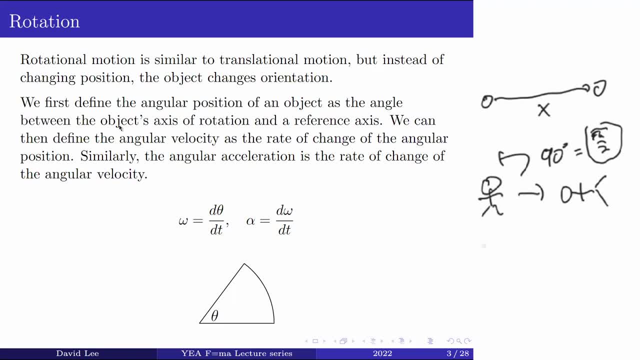 So we can also define an angular velocity, which is the radius of your rate of change of your angular distance, and an angular acceleration, which is the rate of change of your angular velocity. And this is just similar to normal velocity and normal acceleration. It's. 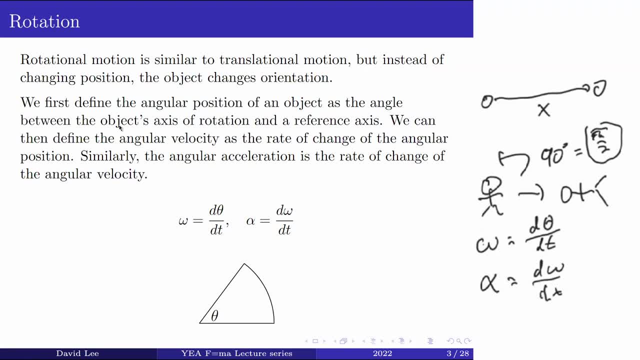 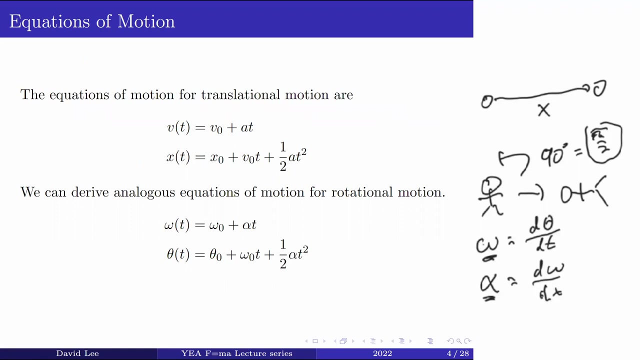 just for angles instead of position, And the symbols we commonly use for these are omega for angular velocity and alpha is for angular acceleration. All right, So we have some equations of motion for translational motion, And if you remember them, they are these equations: 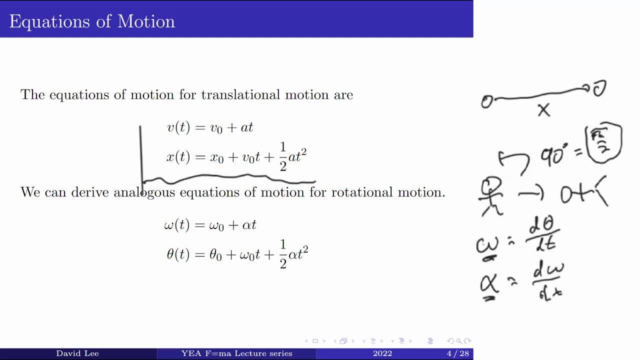 right here, And and. So, since the velocity and acceleration were similarly defined, v equals dx dt and a equals dv dt, if you look at these two equations, they're basically the same as these two equations. So if we go through the exact same steps, you'll get these two equations. 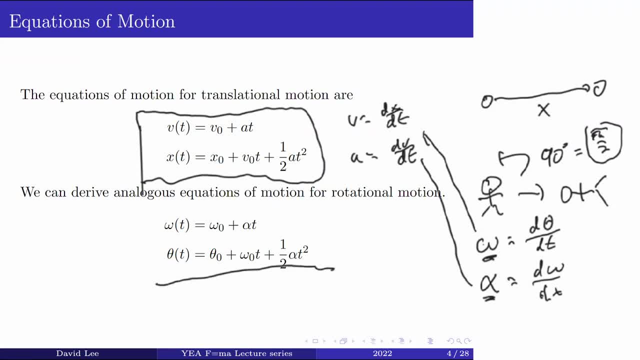 So, since the velocity and acceleration were similarly defined, v equals dx dt and a equals dv dt. if you look at these two equations, which are basically the same, but you can use them for constant angular acceleration instead of the previous, these two were for constant translational acceleration. 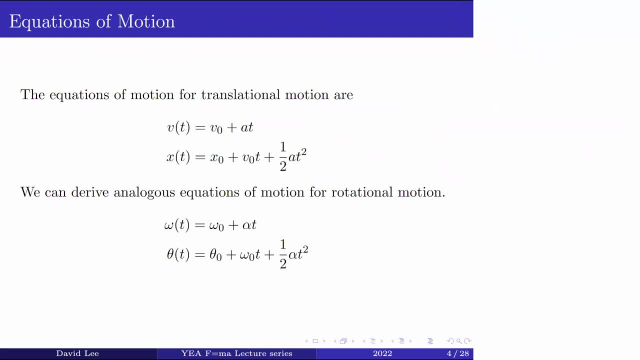 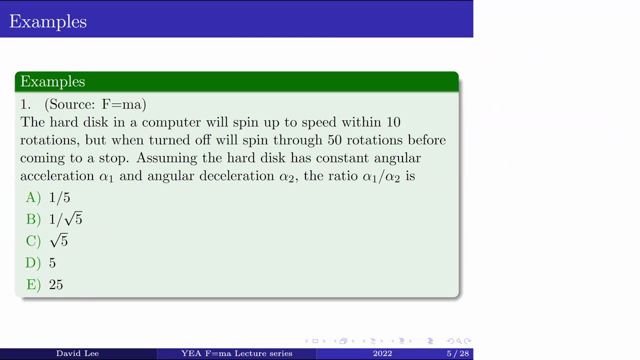 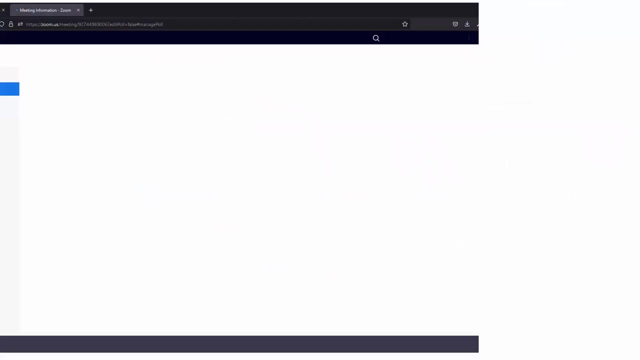 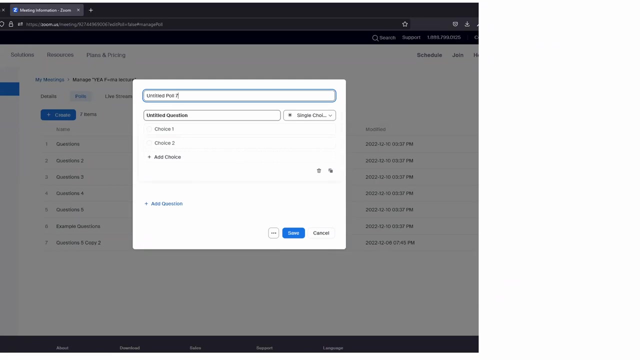 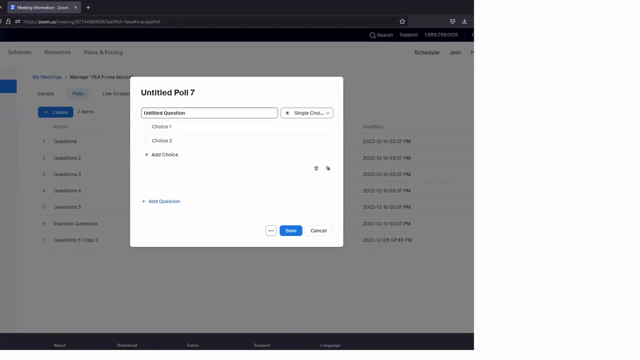 All right, Now let's try an example. So I will, as usual, I will start my poll. Oh no, Um, hold on. Yeah, so I'll give you a few minutes to work on this And shoot. 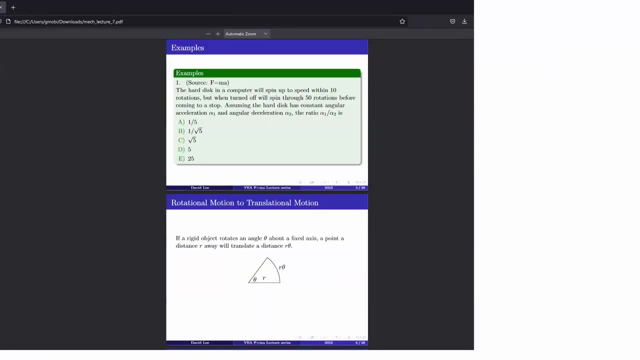 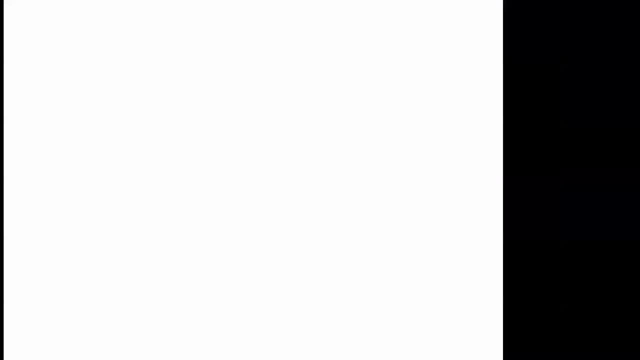 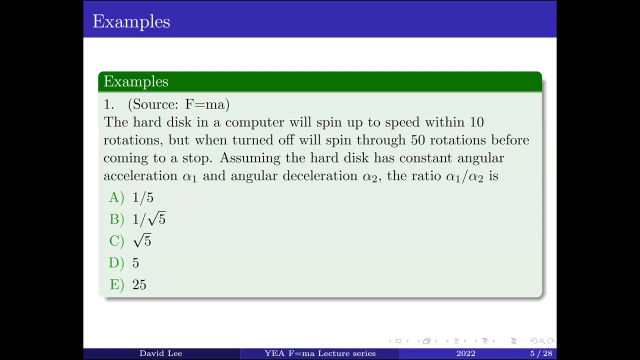 Oops, I will try to fix this. All right, we're back, So I'll give you a few minutes to work on this question And feel free to ask any questions or send me your answers. I will give you a few minutes to work on this. 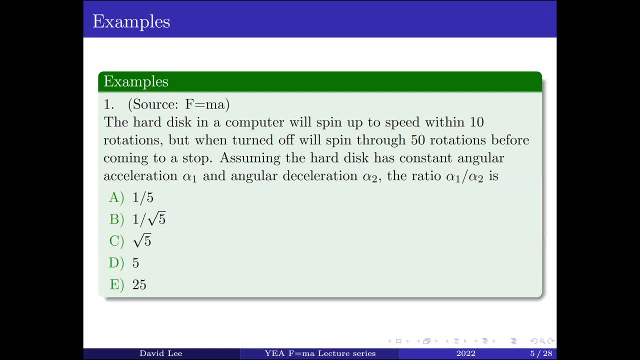 And shoot. Oh no, All right. So I'll give you a few minutes to work on this And feel free to ask any questions or send me your answers. And feel free to ask any questions or send me your answers. And feel free to ask any questions or send me your answers. 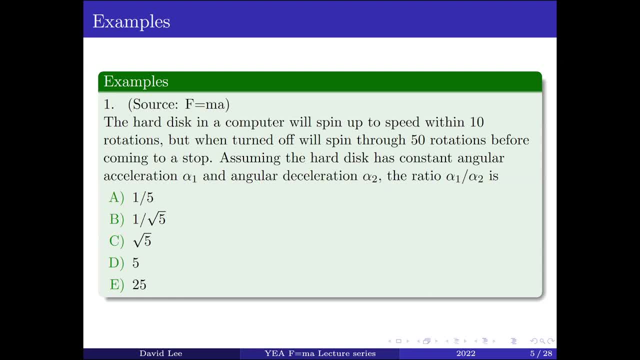 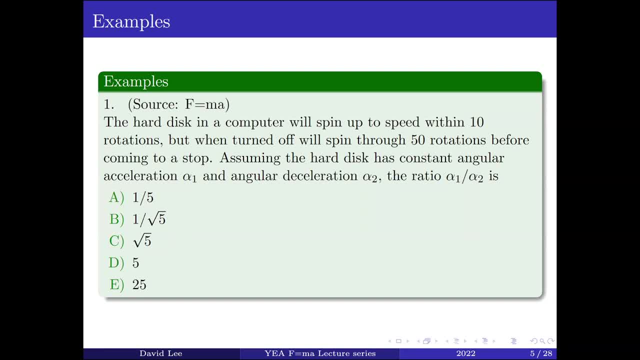 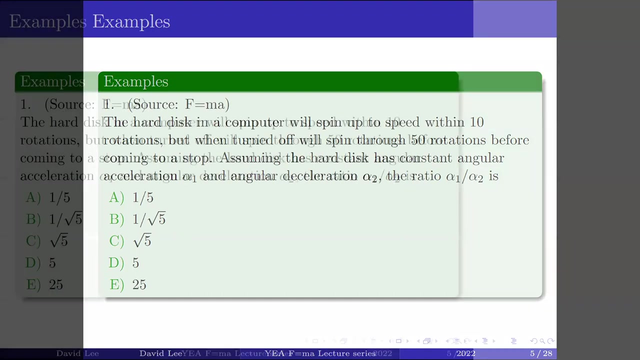 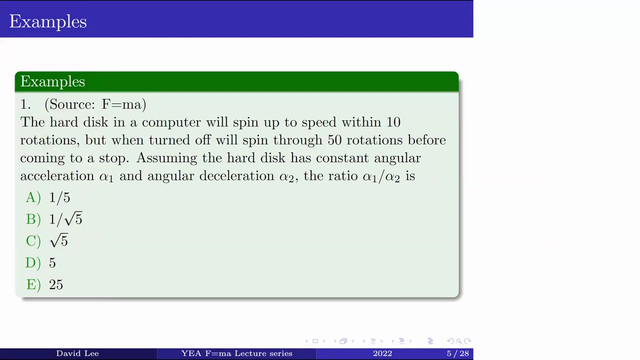 So I think the correct answer here should be D or let's take a look. First of all, let's look at what's going on. So we have a computer disk which is spinning, and I'm assuming it will accelerate at a constant. 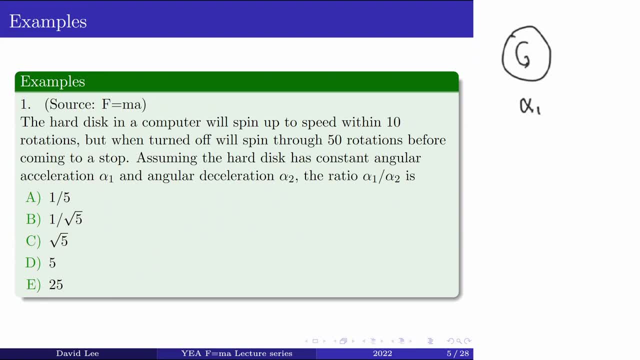 acceleration alpha one until it gets up to speed, And after that I guess it will just continue spinning at a constant angular velocity of omega And then after that, after it's done spinning, it will slow down at angular acceleration alpha two And this makes the angular velocity go from omega to zero. 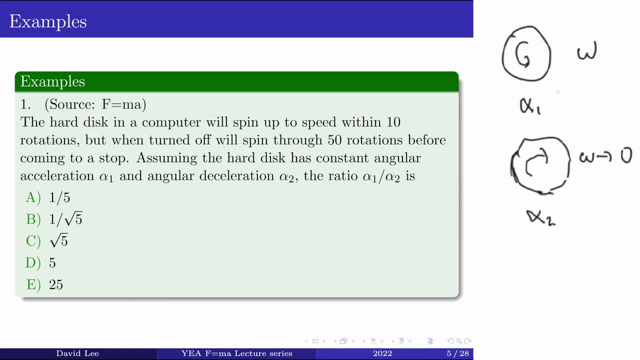 So what do we know? Well, we know that as it's accelerating, It will spin up to speed in 10 rotations, And when it's decelerating, it will spin down to a stop in 50 rotations. Okay, that's very cool. 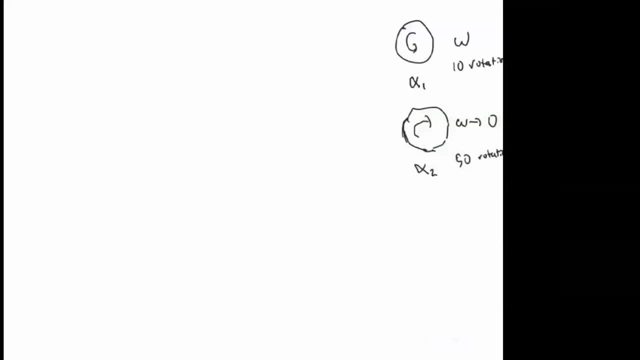 So let's look closer at this problem. Okay, So let's look closer at this problem now. So how will we solve this problem? Well, we can use our kinematic formulas, And before I mentioned that we can have used the same equations. data equals one half alpha. 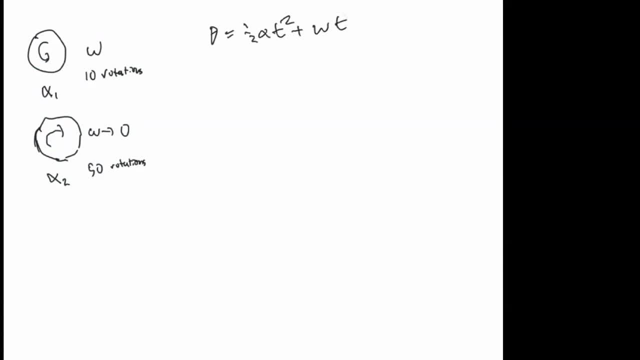 T squared plus omega T. Okay, And omega is omega 0 plus alpha t, And we have like the same equations as in the translational case, like this one corresponds to delta: x is half a t squared plus vt. And this one corresponds to delta: v is just a t, right? 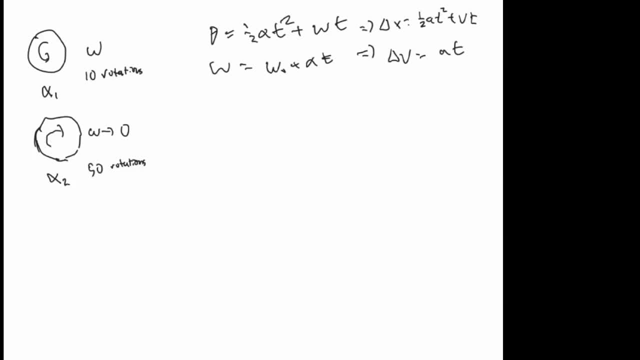 But turns out we can actually use the other kinematic equations that we derived from these two. So like: what's one v squared v final squared equals v, initial squared plus 2a times delta x. We derive this from these two right. 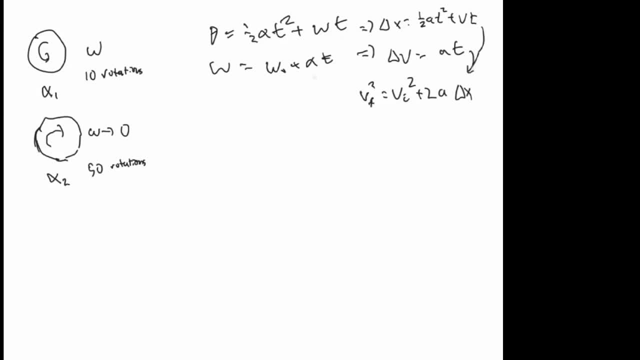 So if we follow the same steps we can get the same equations: Omega final squared equals omega initial squared plus 2 alpha times theta. And in general, if you have a kinematic equation that works with x and v and t and a and stuff like that, 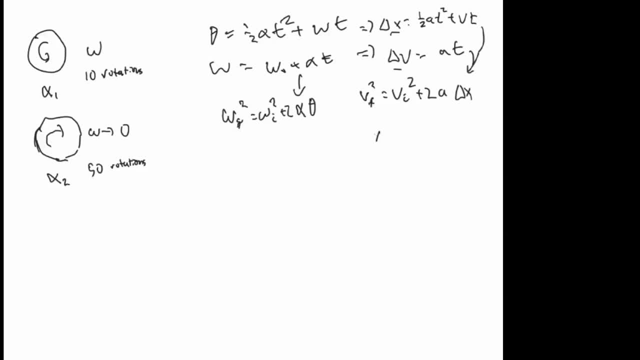 you can probably just replace x with theta, replace v with omega and replace a with alpha, And you'll get the corresponding equation in rotational motion. All right, so back to the question. I think this equation will be the most useful here, because we know: 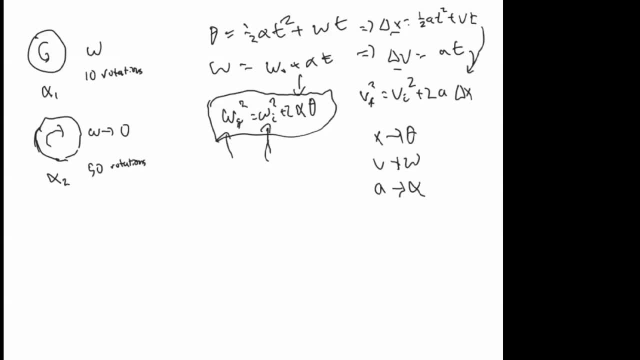 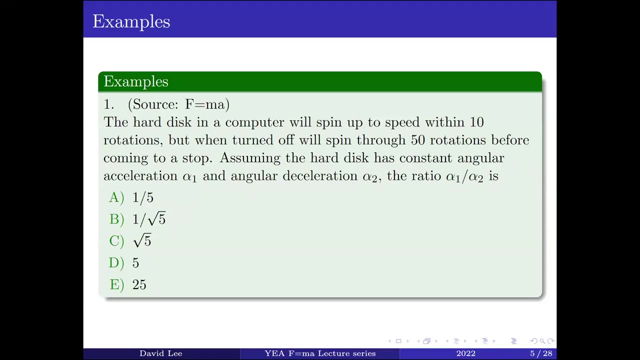 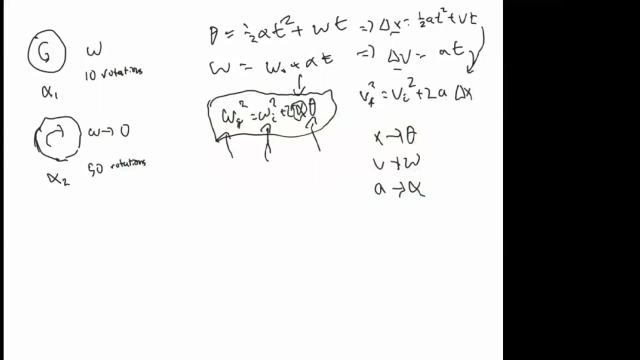 we know what omega final is, we know what omega initial is and we know what theta is. And if we go back to the problem, the problem's just asking us what is the ratio, alpha one over alpha two? So we want to find the alphas and we can do that, because alpha is the only unknown in this equation. 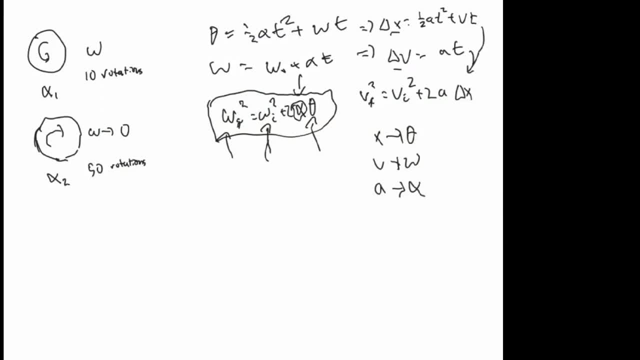 All right, so let's write down this equation. So, first of all, for the accelerating phase, what do we get? So omega final here is just omega, and omega initial is zero And it has angular acceleration, alpha one, and it goes through ten rotations. 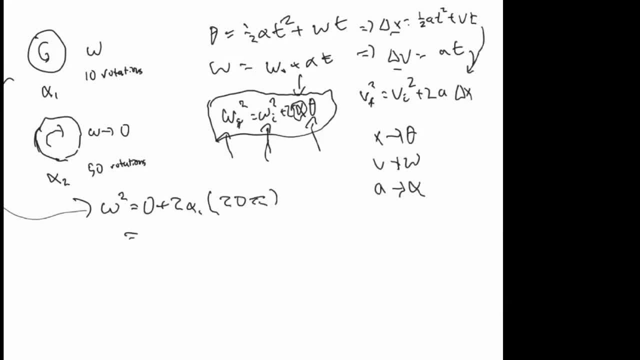 which is 20 pi. All right, so we get that alpha one is omega squared over 40 pi. Very nice. Now what about alpha two? Well, if we write down the equation- but now we're decelerating- well, its final omega is zero. 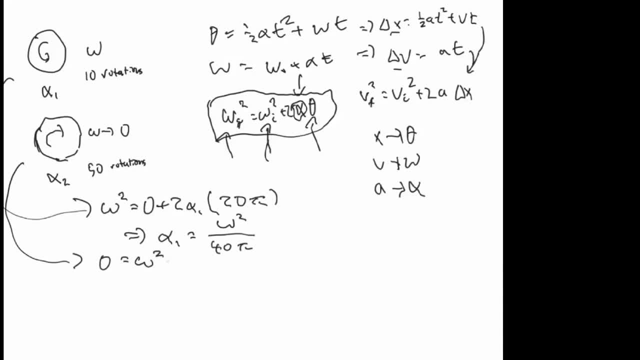 Its initial omega is just omega, And then its accelerating at minus alpha two And 50 rotations, so 100 pi, All right, And then we get that alpha two is equal to omega squared over 100 pi. So now we have the information we need to solve the problem. 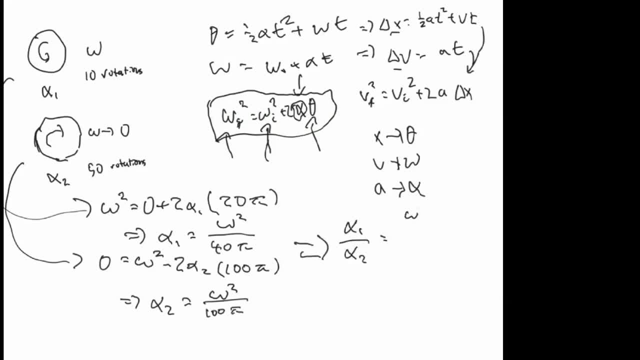 We get the alpha one over alpha two, Omega squared over 40 pi And Omega squared over 100 pi. Sorry, 200 here, And we get that. the answer is five. Alright, cool, Any questions, or I will just move on. Okay, then. 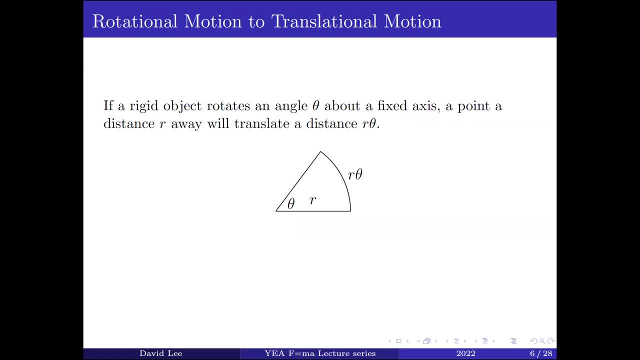 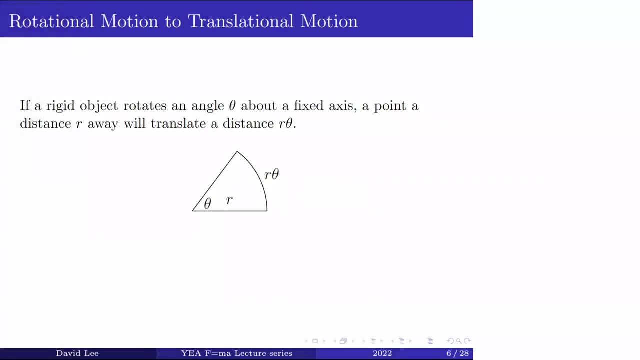 So let's talk a bit about it's this rotational motion to translational motion. so if a rigid object rotates an angle theta, a point or away from it will translate our theta. this is like, I guess, how circles work. so What this means is basically just: 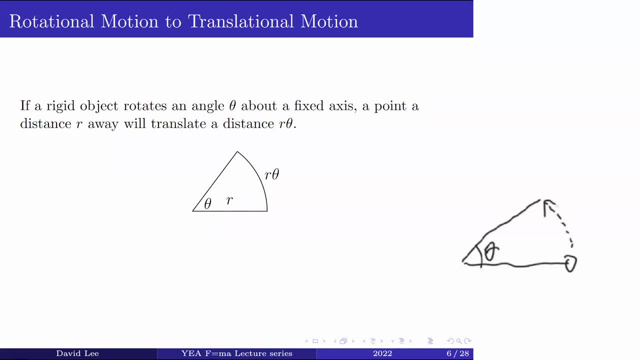 An object that moves this way, If this is our, and this is data, than this distance will be our theta. and note notice that theta here has to be in radians, otherwise this won't work, so always use radians. And so, basically, if we write a distance as as our theta, 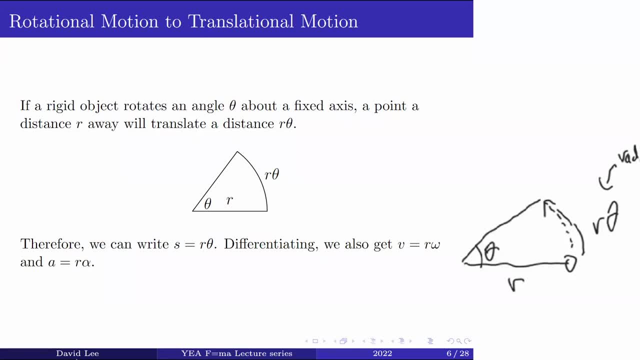 We can get that V equals our Omega and a is our Alpha. so I guess if we have something moving in a circle, We can write V equals our Omega, because if this angle is changing at a rate Omega, than this distance will also be changing at a rate or Omega. 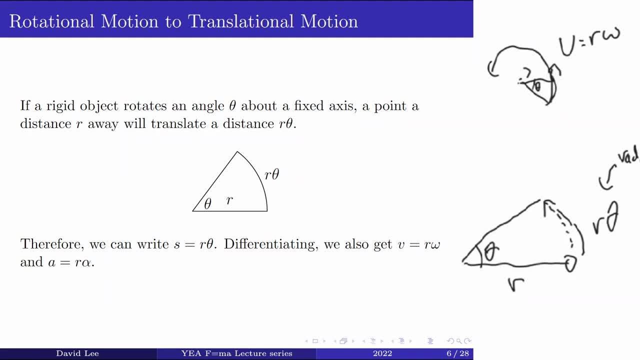 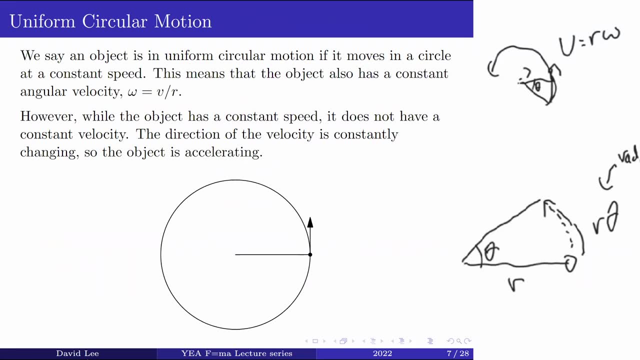 So this will be its velocity, and similarly for acceleration. All right, Now let's talk about uniform circular motion. So this is a special case of circular motion. I guess it's just an object moving in a circle with a constant speed, it's just. 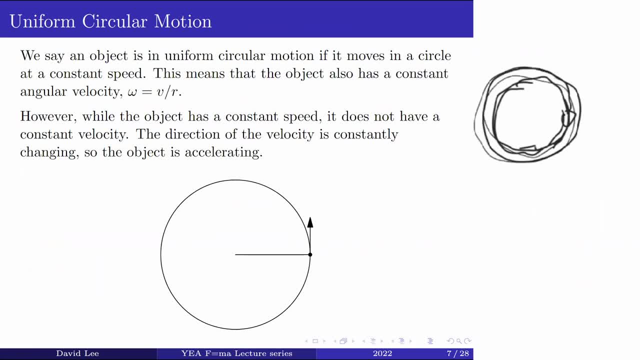 Moving around and around like that. However, it velocity is actually changing here, because if we look right here, it's velocity points that way, but a little while later it points that way and Correction is direction continually changes. Which is All the dumb dumb. 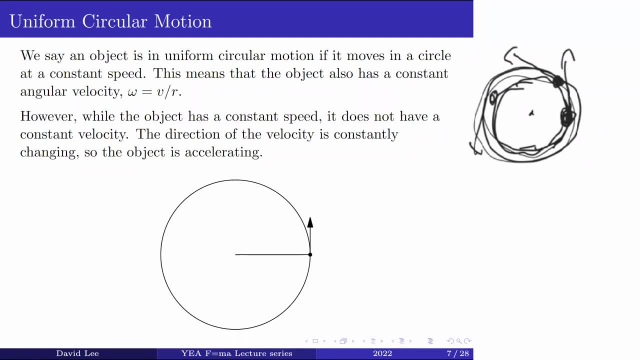 I'm sorry. do you have a question? I guess not, Because let's continue focus on what. i'm sorry, I couldn't really hear you Clearly. do you have a question? Okay, nevermind, let's continue. So yeah, the velocity, the direction of the velocity is changing, even though 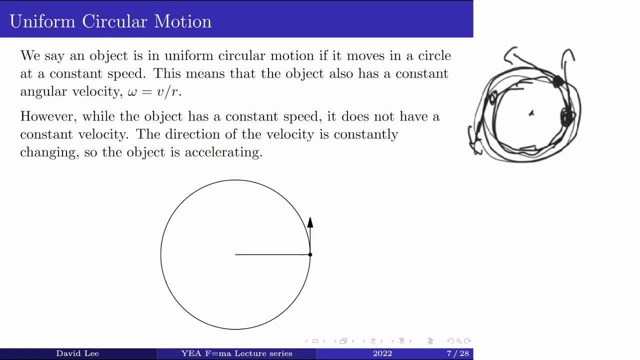 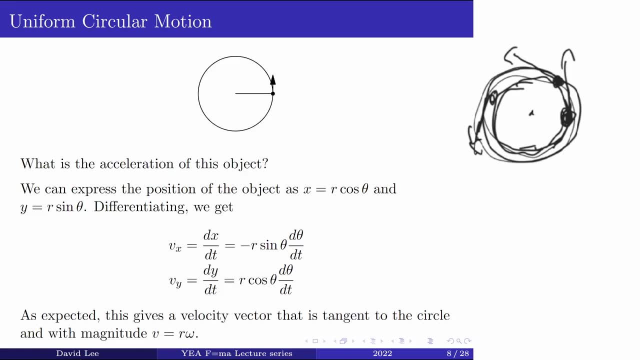 The magnitude is not, and so this means that we have to have an acceleration. Well, what is this acceleration? Well, All we have to do to find it is, Say: express Its position as a function of theta, and theta is a function of time. so we'll get its position as a function of time. 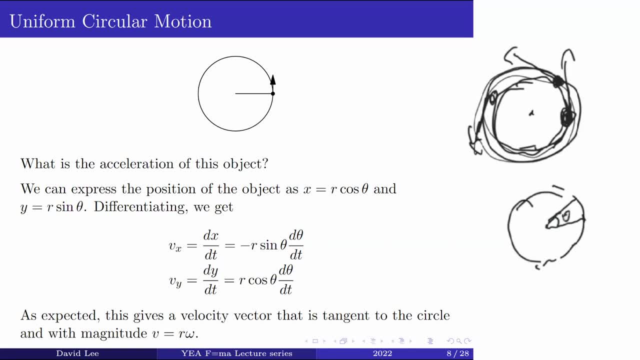 So say this is like our theta, Then it's X position. here Is our cosine theta and it's why position here, Our assigned theater. So now we'll get its wide velocity by differentiating and notice that data is a function of time here. so we also have to use the chain rule to 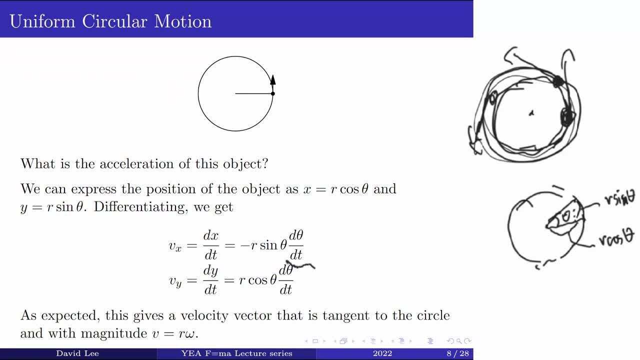 Add a term: D theta DT, And similarly, we'll get our wide velocity and X velocity listed here. So, like we said before, Okay, so this is Negative. our sine theta times Omega And this is our cosine theta Times Omega. 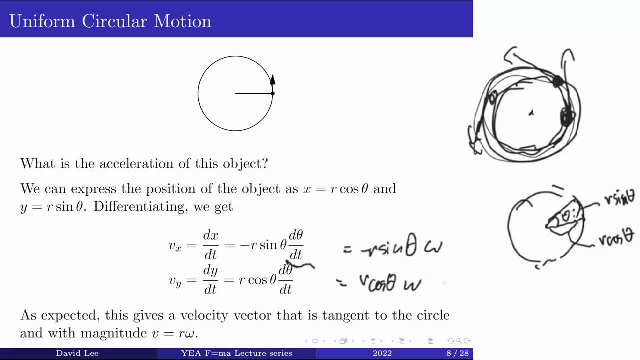 So then, What? what is this velocity? well, if you draw it out, all it's doing is it's tangent to the circle, as we expected, And its magnitude Is the square root of negative: our sine theta- Omega squared, Plus our cosine theta- Omega squared. 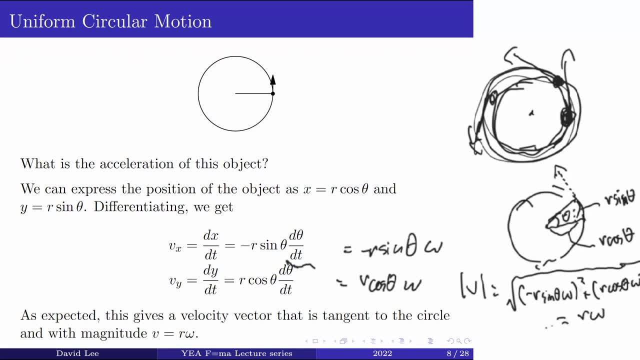 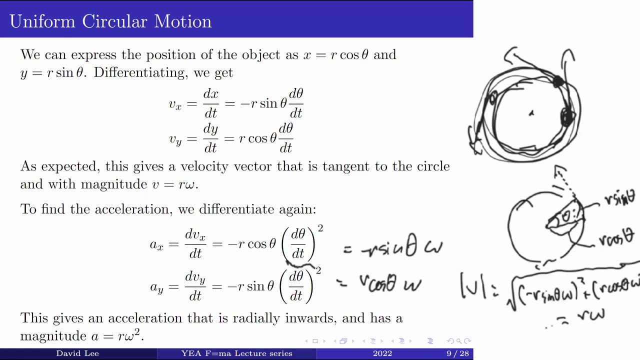 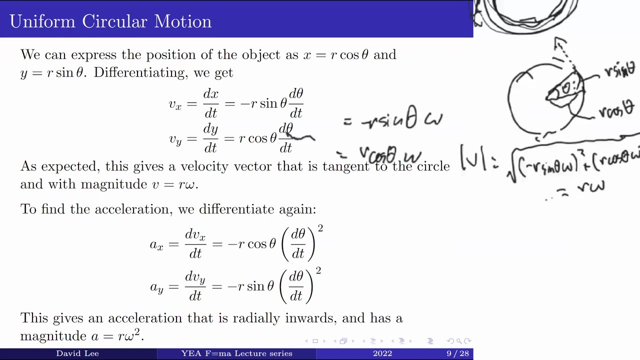 And this is just our Omega, like we expected. Okay, now we have its velocity and we can just differentiate again to get its acceleration. So Those were our formulas for the velocity. Now, if we differentiate again, We will get this, these Formulas for acceleration. 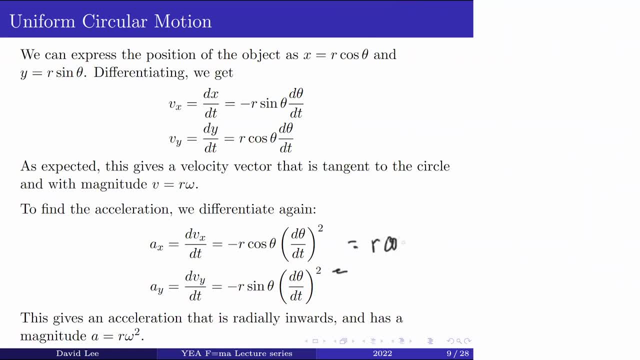 So this is our cosine, theta Omega squared, And this is negative, our sine theta Omega squared. All right, what does this mean? Well, If we try in our acceleration here, We'll find that it's in this direction And its magnitude. 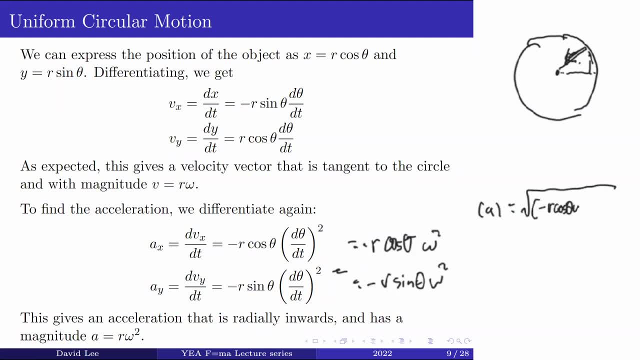 Is the square root. negative, our cosine theta Omega squared squared, Plus negative, our sine theta Omega squared squared. And this is our Omega squared. So what this tells us Is that If an object's moving in a circle with radius R And angular velocity Omega, 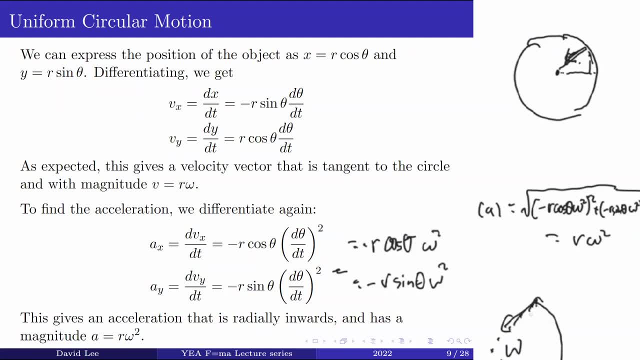 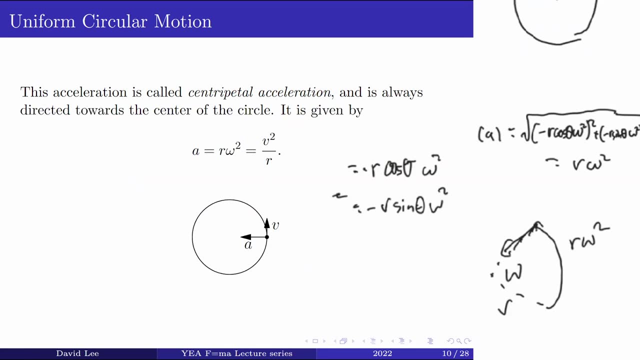 Then it has to be accelerating radially inwards, With the magnitude of the acceleration being our Omega squared. All right, And this is very important, This is called the centripetal acceleration And, As I mentioned earlier, It's always towards the center of the circle. 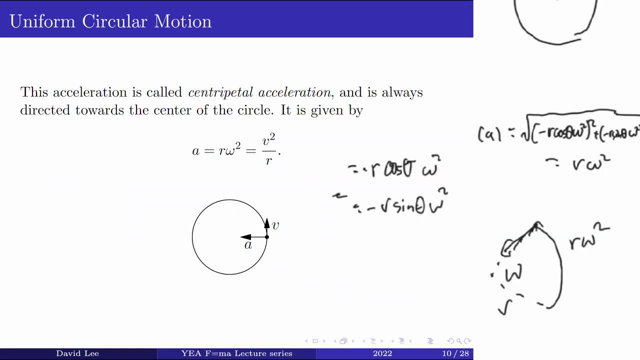 So any object That is traveling in uniform circular motion Must have this acceleration Pointed towards the center of the circle, And We can write it as equals R, Omega squared, Or if we substitute in Omega, Omega here equals B over R. 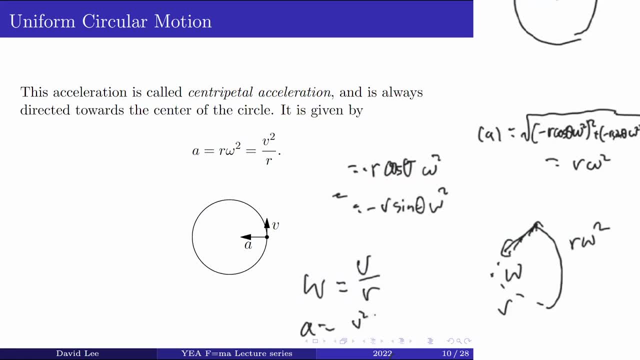 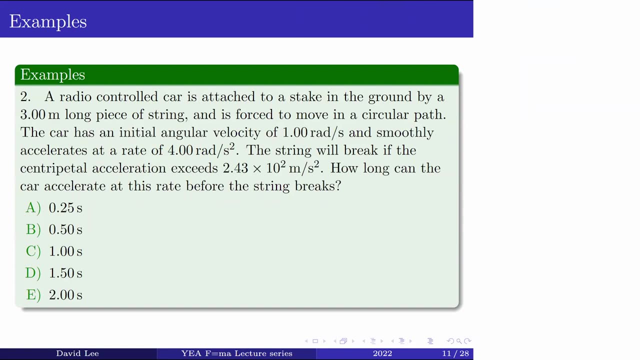 We'll get that. A is also V squared over R. All right, Now let's do an example. So I will also give you a few more minutes And feel free to Ask Questions Or Send me your results, Okay. 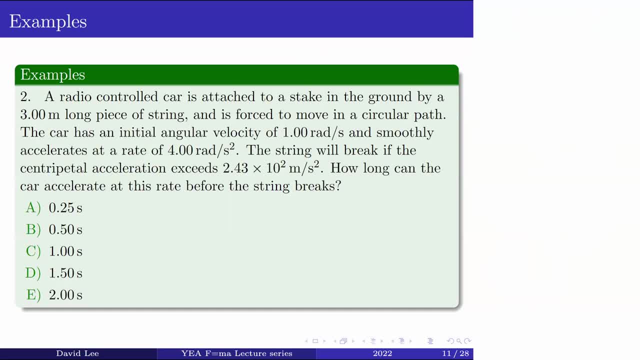 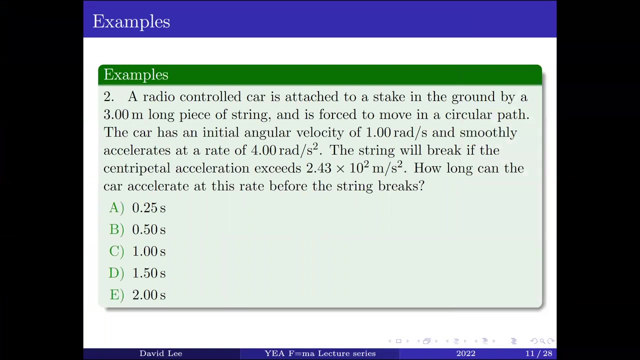 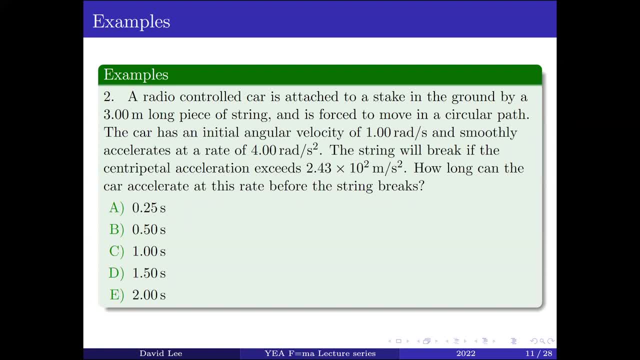 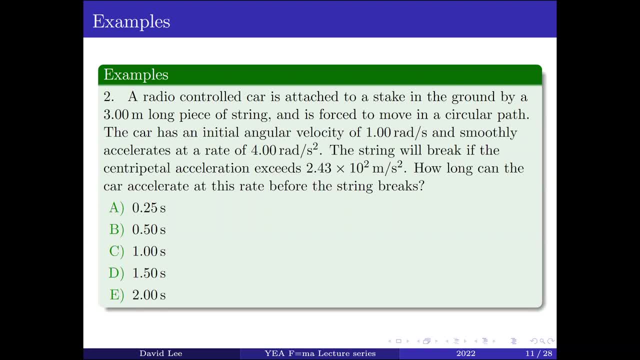 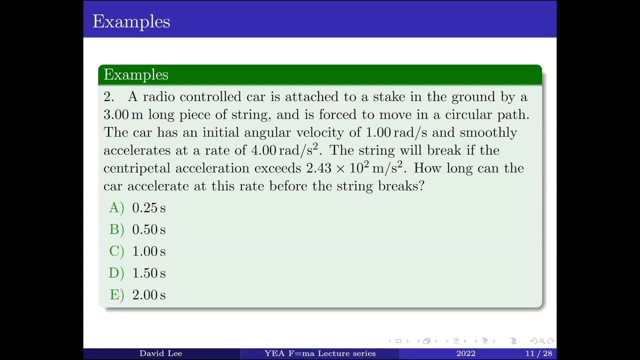 so one person chose b, a lot of people chose e and also one person chose f. and just a quick contest tip: you should never choose f because it's um, basically never the answer. so, yeah, in this case, f was not the answer, the answer was e. so it's good that a lot of people chose that. 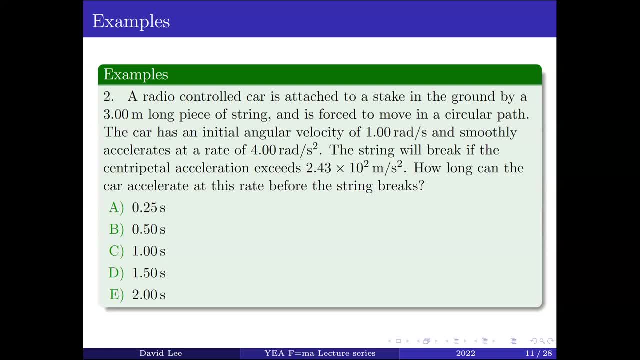 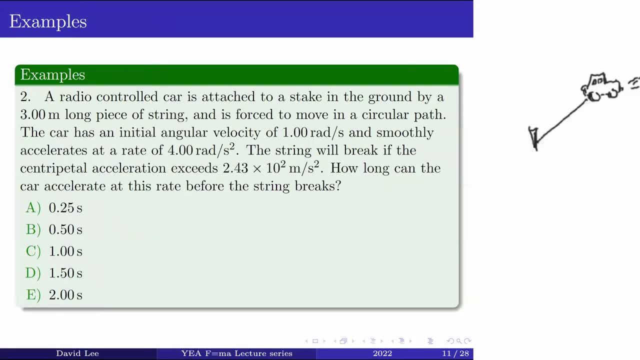 um, so let's talk about this question. so we have a car here and it's attached by a stake in the ground, so it's forced to move in a circular path and the radius of this path is three meters. so it's moving in a circle and initially its angular velocity is one radian per second. 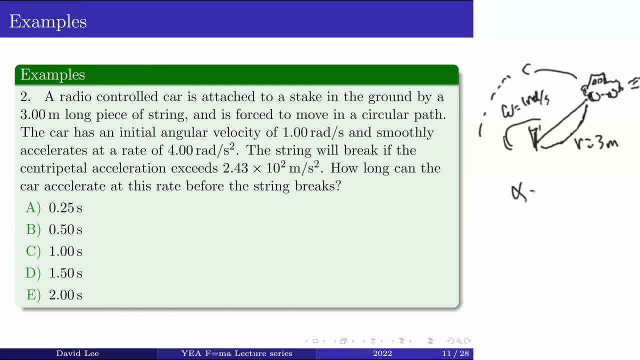 and it has an angular acceleration alpha of four radians per second squared, all right. and the question says the string will break if the centripetal acceleration a becomes too high, and specifically a greater than 243 radian or meters per second squared. all right, so how do we solve this question? 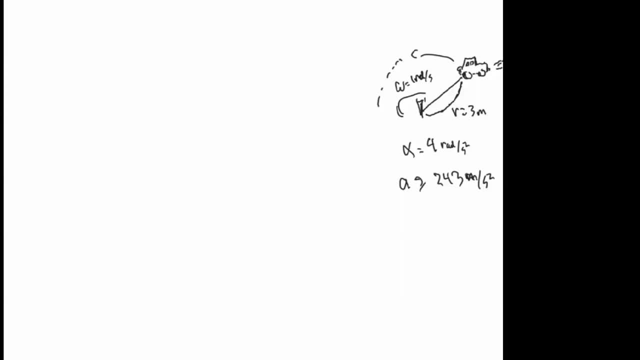 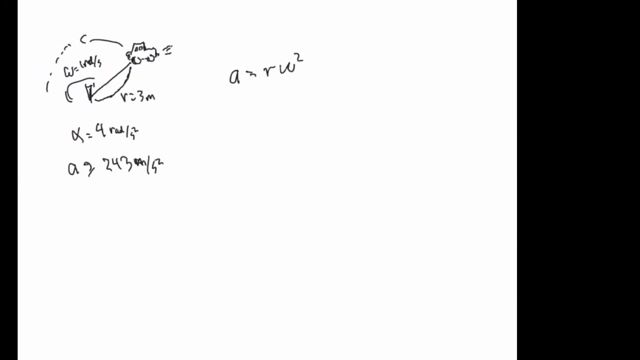 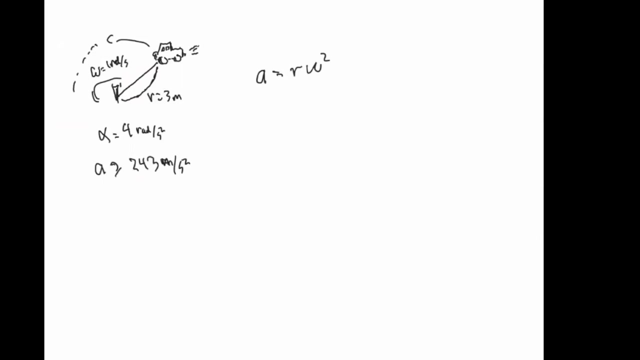 well, it's actually pretty simple. so if we go back to our formula for a centripetal acceleration, the acceleration is r, omega, squared right. so so the key is to realize here: well, when will the string break? well, the string will break when omega reaches square root, a over r. 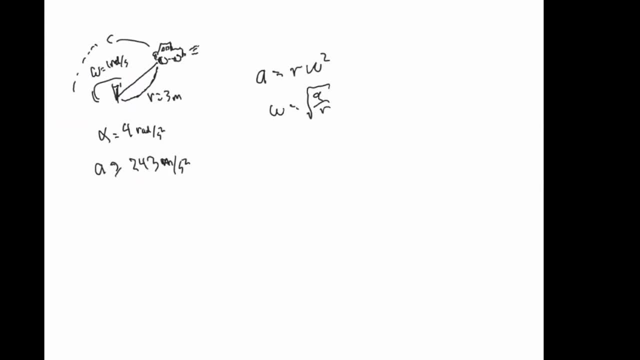 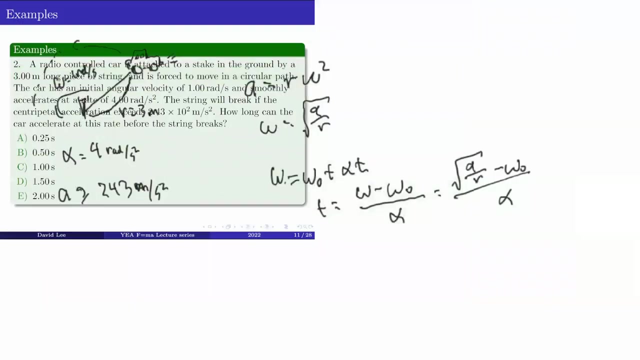 and when will omega reach this point? well, we have the kinematic equation: omega is omega zero plus alpha t and omega is on the singer, so our t will be omega minus omega zero over alpha, or we can substitute in this. and so now, if we go back to our problem, 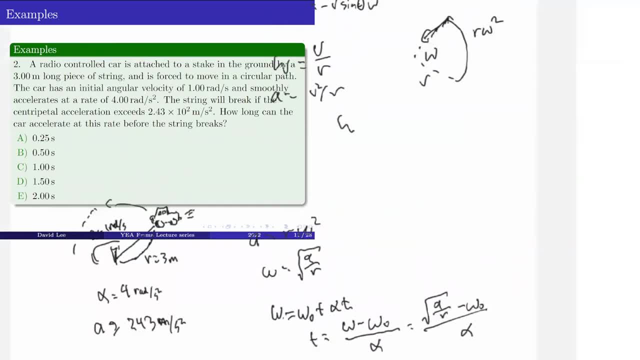 oop, let's do this. so now, if we go back to our problem, I wouldn't be – if you don't repeat it, start over, we're not going to get into it. you know, we know what A is, we know what R is, we know what omega 0 is and we know what alpha is. 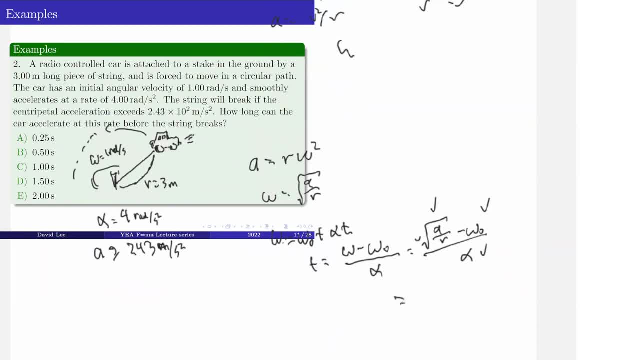 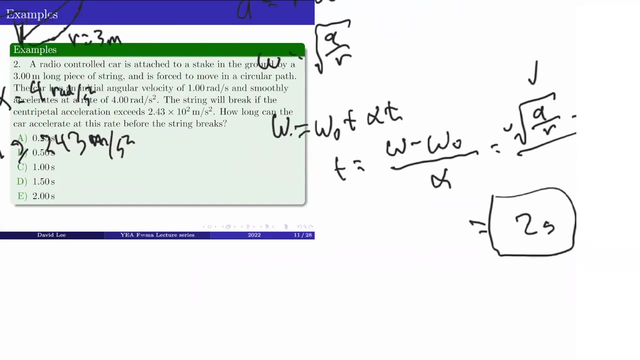 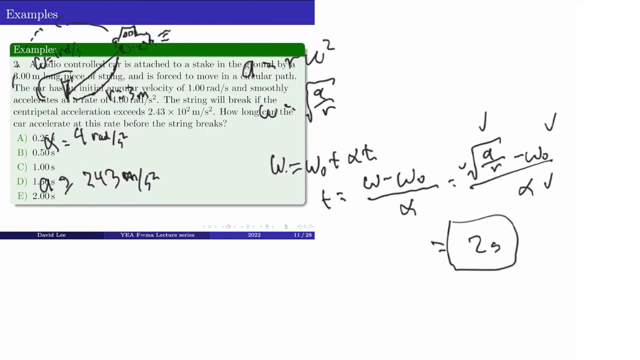 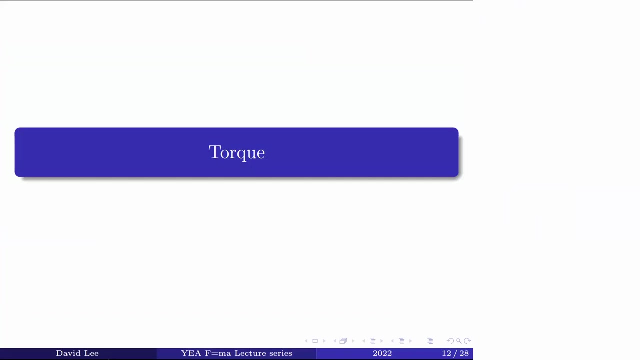 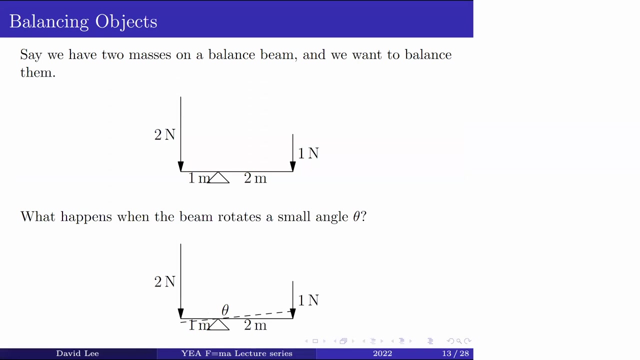 So now we can just plug all of these in and this will give a time of two seconds. All right, cool. Do you have questions or no? All right, so let's move on, And now we can talk about torque. So what is torque? 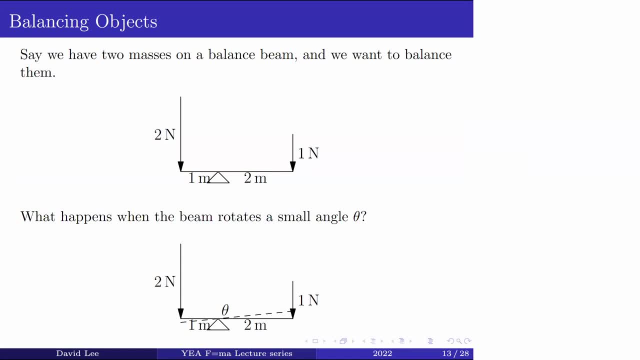 Well, let's think about torque. Let's think about torque, Let's think about balancing objects. here for a second. The idea behind torque is: if you have two forces that act at uneven distances on a rigid body like this, well, what will happen if the beam rotates a small angle? theta. 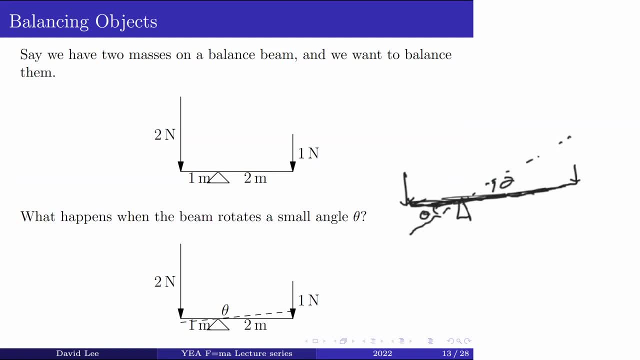 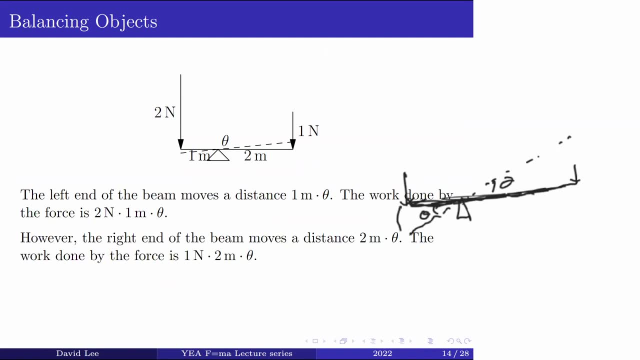 Well, what would happen is that this end of the beam moves the distance of, say. in my example it was one meters and two meters, So this end of the beam would move one theta, but this end of the beam will move two theta. 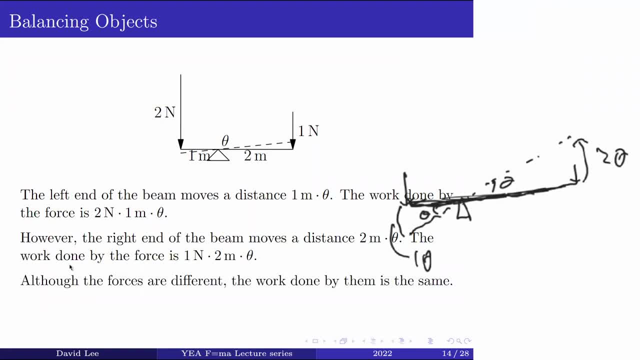 All right, But what does this mean? Well, in my example we also had a force of two newtons here and one newton here. Well, this force does two newtons times one meter times theta, or two joules times theta- amount of work. 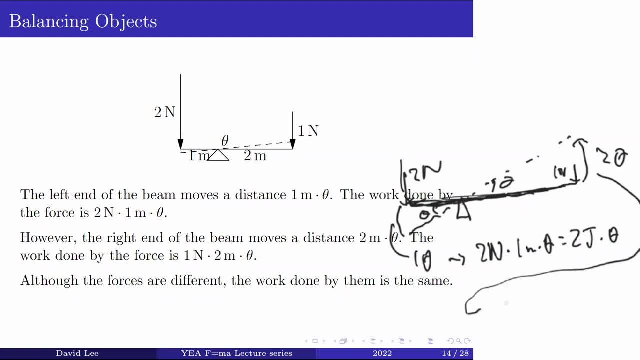 All right, And this force also does well. it does one newton times two meters times theta. also two joules times theta amount of work. Okay, so we see that these two forces, although they're different in magnitude because of how far away they act from the pivot, 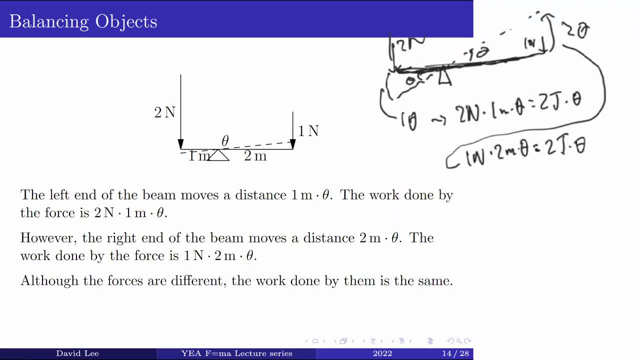 okay, so we see that these two forces, although they're different in magnitude because of how far away they act from the pivot, they will do the same work while our object rotates an angle of theta. they will do the same work while our object rotates an angle of theta. 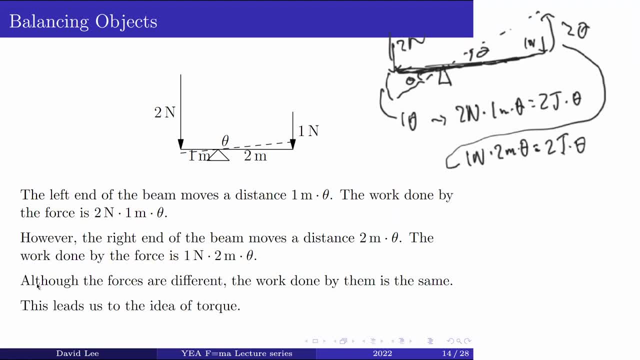 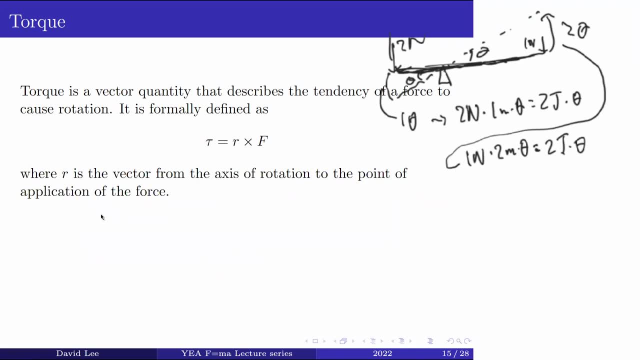 So this motivates our idea of torque, which is basically, if we multiply our force by the radius at which it's acting, we get- well, we'll get how much work per angle does. So this motivates our idea of torque, which is basically, if we multiply our force by the radius at which it's acting, we get, well, we'll get how much work per angle does. So this motivates our idea of torque, which is basically, if we multiply our force by the radius at which it's acting, we get- well, we'll get how much work per angle does. So this motivates our idea of torque, which is basically, if we multiply our force by the radius at which it's acting, we get, well, we'll get how much work per angle does. 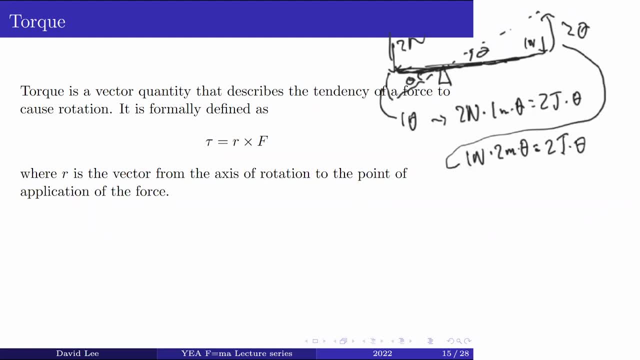 So this motivates our idea of torque, which is basically, if we multiply our force by the radius at which it's acting, we get how much work per angle does. So this motivates our idea of torque, which is basically, if we multiply our force by the radius at which it's acting, we get how much work per angle does. 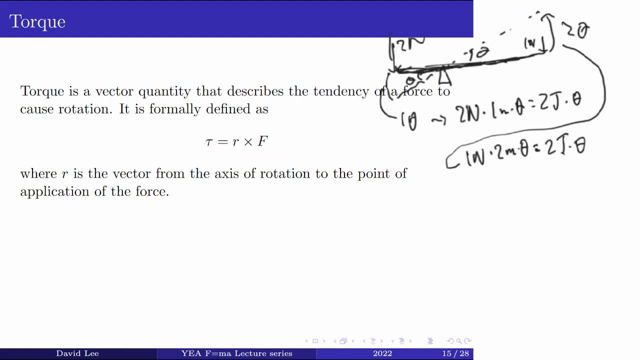 So this motivates our idea of torque, which is basically, if we multiply our force by the radius at which it's acting, we get how much work per angle does. So this motivates our idea of torque, which is basically, if we multiply our force by the radius at which it's acting, we get how much work per angle does. 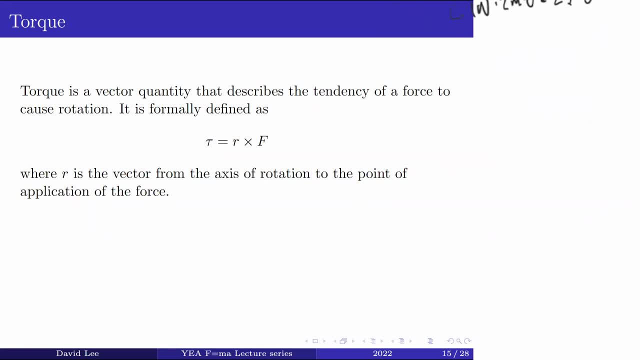 So this motivates our idea of torque, which is basically, if we multiply our force by the radius at which it's acting, we get how much work per angle does. So this motivates our idea of torque, which is basically, if we multiply our force by the radius at which it's acting, we get how much work per angle does. 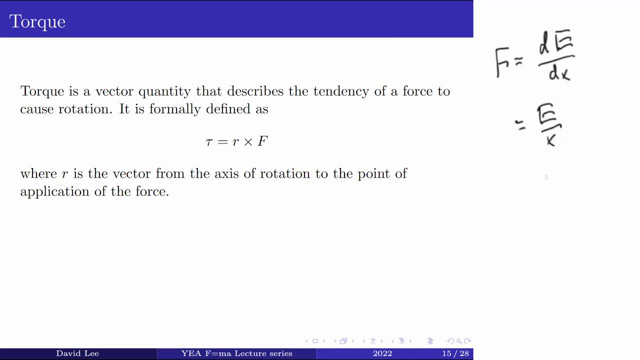 Well, we see now that x is r theta, right, So this is e over r theta. So if we simplify this, f times, r is e over theta. So what we call this now is a torque tau, And tau is the symbol normally used for torque. 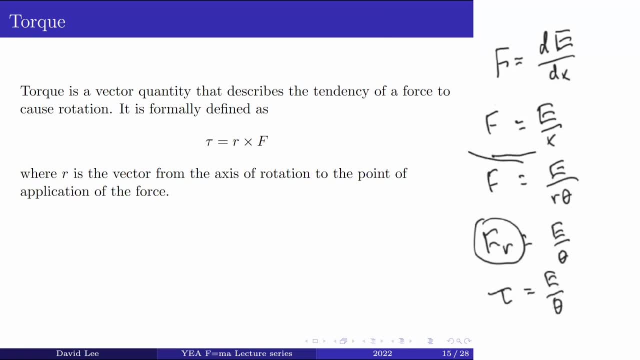 Tau is e over theta, So these two equations are translational and rotational analogs of one another. So we can think of torque as really just a rotational force. And if we want to define torque more generally, what we get is it's actually the cross product. 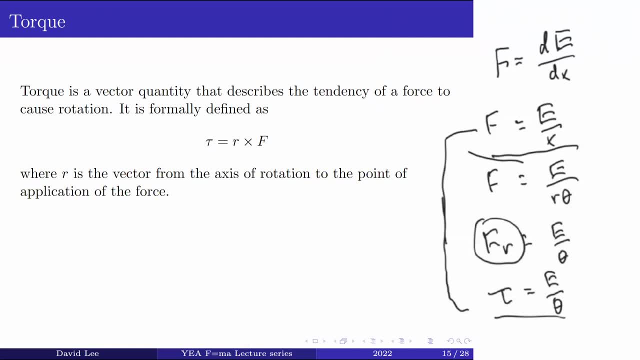 of r, theta, R, radius and the force. So if we have a pivot here and we have a radius r and then we have a force that's not entirely perpendicular, Well the torque will be f times r times sine theta. So we can think of this as the either theta being 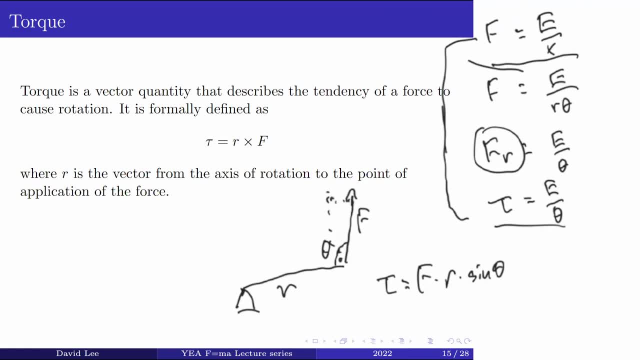 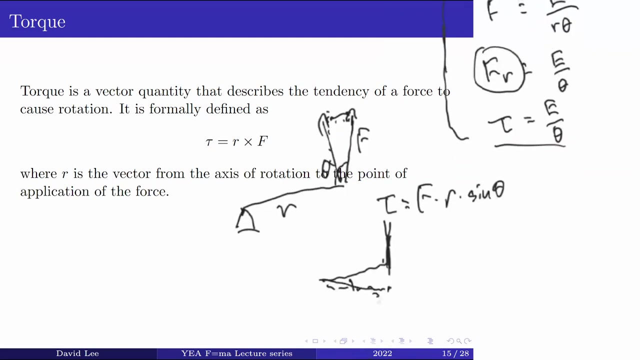 sine theta being the component of the force. that's in the right direction to apply torque. Or we can also think of r? sine theta as the lever arm, So how much leverage we're actually getting from our radius? But anyways, there's a torque as a cross product. 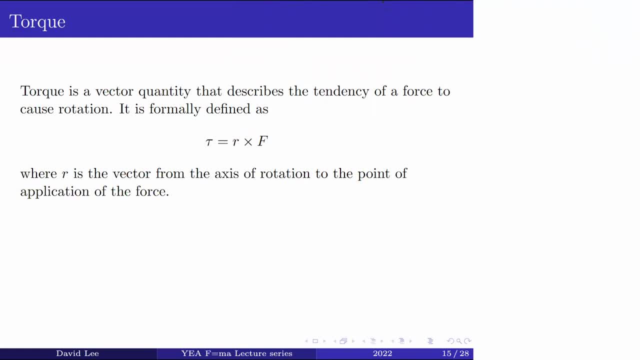 It is a vector, but normally we'll just be thinking about either clockwise or counterclockwise torque, So normally we won't have to worry about the direction of torque in simpler problems like this. So yeah, torque is the equivalent of angular force. I think we motivated that with energy. 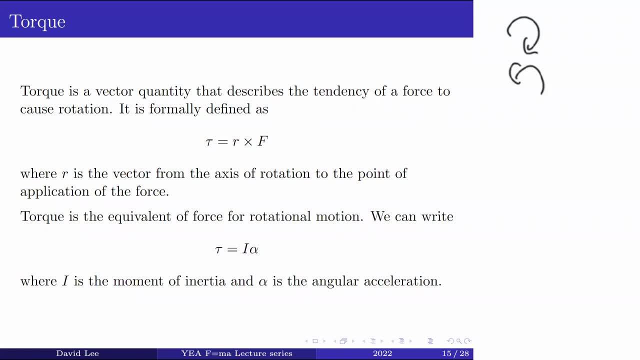 but now we had force equals ma right. So now we should be able to define some equivalent for angular motion. Well, we have our angular force, which is torque, and we have our angular acceleration alpha. Now we're just missing. what is our mass? 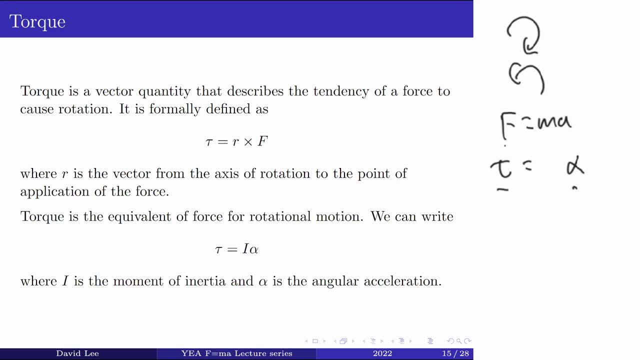 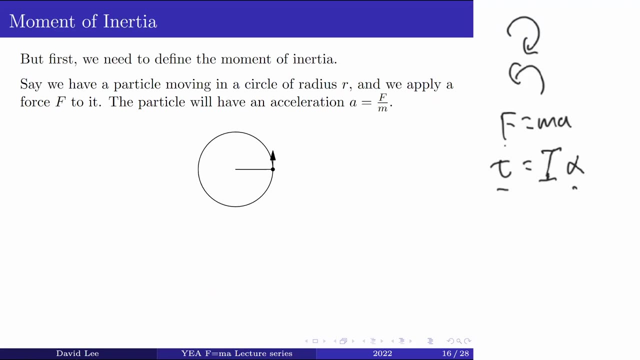 right? well, it turns out we can't just use mass here. We have to use something known as the moment of inertia, And I will talk about that next. So say, we have a particle moving in a circle, as usual, and we're applying a force. Okay, just one particle here And we apply a force. 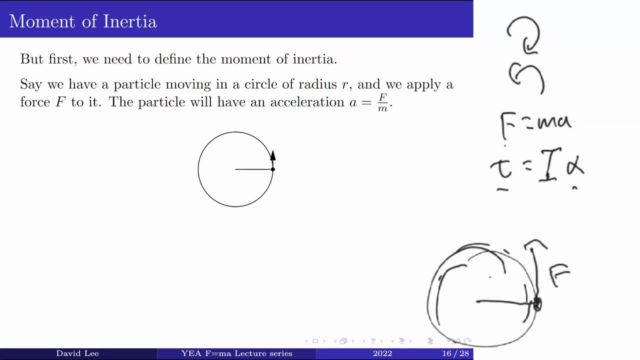 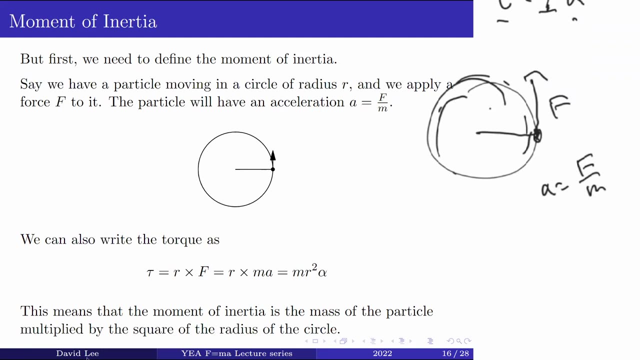 And by Newton's second law. okay, our acceleration is force over mass. Okay, that's very cool, But what about our acceleration, Our angular acceleration, And what about our torque? So the torque is F times R And the angular acceleration is. well, we know that R alpha equals A. So the angular acceleration, 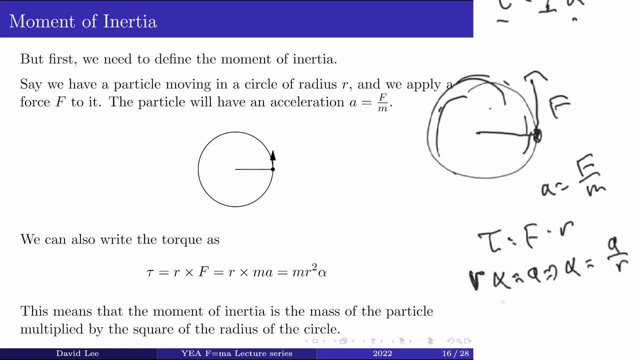 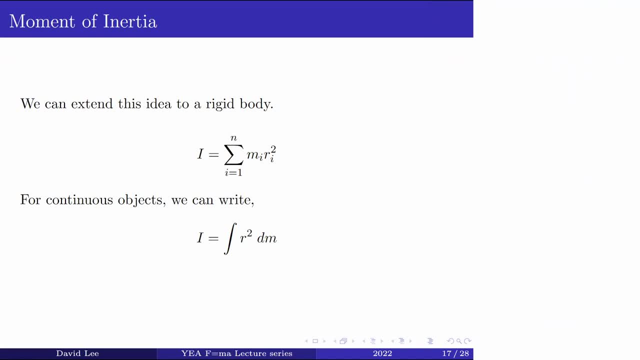 And then we get that R over R, And then we get that R over R. And something important to point out is that these are all of the rotational quantities are relative to a certain axis, So let's say we're like spinning around this axis. 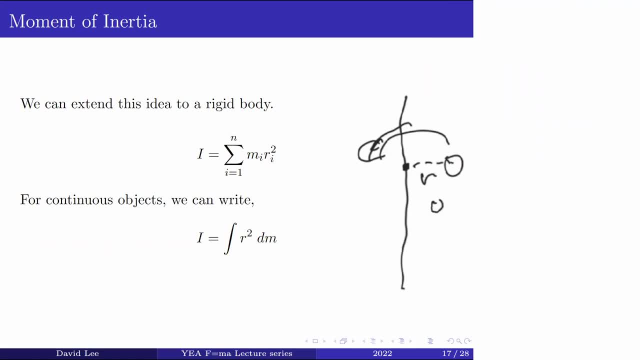 Well, this will be our R. Let's say we have a triangle of points, How about that? And these are our R? And these are just point masses connected by massless rods. So our total moment of inertia is M1- R1 squared plus M2- R2 squared plus M3- R3 squared. 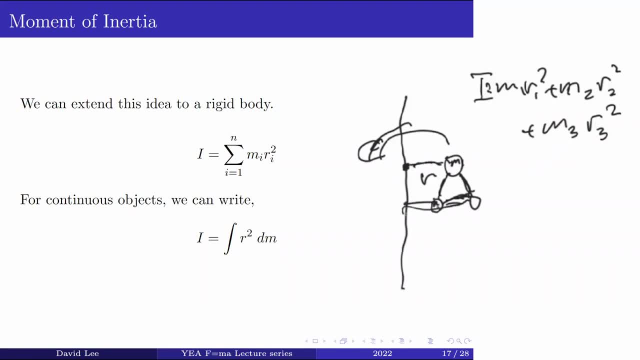 Those are our three masses, These are our three radii And this is our axis. Well, actually this is just an example- This can change Like if our axis becomes here and now we're rotating around that axis, well, all of our radii will increase. 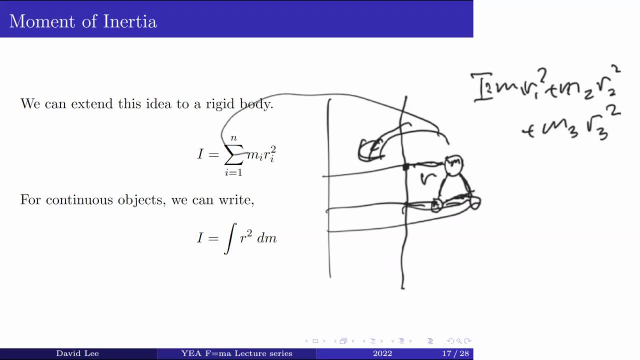 So it's always important to pay attention to what axis of rotation you're talking about when you're doing these problems. And there is also the continuous case of our equation, which is that I is equal to R. I is the integral of R squared DM. 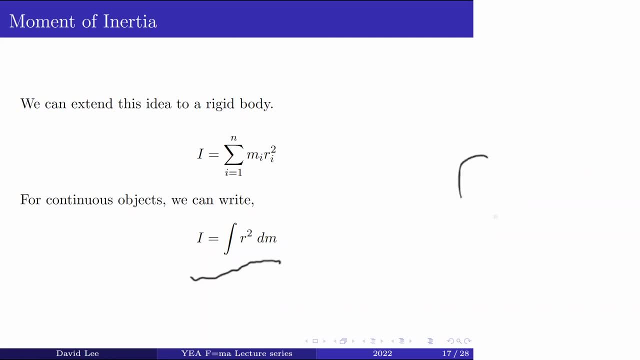 So if we have something like a disk, we can just- and it's rotating around its center, We can just split it into tiny pieces And for each piece that's a small mass DM. We just multiply by its R squared And take the integral, which is basically summing up. 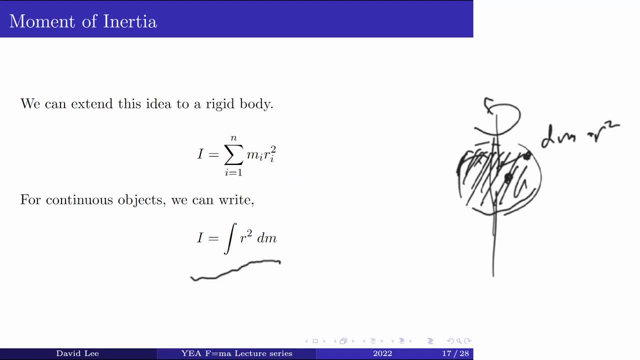 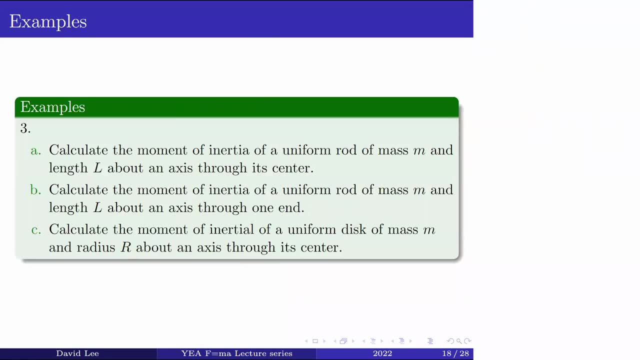 Everything, And that's how we find the moment of inertia. So let's do some examples. I'll give you a few minutes to think about these And, as always, if you have any questions, you can ask me or send me your answers in the chat. 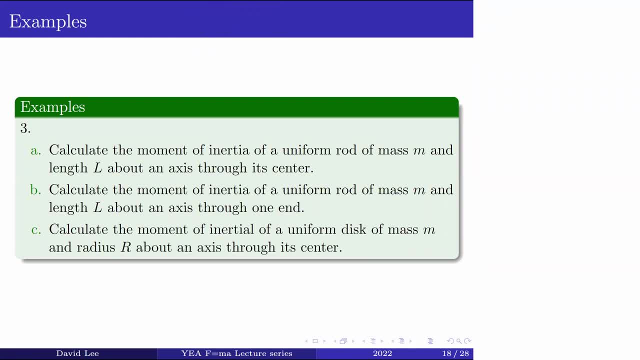 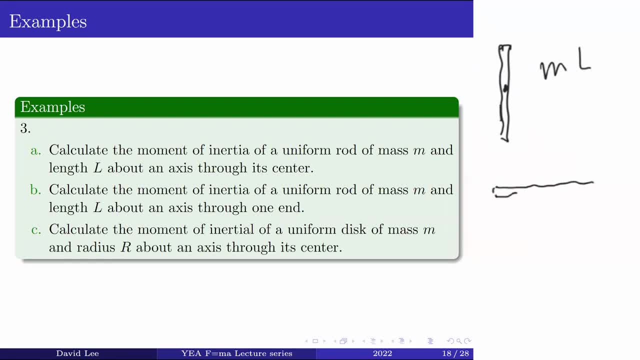 if i draw this in 3d kind of, this will be the axis and it's rotating around there. okay, so what is its moment of inertia? well, it's a continuous moment of inertia. so, in order to draw this rod, we have to use our formula of: i equals the integral r squared dm. 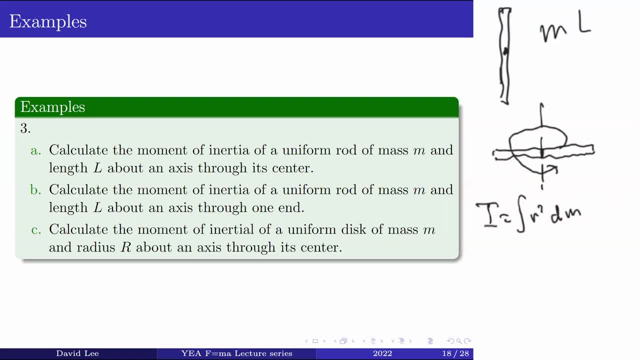 all right. so what is a small mass element here? well, if we think about a rod and we chop it up into tiny pieces and each piece has length dr, well, what is the mass of each piece? well, it will just be m times dr over l, all right. 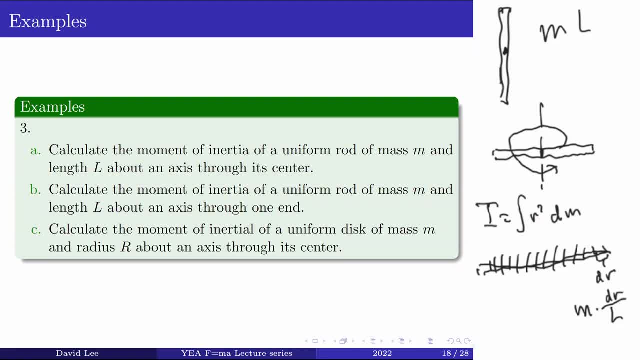 and so if we plug this in, what we should get is i. i equals integral r squared times m, times dr over l. well, it goes from negative r over two, l over two to plus positive l over two. so those are our legs and physical r로downPR ا English Vocabularies, wwwB. robićaongcom. 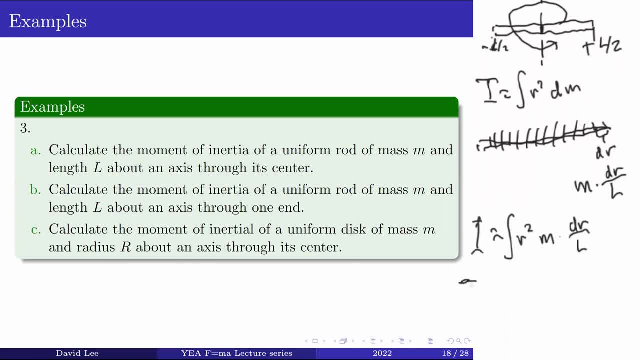 limits of integration. So let's do this integral: Negative l over 2 to l over 2 r squared m over l dr, And this will be m over l times one-third r cubed from negative l over 2 to l over 2.. 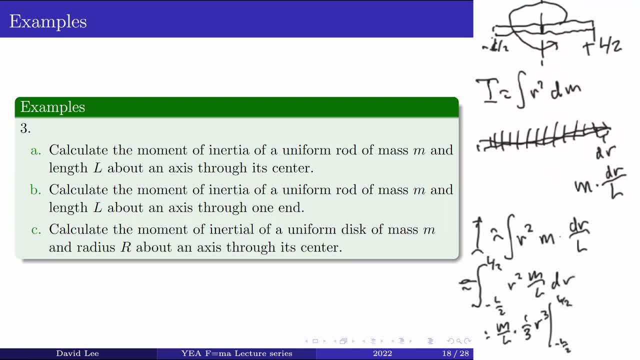 And if you plug in the limits, you should get that this is equal to one-twelfth m l squared. All right Now. hopefully that gave you some idea of how to do these, how to calculate these moment of inertias for such objects, And so I'll give you a little bit of time to do this. 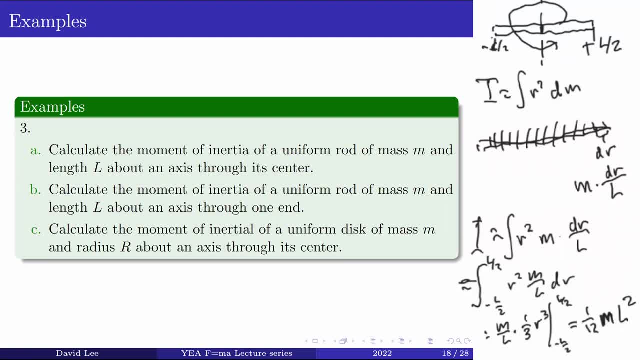 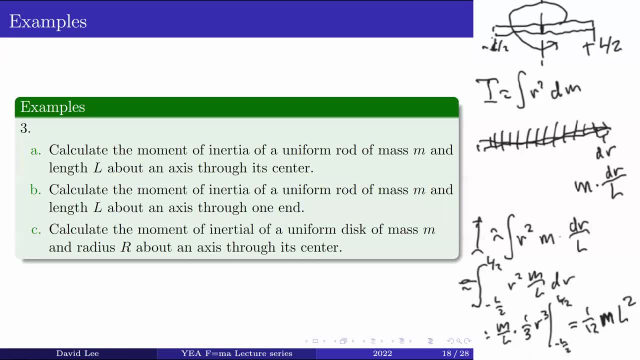 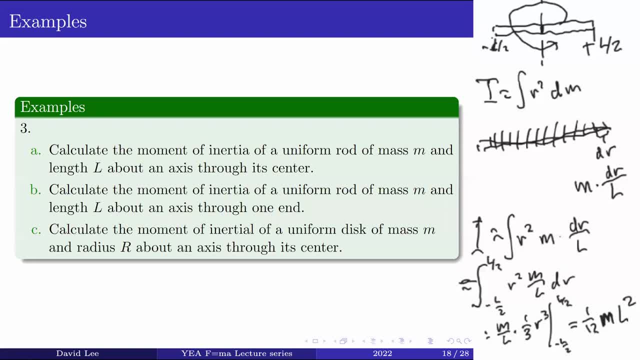 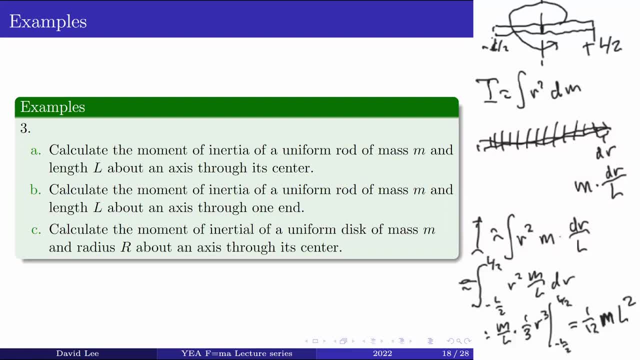 And then I'll give you a few more minutes to try parts b and c. So all right, So let's, let's talk about parts b and c now. So part b is asking us to calculate the moment of inertia. This is also a uniform rod. 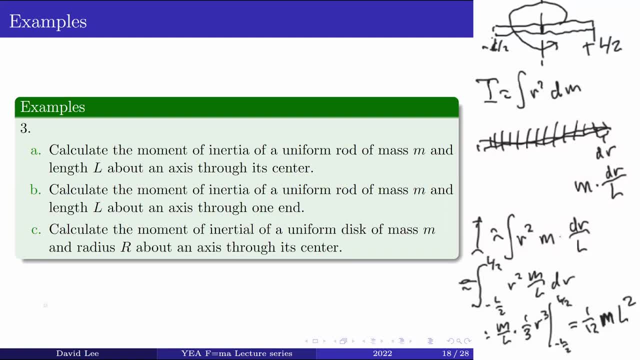 But it's round and axis through one end. So, as I said earlier, which axis? it's around changing the moment of inertia. So before we had something like this, Now we have something like this. All right, But the equation is basically the same. 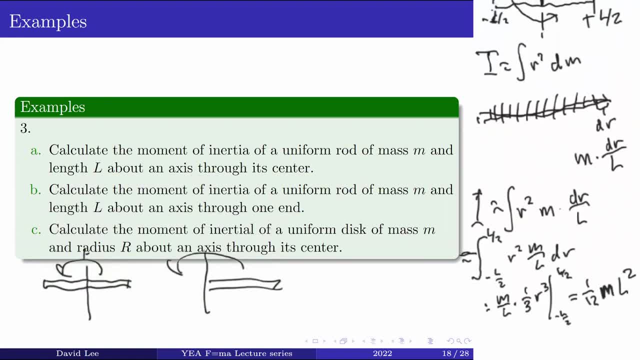 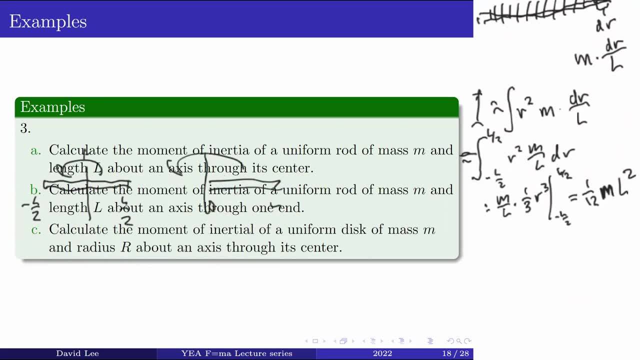 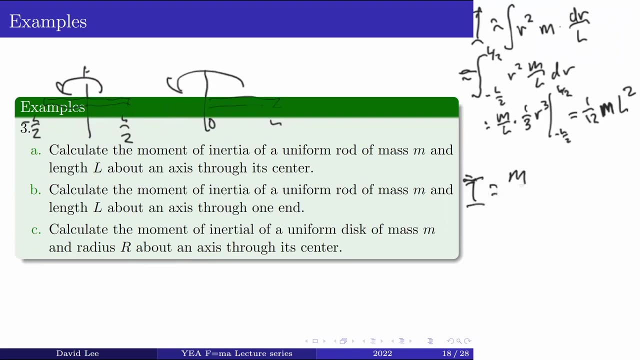 We just have to change our limits of integration. So before it was negative L over 2 to L over 2. Now it's from 0 to L, So we can use the same formula for it's M over L, one-third R cubed from 0 to L. 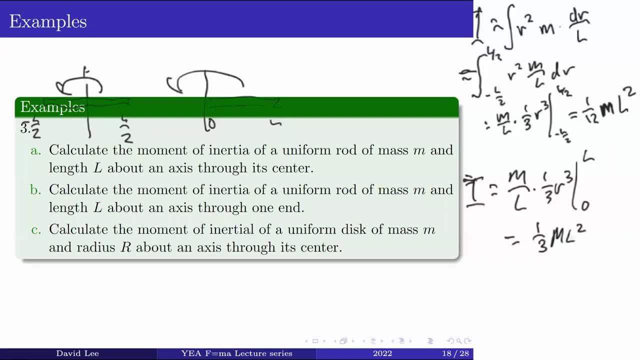 And this is just one-third ML squared. All right. Part C is a bit trickier, because we have a disk Now a disk is two-dimensional Instead of our one-dimensional rod. So how would we approach this problem? So we have to split this up into many different masses. 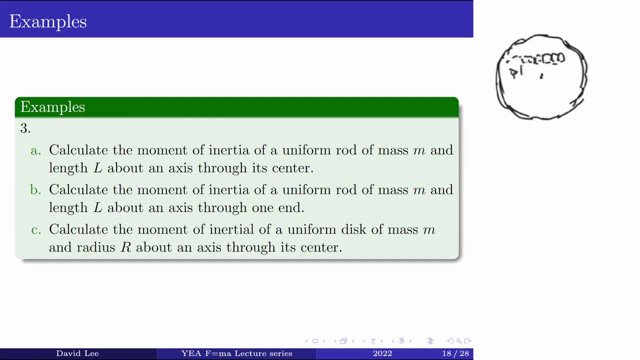 And then, for each one of these, calculate dm times R. So let's first split it up into. how will I do this? Let's split it up into dx's and dy's, Like this is we're going to integrate in Cartesian coordinates for now. 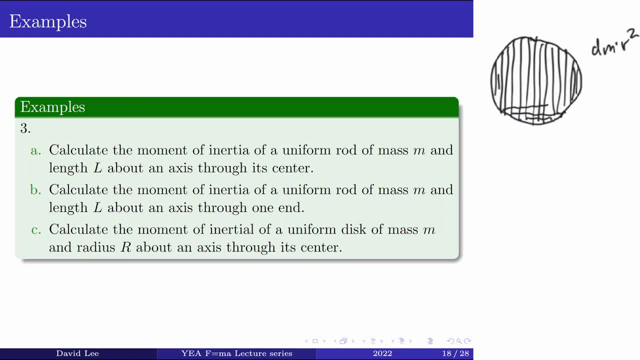 Just as an example. Normally, if you know polar coordinates you can probably see that it's going to be easier in polar coordinates. But just to illustrate, since probably also some of you don't know polar coordinates very well, So we can have a mass at position x, comma, y. 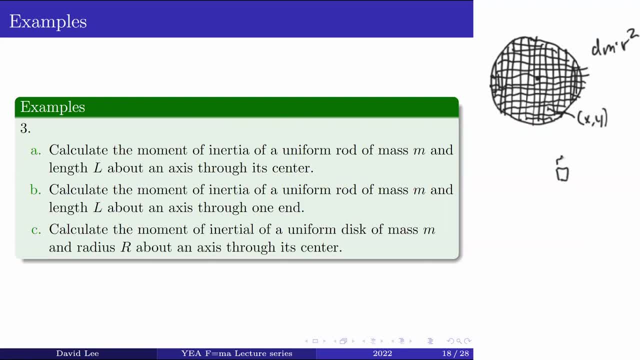 And it's basically a square With length dx and height dy. So what's its mass? Well, that's easy. Since it's a uniform disk, its mass is just m times the area that the square has dx dy over the total area of the circle, which is pi r squared. 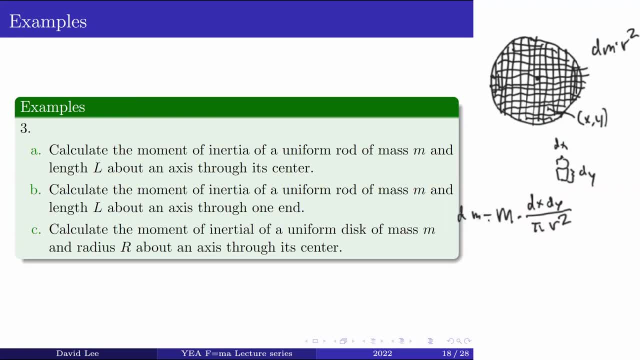 So this is our dm. Okay, Pi, let's use capital R, Because I used lowercase r for the position or radius coordinate, So now we can try integrating. It will be integrating over our circle And we have m over pi. capital R squared times, lowercase r squared dx dy. 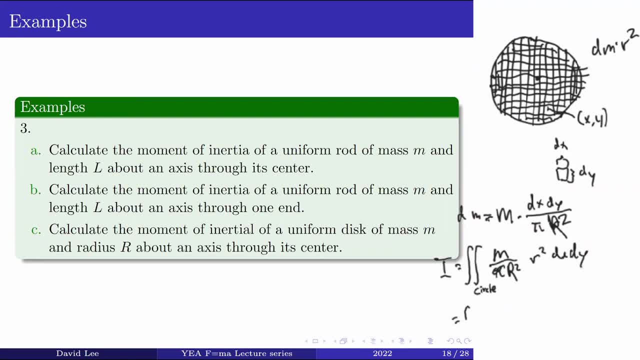 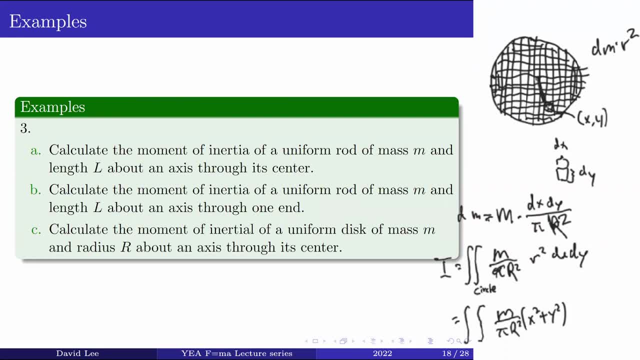 So if you try to find its radius, well that's just square root, x squared plus y squared by Pythagorean theorem. So our r squared is just. So our r squared is just x squared plus y squared, And then dy dx. 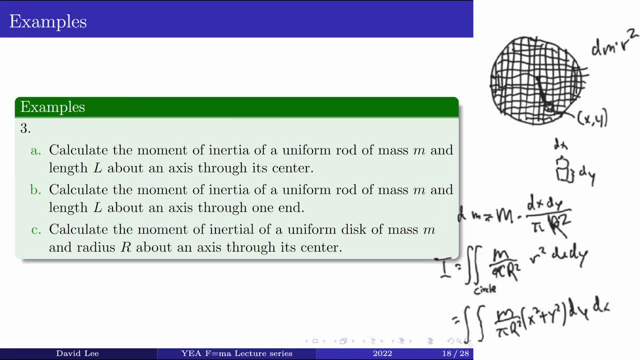 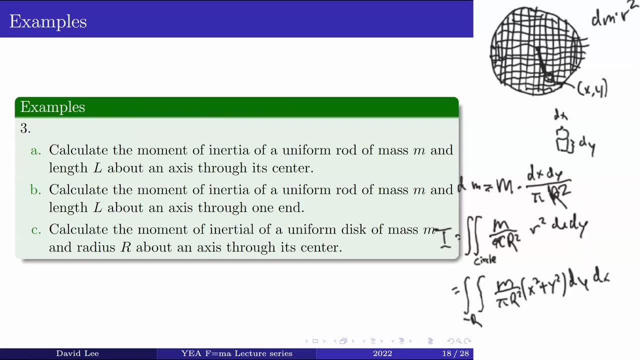 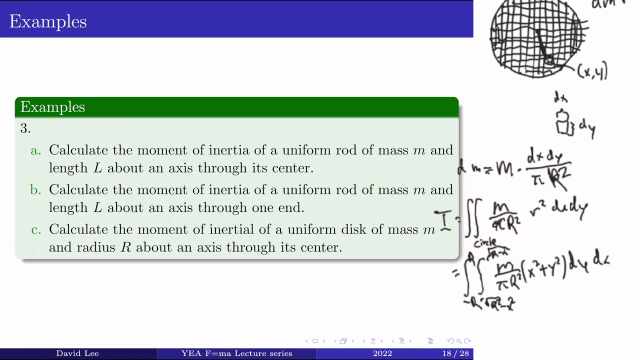 And then we can put on limits of integration. So y x can go from anywhere from negative r to positive r, And then, once you fix x, y will go from root r squared minus x squared to root r squared minus x squared. Oh, that's hard to. 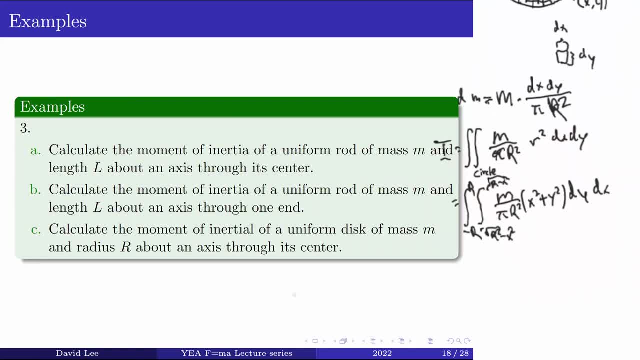 That's hard to tell. Okay, I'll rewrite it bigger. Our moment of inertia is the integral from negative r to r. integral negative root r squared minus x. squared root r squared minus x squared M over i r squared times: x squared plus y squared. 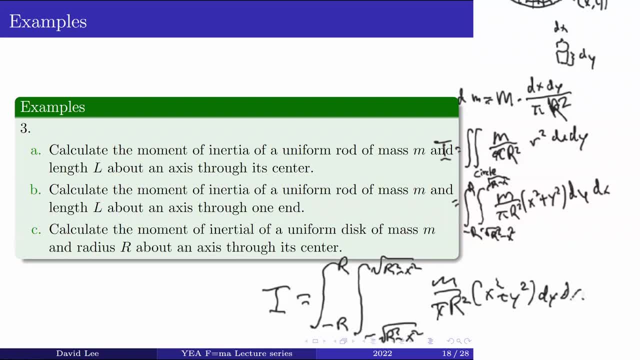 dy dx. All right, And this isn't too hard of an integral, Hopefully I think Yeah, it looks okay, But it is quite tedious And, by the way, if you do this, you should get an answer of one half m? r squared. 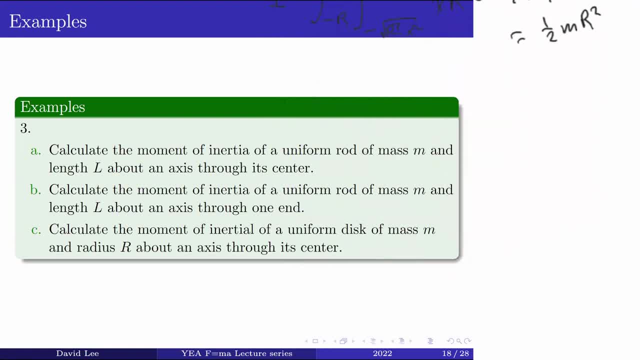 Which is the answer. But there is a faster way, which is using symmetry. So a lot of times in physics you can use symmetry to make your calculations easier and much quicker and not messy like that. So instead of splitting it up in Cartesian coordinates, what we can do is just split it up into little rings, like this: 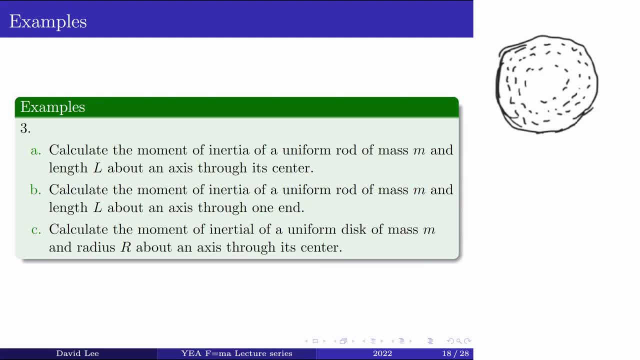 So, instead of splitting it up into little rings like this, you can just use symmetry as a vector. So instead of splitting it up into little rings like this, All right, And Yes, this is essentially integrating and polar coordinates. So Why did we do this? 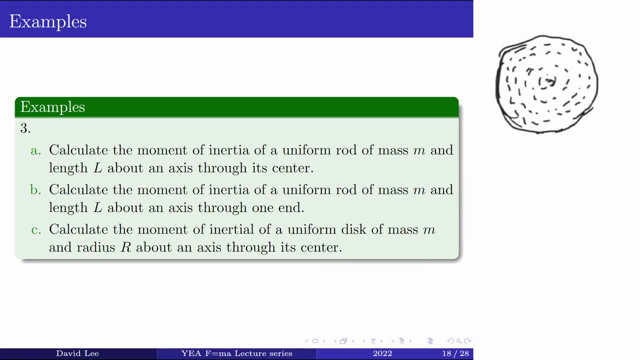 Well, this makes it much easier because in each ring there's the same radius. So when we consider D m, r squared 2. Well, we have the same radius, so we'll just add up all the dm's and then multiply by r? squared. 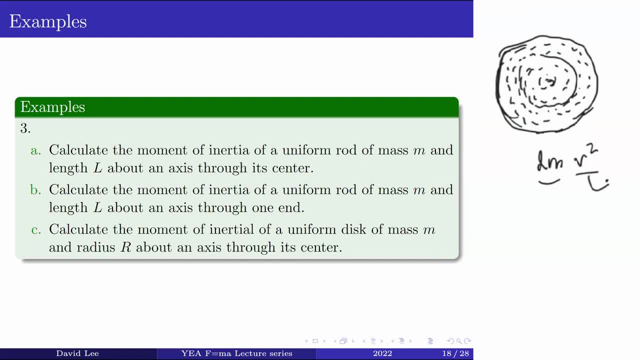 So what is the mass of one such ring here? Well, what is its area if it has radius little r and thickness dr? Well, we can think of it kind of like, I guess, a collection of small rectangles. So if we cut it here and unfold it, we'll just get a large rectangle. 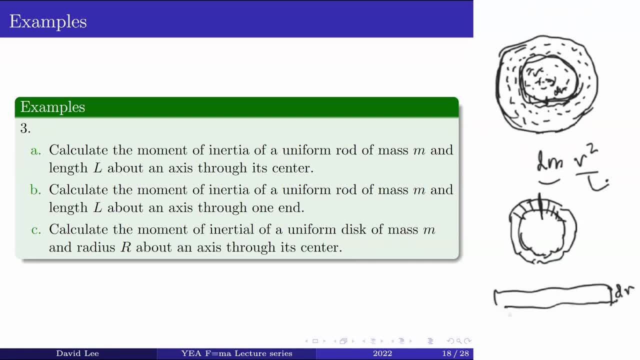 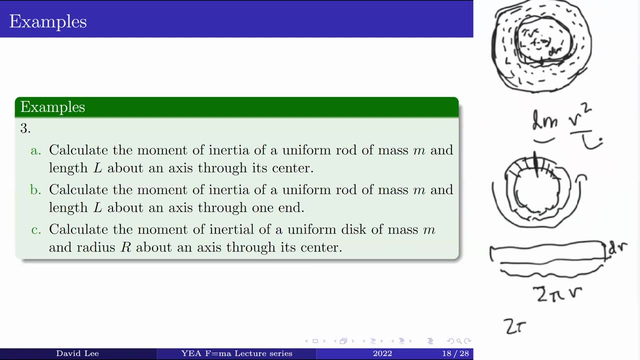 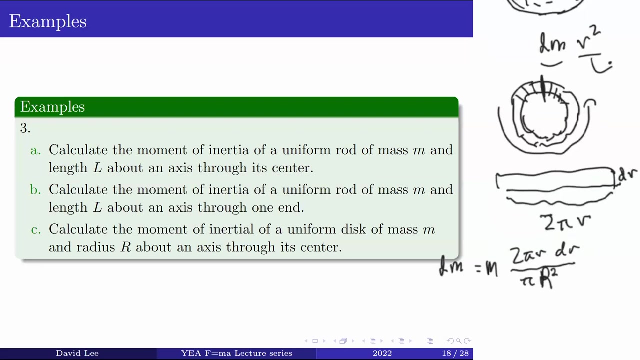 It has thickness dr and length 2 pi r, because that was the original circumference. So now its area is just 2 pi r dr, So its mass is m times its area over the entire area And this should simplify to be 2 m r over 2.. 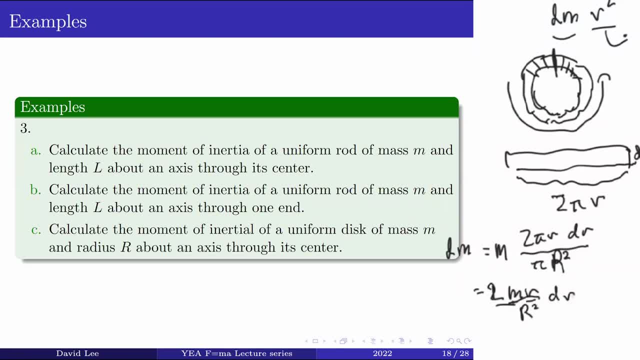 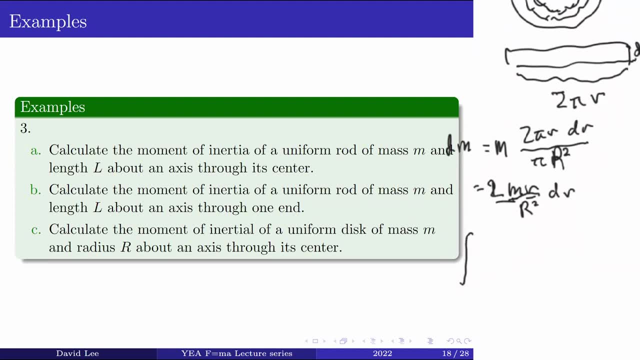 r squared dr. All right, cool. So now all we have to do is integrate this from 0 to big R. We have 2 m r over r squared times, r squared dr, And this will be just one half r to the fourth over r squared. 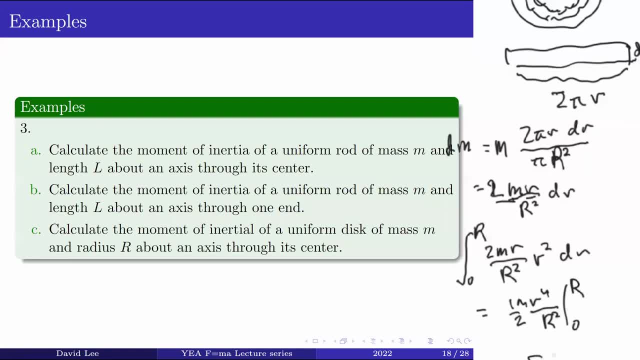 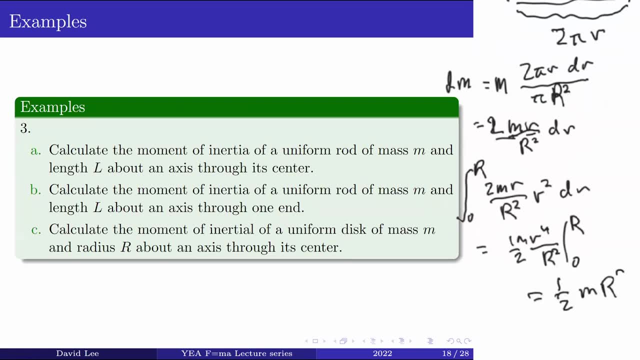 times m, of course, from 0 to r, which is one half m r squared. So we get the same thing, but it's just much easier this way. All right, Now it is 2: 37,, which is seven minutes after 2: 30,, which is when we were supposed to have our break. 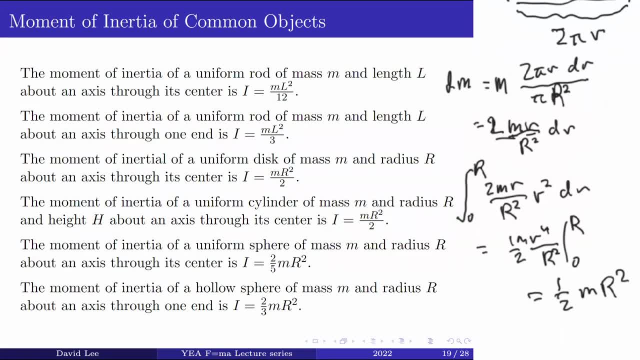 But so I'll just give you this big list of stuff. Yeah, We already calculated a few of these, And well, you should know how to calculate all of these, But during the contest it will be very time-consuming to recalculate these every time. 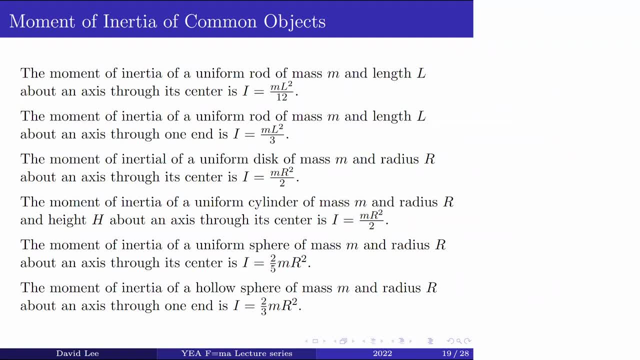 you need to use them. So I would recommend, like knowing some of the. yeah, I would recommend just knowing some of these very common ones So you don't have to recalculate them each time. And with that I will give you guys a five minute break. 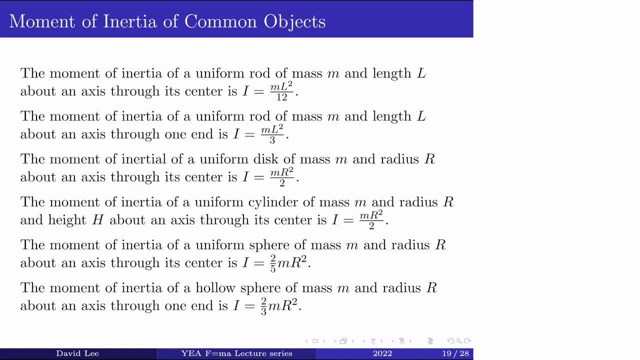 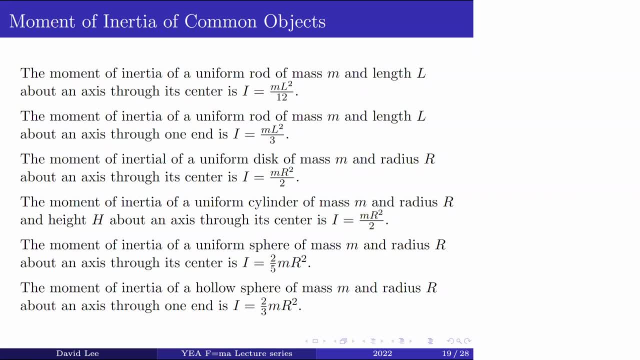 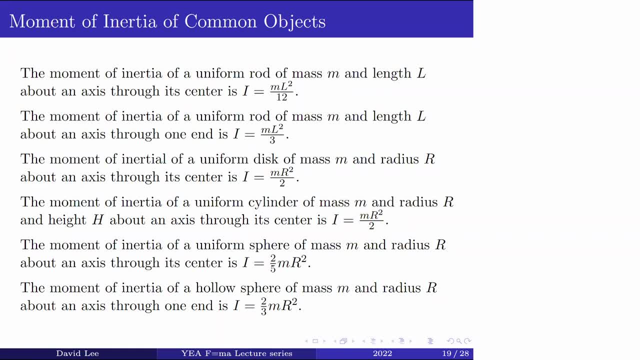 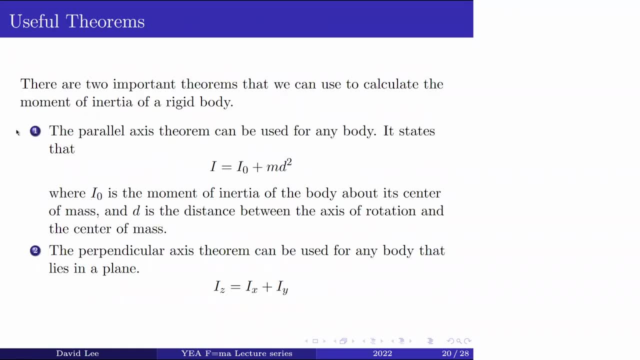 So let's get started. Well, let's talk about two useful theorems, because you won't always be able, you won't always be able to, you won't always be able to always be given one of these common objects here. So these theorems can help you with that. 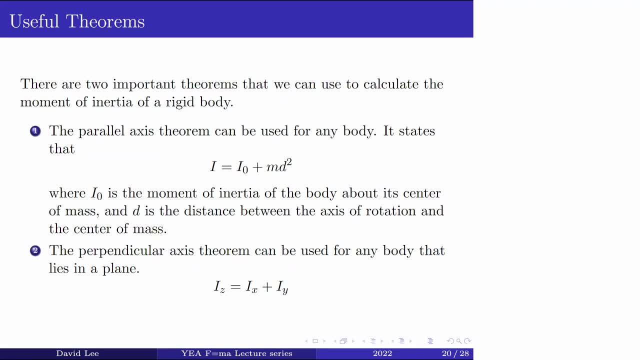 So the first theorem is the parallel axis theorem, And what the parallel axis theorem is saying is: if you have an object, it can be any object, So some weird object like this, and any axis too. Okay, not any axis. The axis has to pass through the object's center of mass. 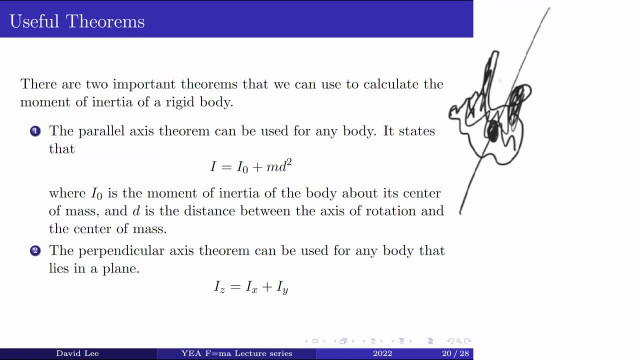 But other than that, any axis through its center of mass, so whatever direction you want, And it's rotating around this axis and it has a moment of inertia, I zero. If you draw a parallel axis, that's a distance D away, And now all of a sudden it starts rotating. 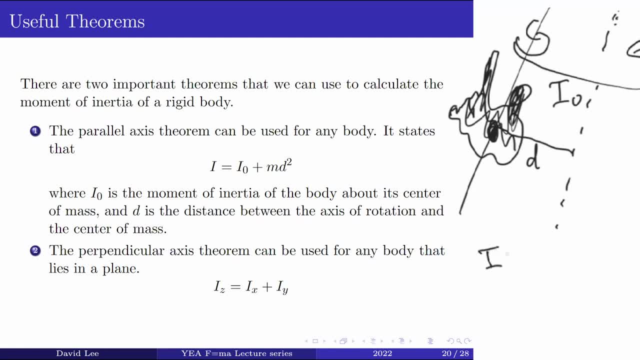 around this new axis, The moment of inertia will be I zero plus M. D squared, M is just the mass of the object. All right, so this theorem is very useful And another one which is slightly less useful, but still kind of useful. 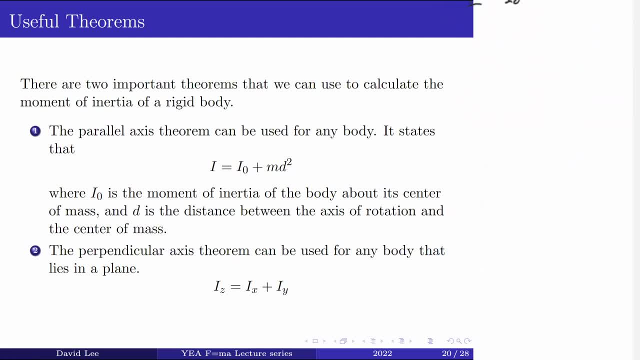 is the perpendicular axis theorem, So this is not as applicable to as many objects, because this only applies to pancake-like objects. and what it states is that: so we have like a pancake here and it has to lie in a single plane, so it has to be completely flat, and what it says is that if it rotates, 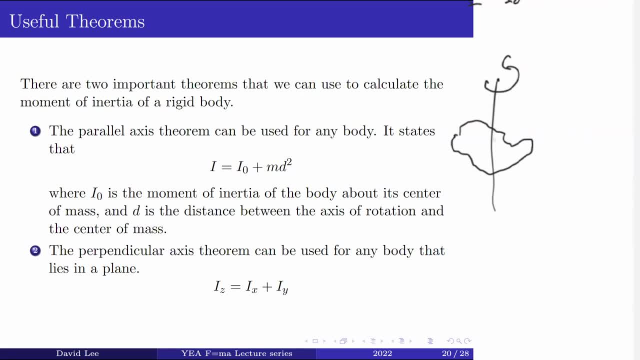 around this perpendicular. so I guess in this case, if we define axes, x and y are here and z is here, so say x, y and z are perpendicular axes and our pancake lies entirely in the xy plane. what this theorem basically states is that the moment of inertia 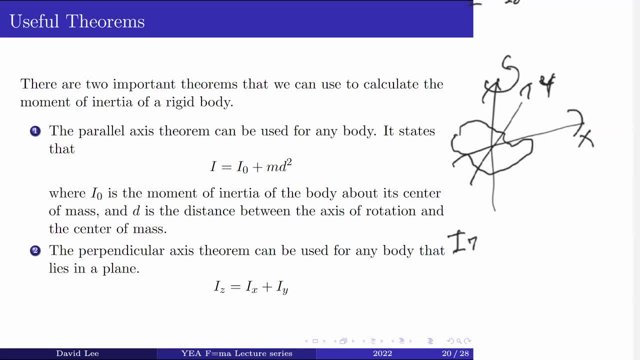 around. And the z axis, which is perpendicular to the pancake, is the sum of the moments of inertia of the x axis and the y axis and the x and y axis axes- Actually they can be any axes, as long as they're perpendicular and in the same plane of the object. 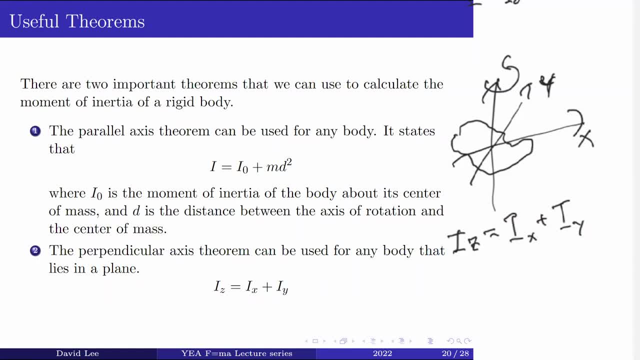 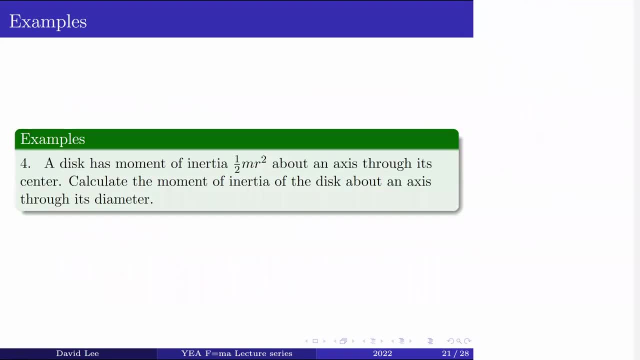 All right, So let's go on to a quick example of this. All right, So let's go on to a quick example of this. All right, So let's go on to a quick example of this. Thank you, You, You, You. 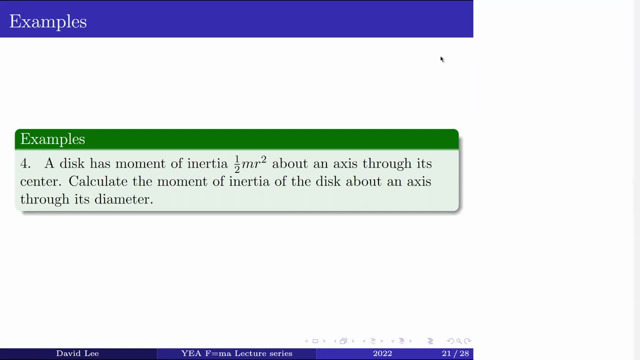 Okay, it's been a while, Let's just talk about this. This is actually a relatively simple problem once you see the trick. So what it's asking is: we have some disk, an axis, Okay, first of all, it's hard to draw. So we have a disk and it's rotating. 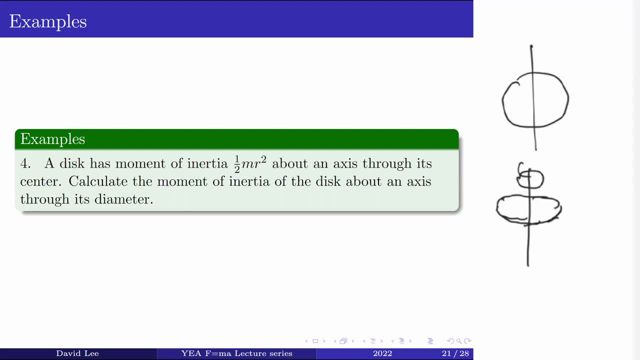 through an axis around its center, and we just derived, a few slides ago, that its moment of inertia is one half m r squared. Okay, so now in the case of this, where it's rotating around its diameter, this is very hard to draw, but it will be like spinning. 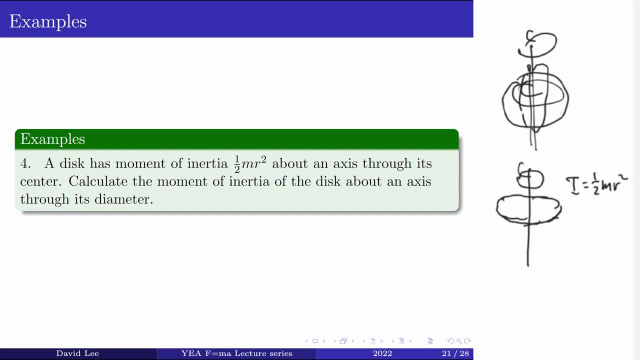 like this way. How to draw it? Anyways, it's rotating around this axis now. So what is its moment of inertia now? Well, to do this, we can use the perpendicular axis theorem. So Okay, but this is a bit different, because with the perpendicular axis theorem, 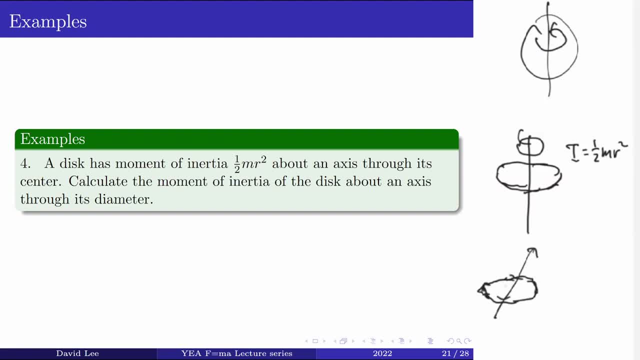 in its original statement. you know two of these moments of inertia and you can add them up to get this moment of inertia, But this is actually the same thing, So we know what this is right. This is one half m? r squared, So we know what this is right. 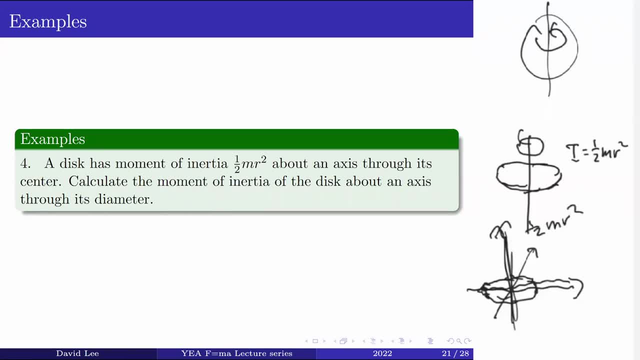 This is one half m r squared And this disc is actually symmetric, So we know that, whatever this, i x will be. i y will also be the same thing, because, well, it's just a circle, right? It doesn't matter, because of symmetry, any axis through its diameter, or basically, 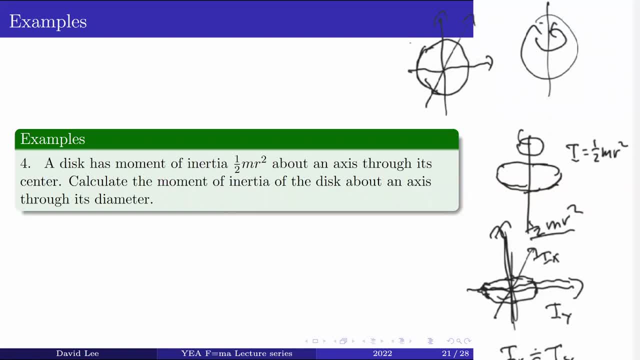 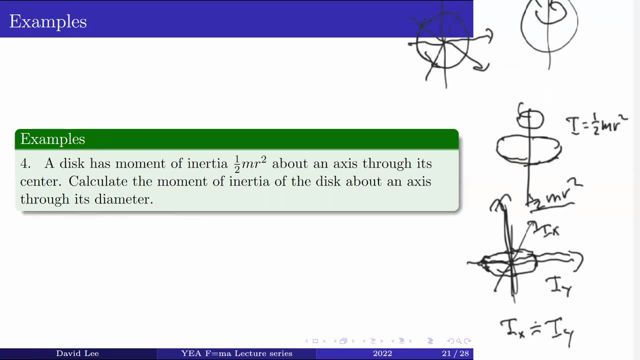 the same things. So the moment of inertia through any axis that passes through a diameter will be the same. Okay, so now we just get that i x plus i y is equal to one half m r squared. but since these are equal, we will just get that. 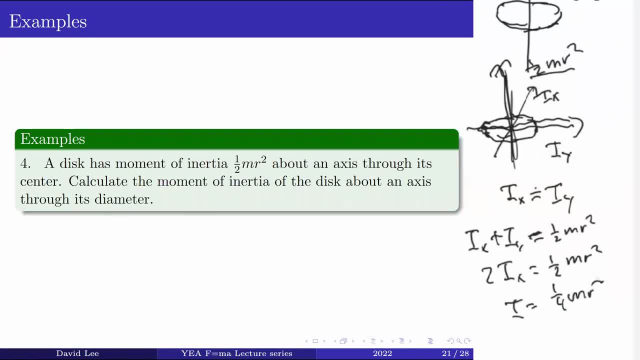 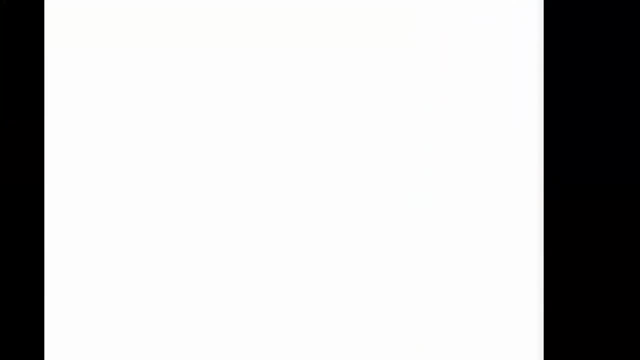 each one is equal to one fourth m r squared. Alright, And that is our answer. So now we know about moment of inertia, So let's just review a bit. Also, one thing important I forgot to mention in my slides is that, Okay, I mentioned this earlier, but it's very important. 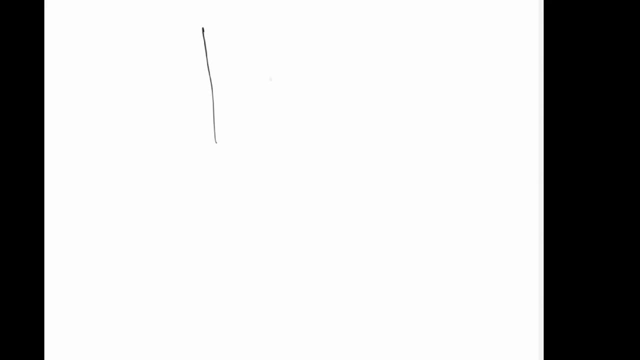 You have to remember which axis you're rotating around, because torque, Oh, that's a big torque. Torque and moment of inertia depend on the axis. So we gotta make sure, like torque with respect to this axis, like if we have forces here, then this will be our r. 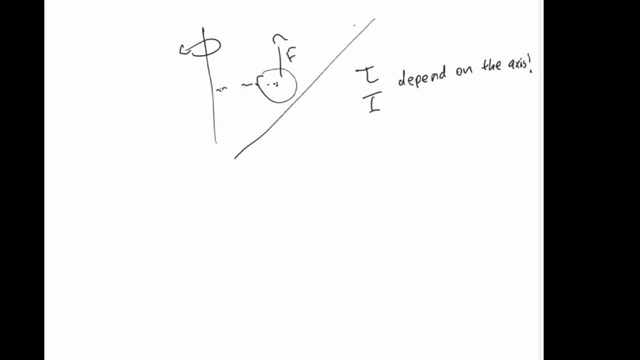 but if it's something like this axis, then okay, this will be our r and also there's gonna be an angle here, So it will be different. But once you calculate torque and i around the same axis, you can use our relation: torque equals i, alpha. So this is basically. 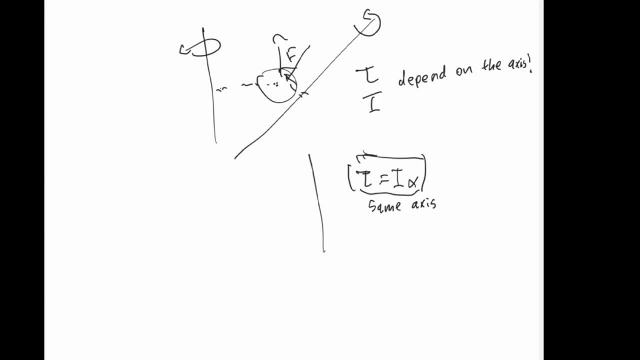 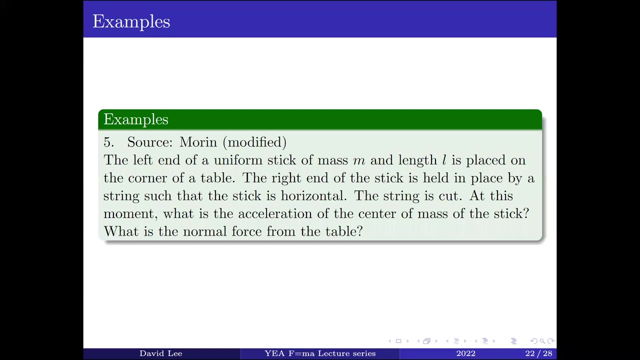 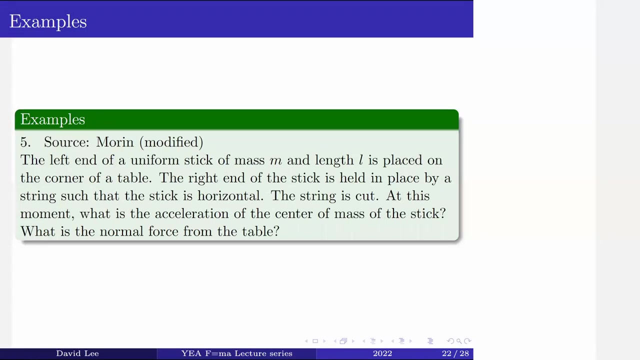 the equivalent of f equals ma for rotation right. So now we can go on to some rotational dynamics problems. They're called Capacitors. Capacitors are the Tactic, Tactic, And What Do you call the Tactic? you, Thank you, Thank you, Thank you. 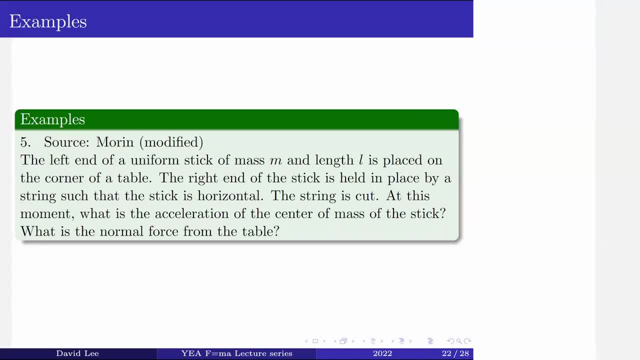 What we have is just to clarify. we have a table- Actually, I do have a diagram- So we have a table, Oh, not in the right place. I have a table here And there's a stick that goes like this: 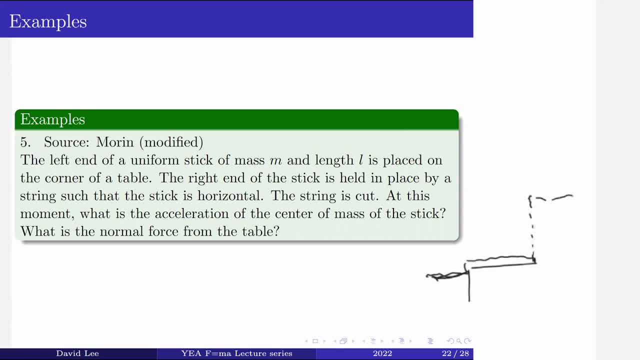 And initially there's a string that's holding it up, but then we cut the string, So now it's going to fall down right. So the problem's asking for the acceleration and also the normal force from the table here. So the problem's asking for the acceleration and also the normal force from the table here. 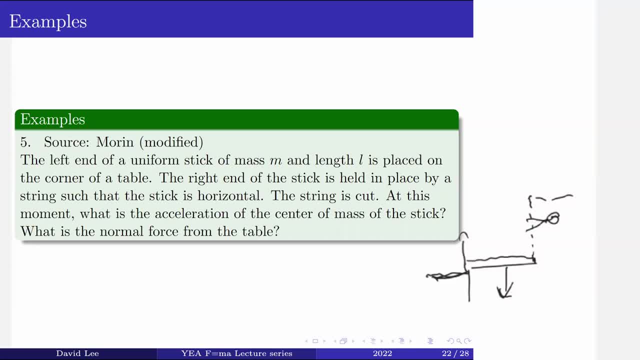 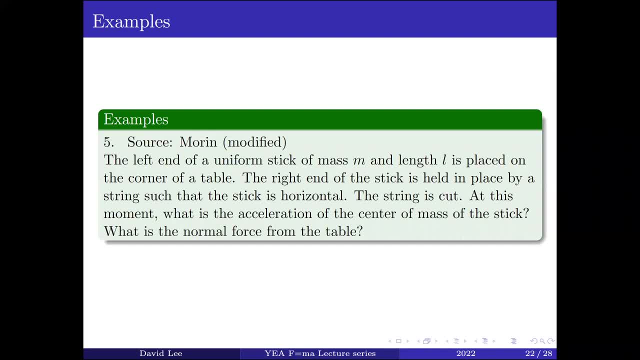 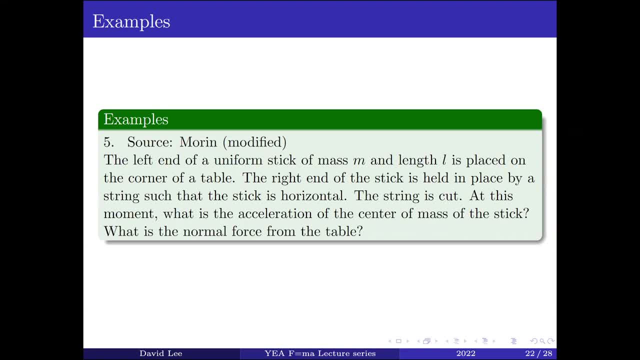 So the problem's asking for the acceleration and also the normal force from the table here. So the problem's asking for the acceleration and also the normal force from the table here. Alright, it's been a while, so let's start talking about this problem. 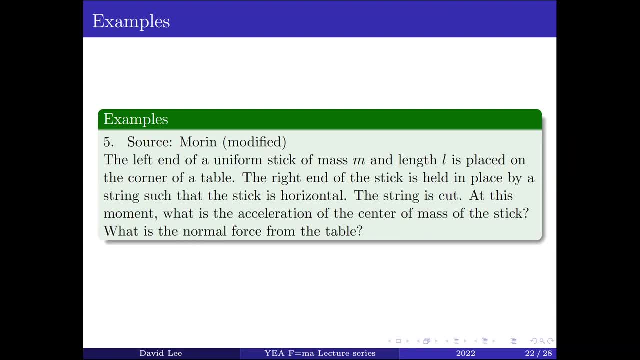 Alright, it's been a while, so let's start talking about this problem. This is quite a tricky problem, So how will we approach this? Okay, if we go back to the diagram I drew earlier. Okay, if we go back to the diagram I drew earlier. 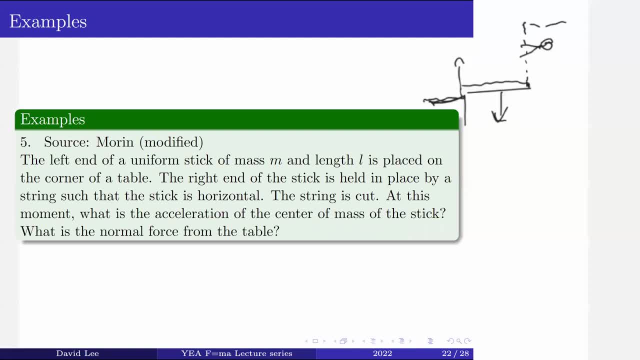 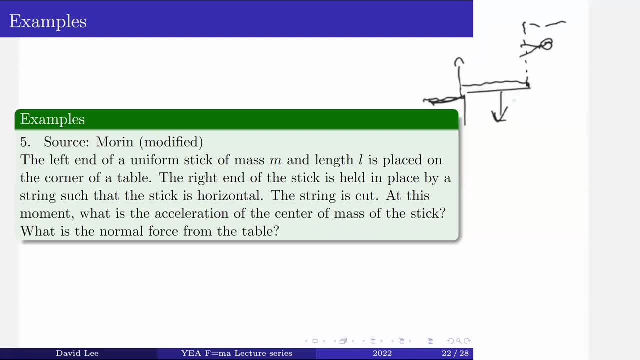 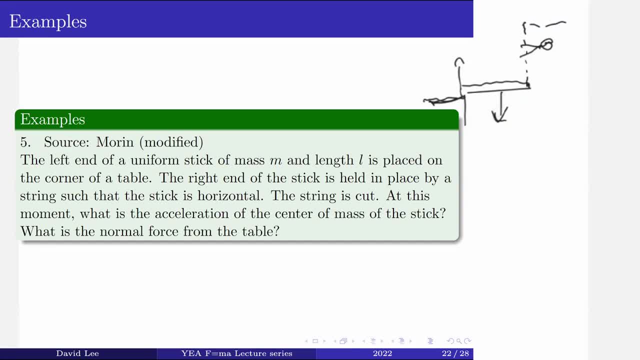 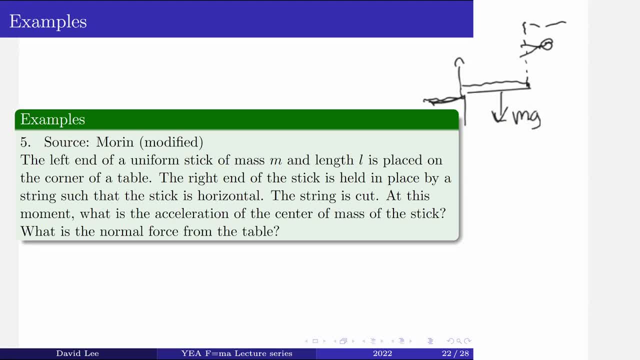 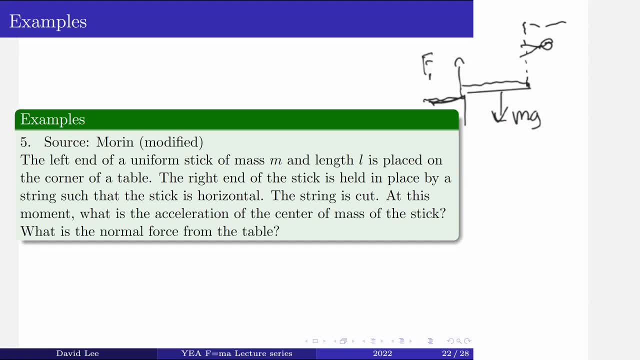 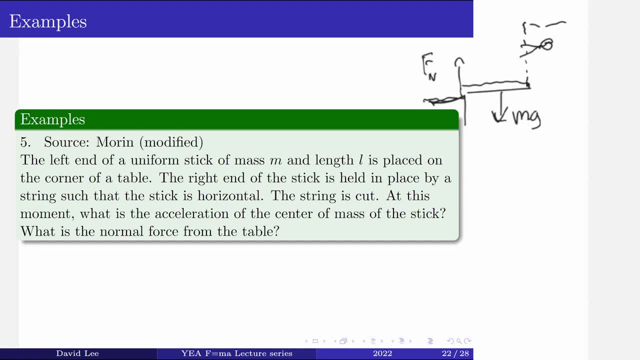 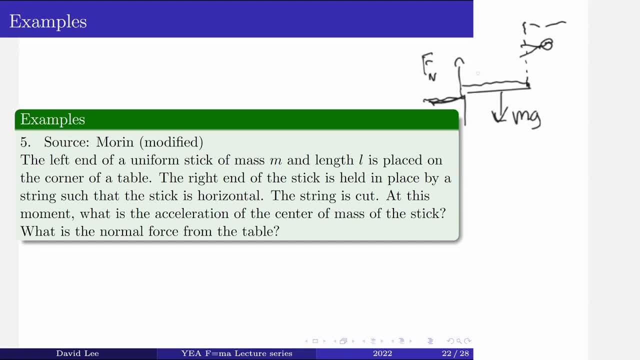 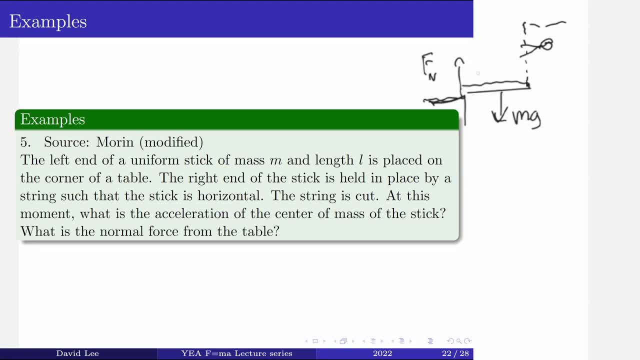 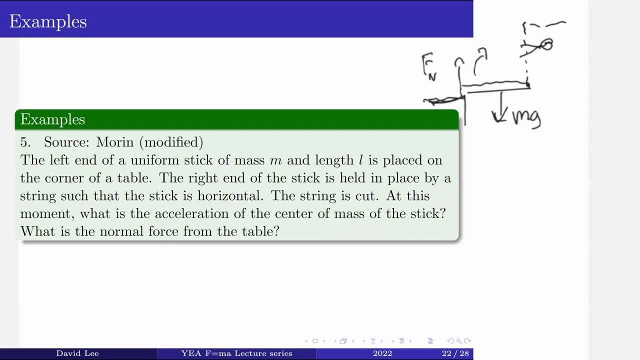 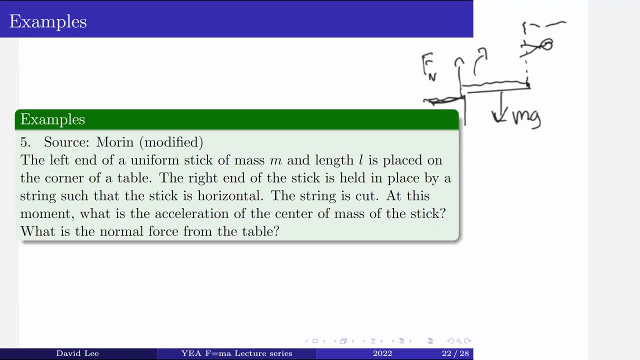 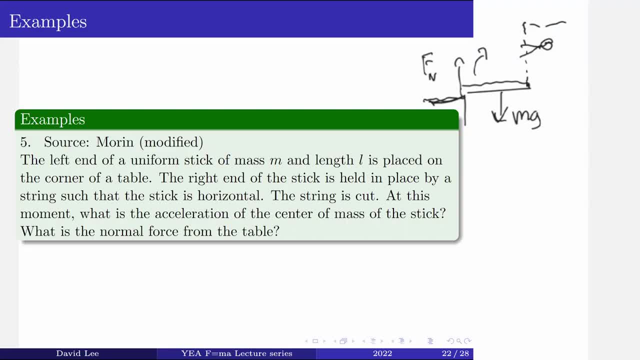 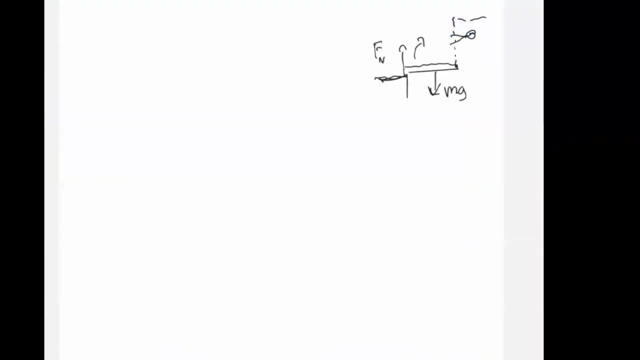 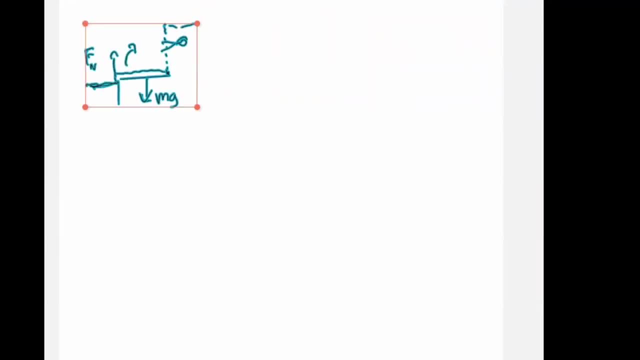 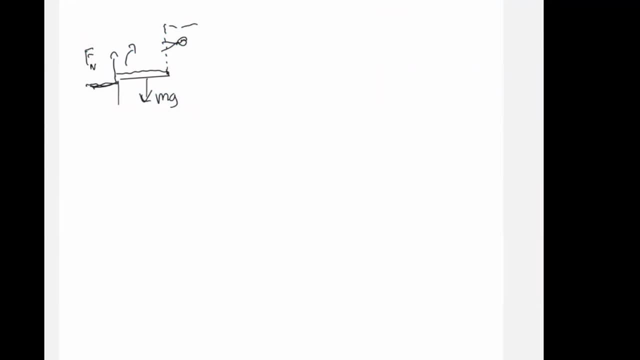 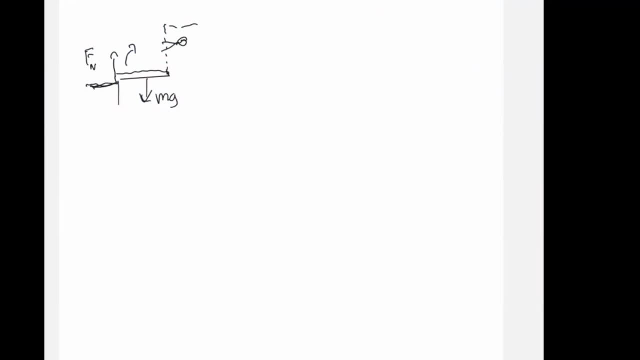 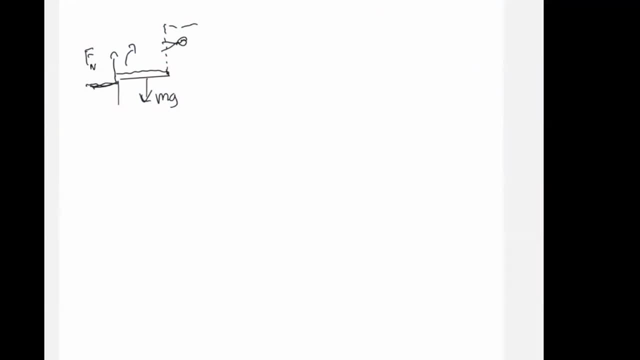 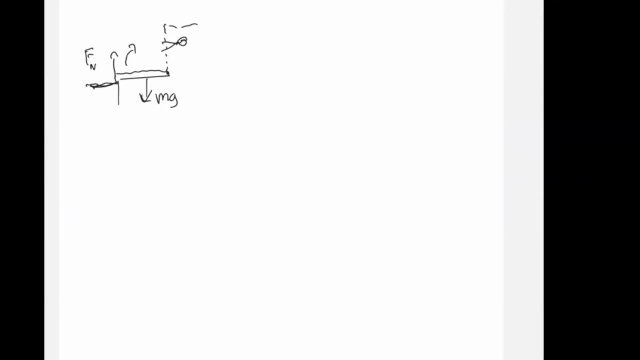 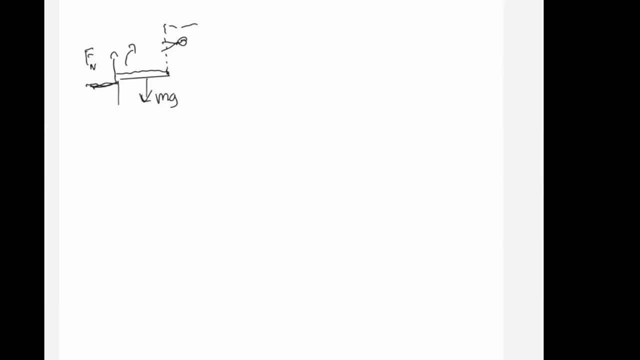 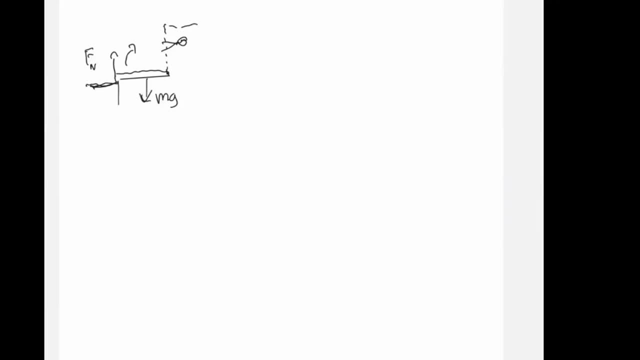 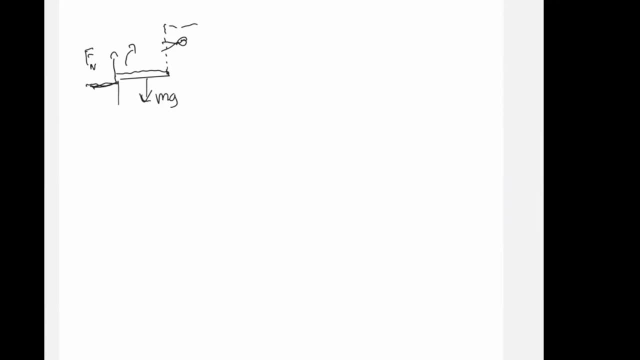 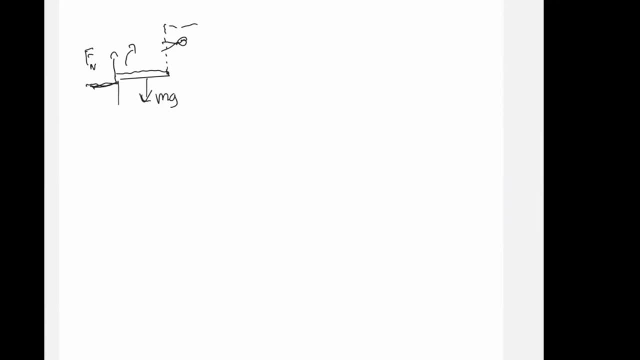 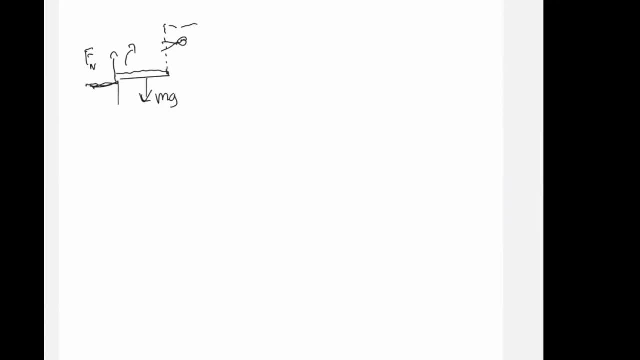 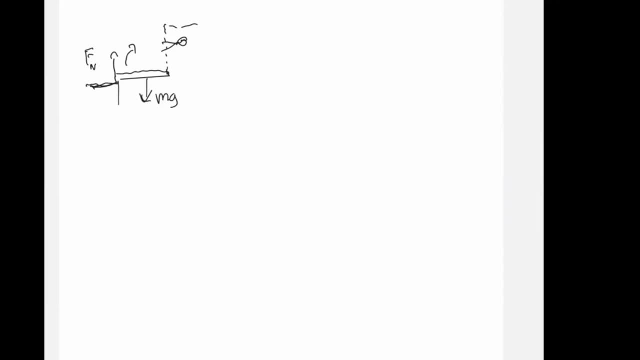 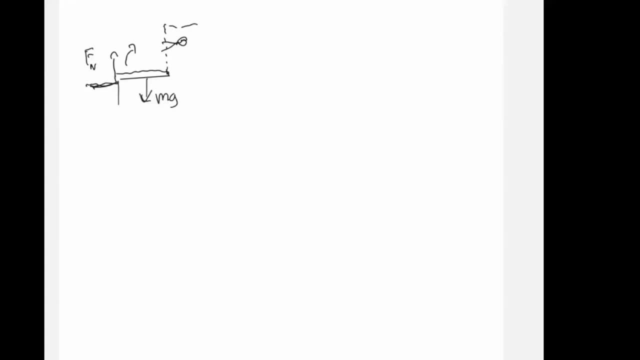 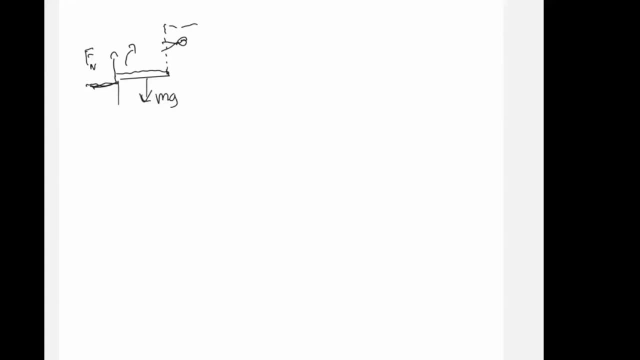 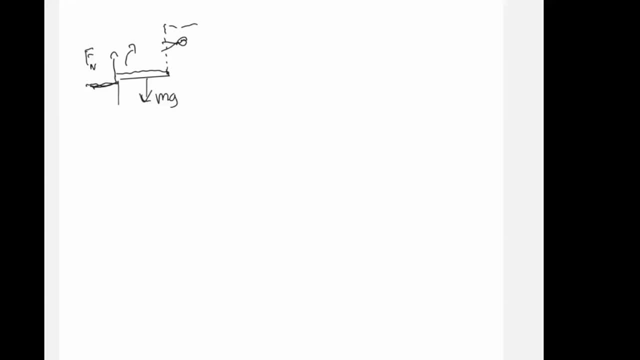 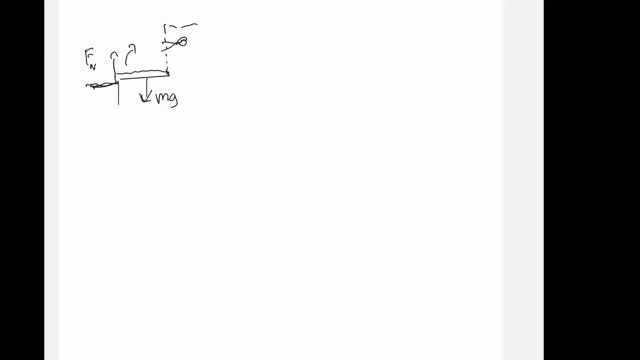 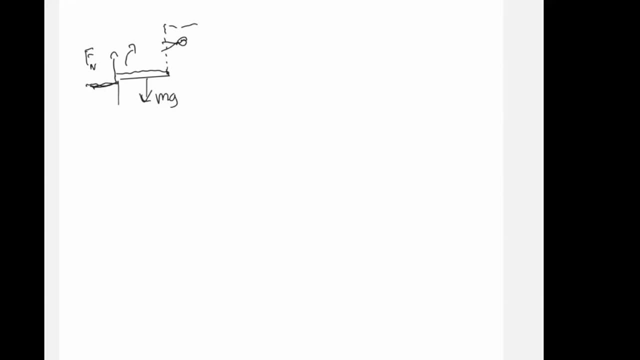 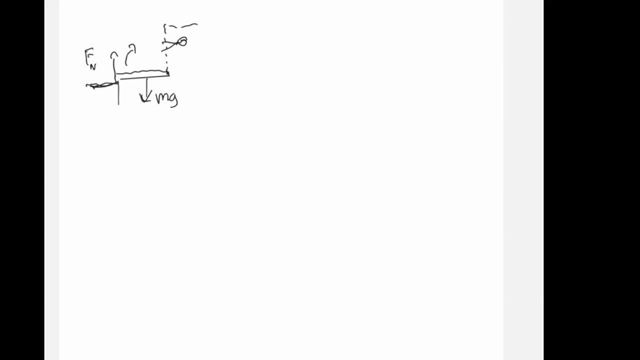 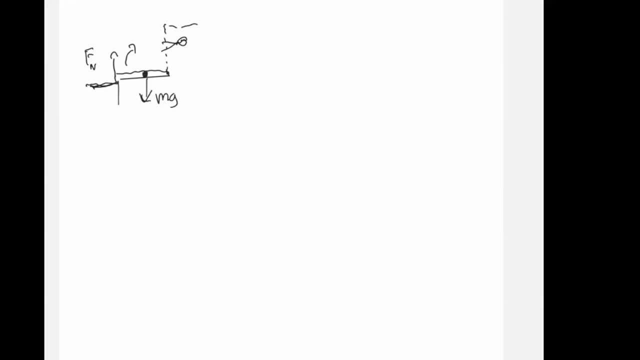 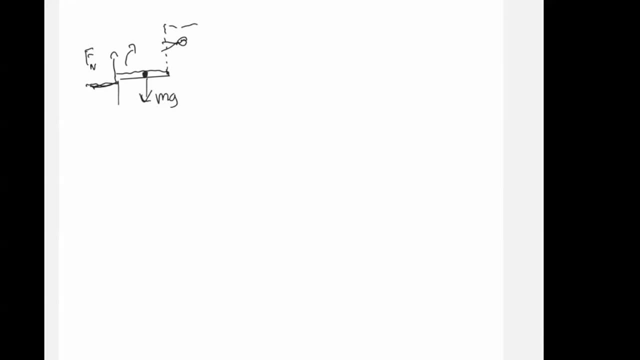 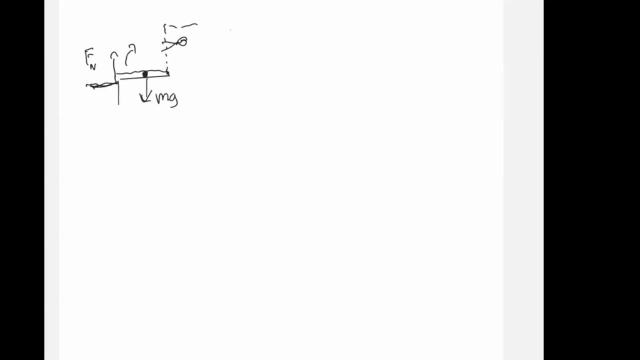 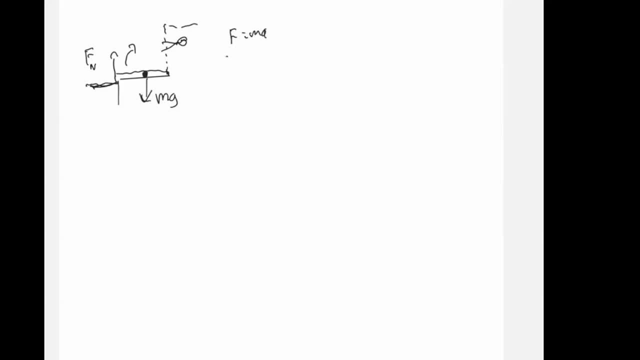 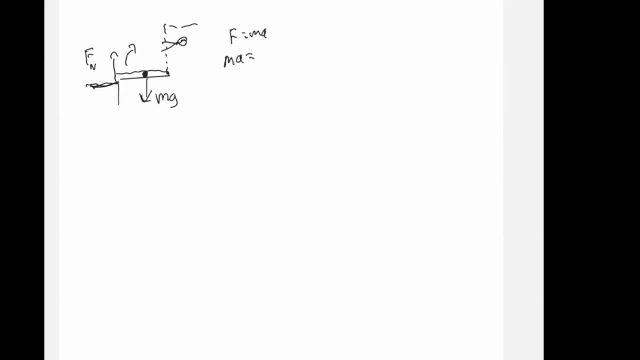 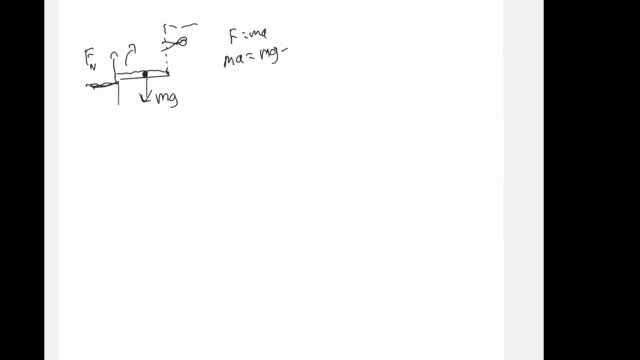 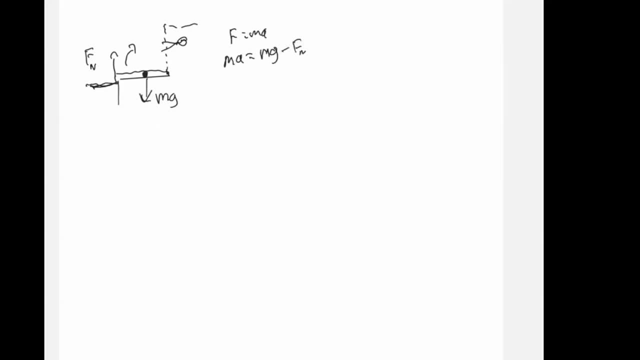 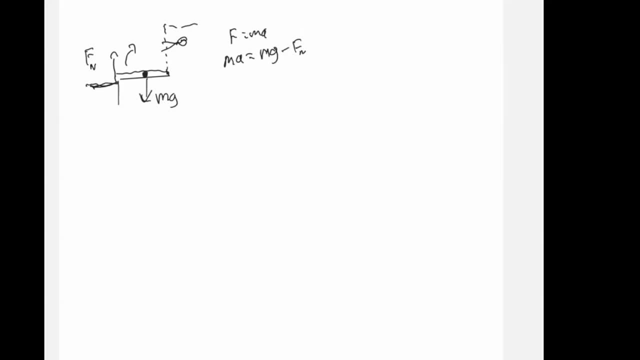 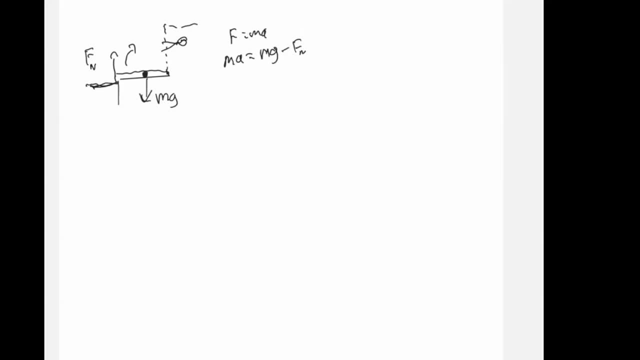 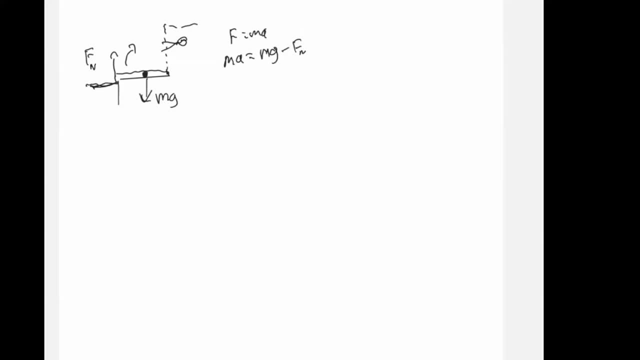 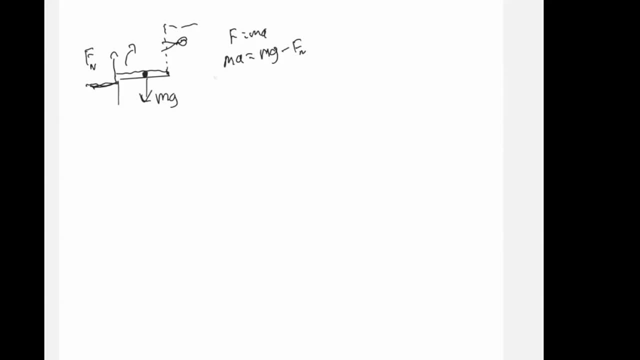 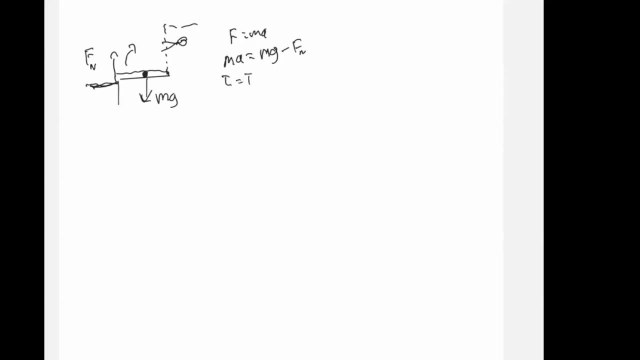 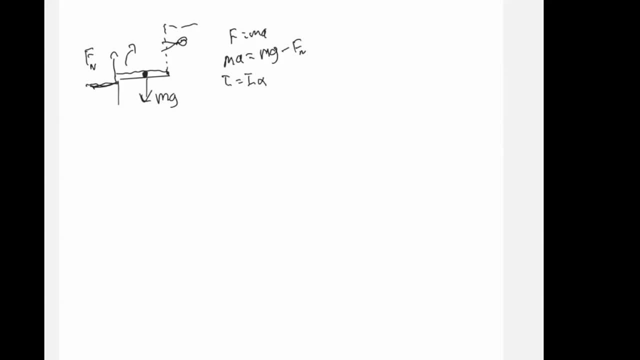 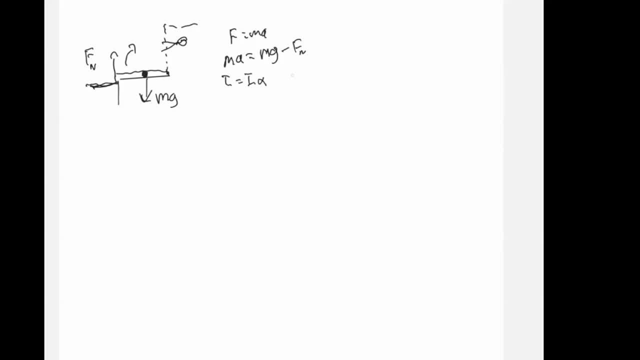 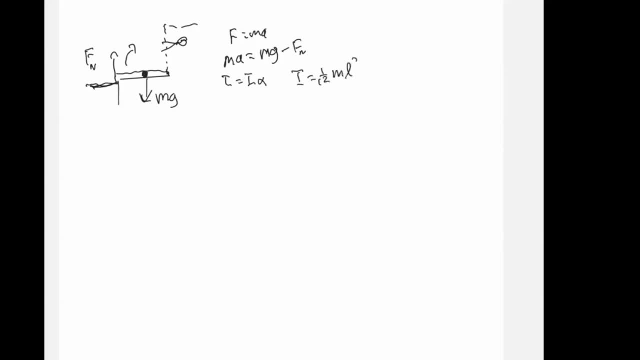 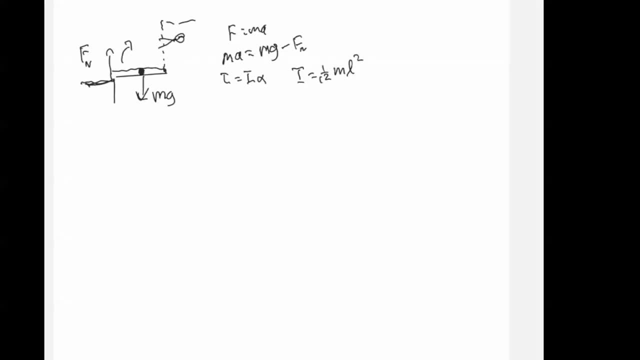 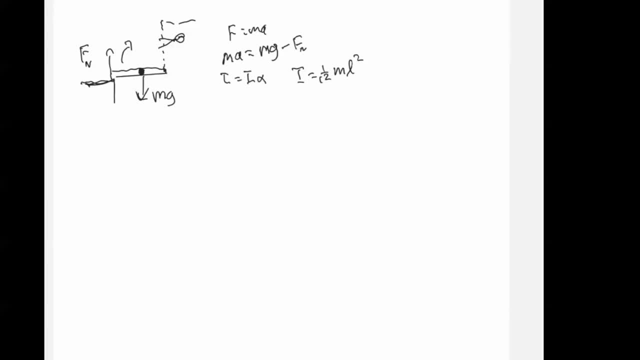 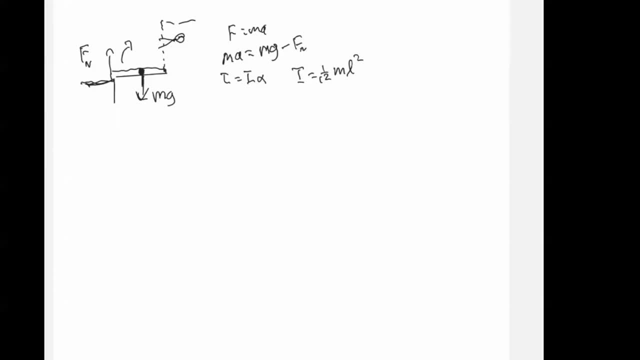 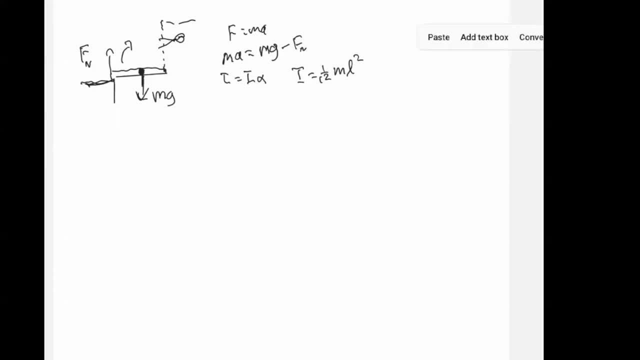 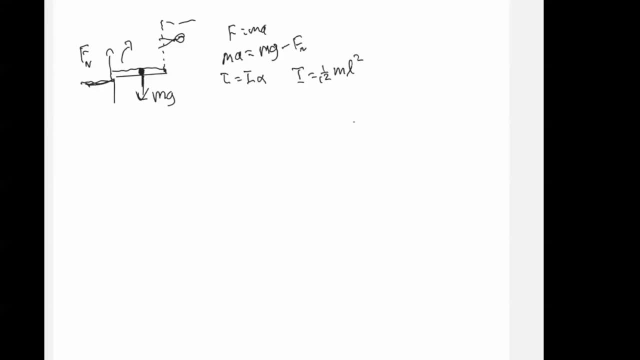 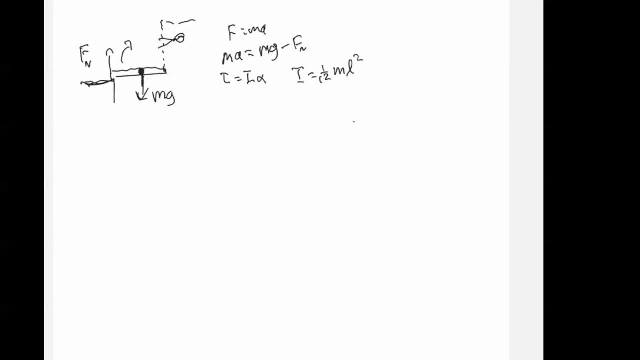 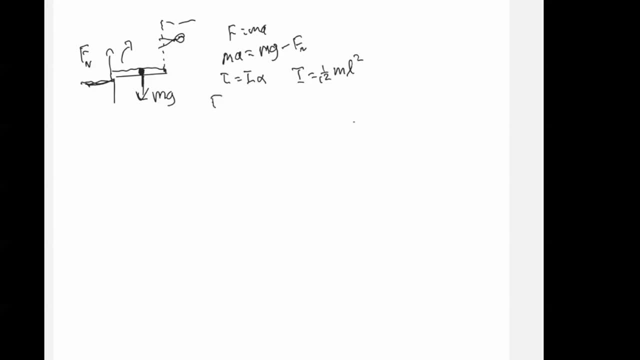 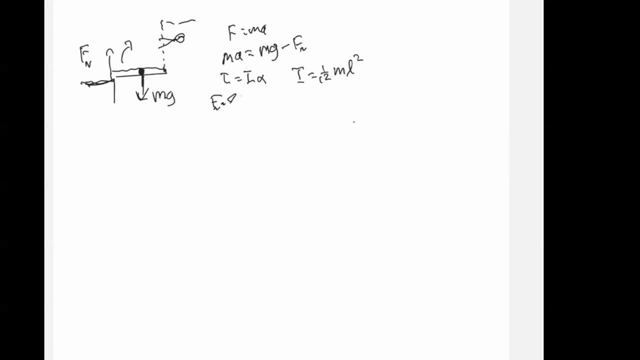 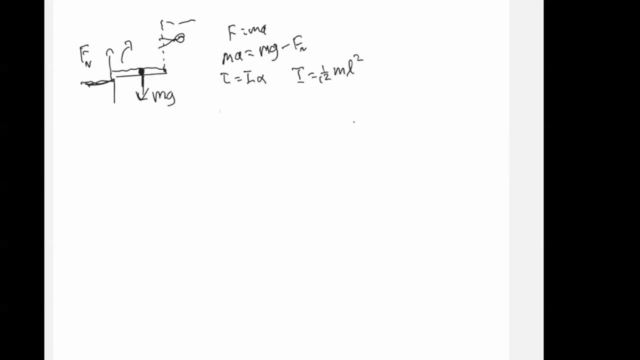 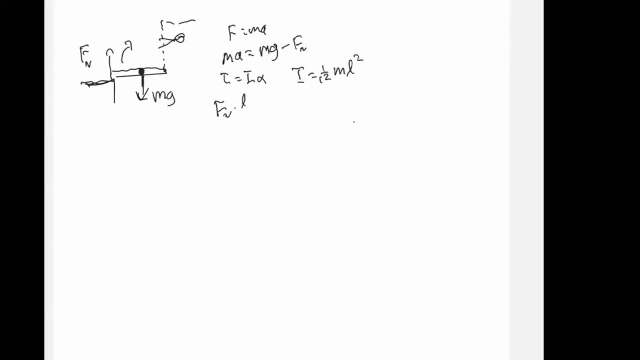 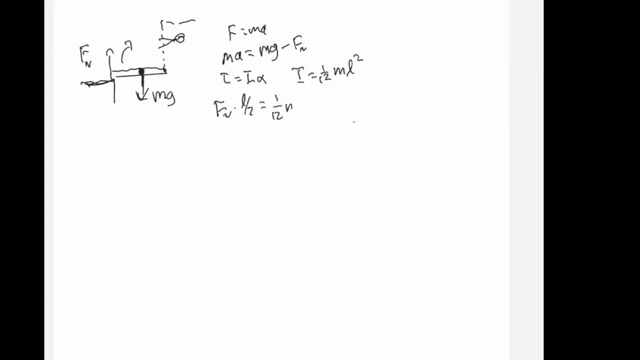 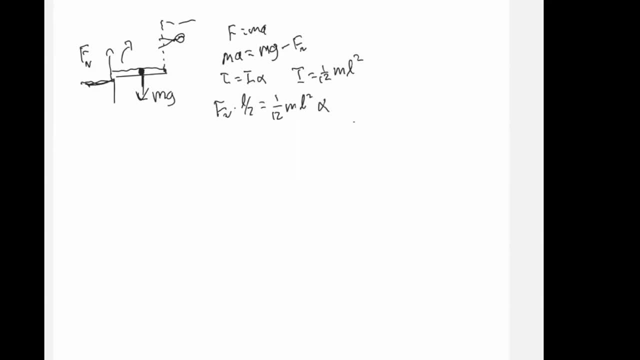 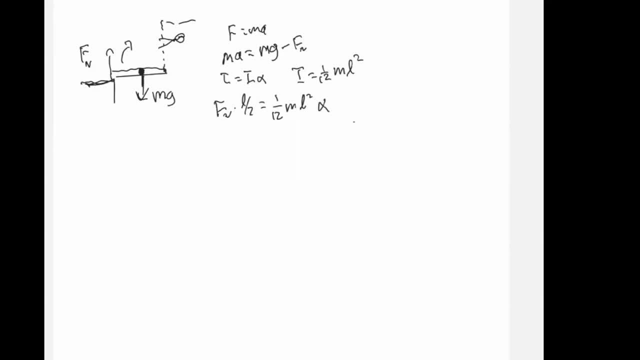 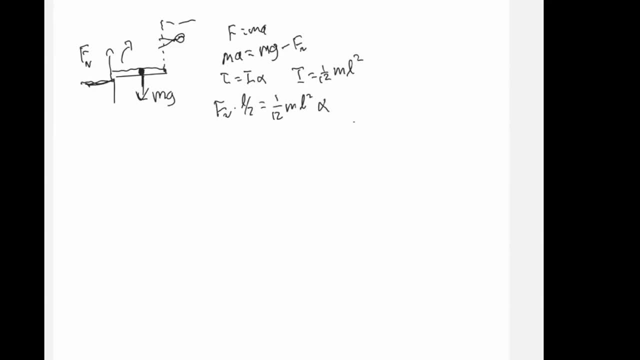 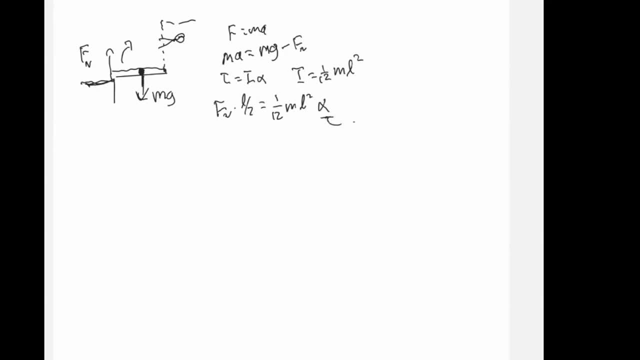 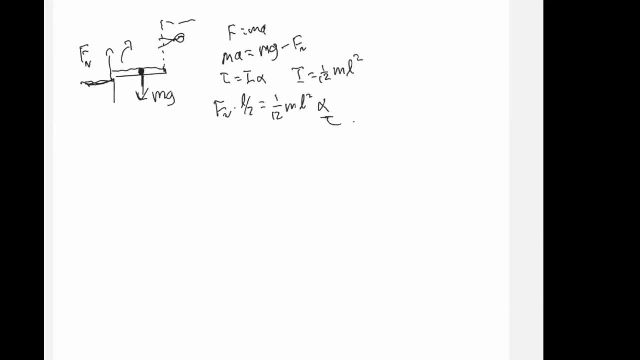 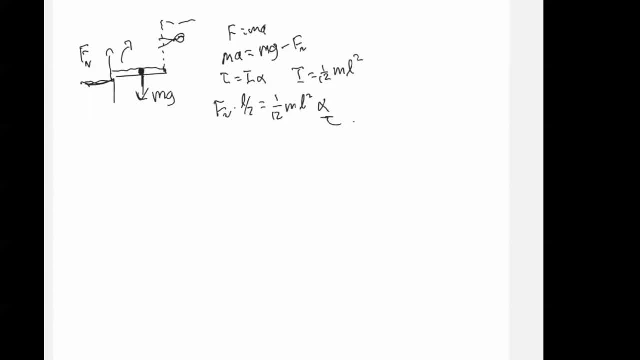 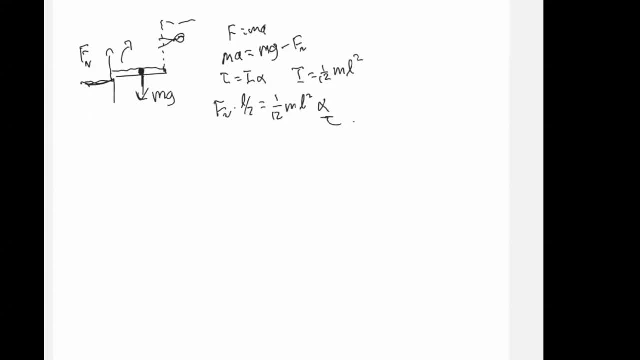 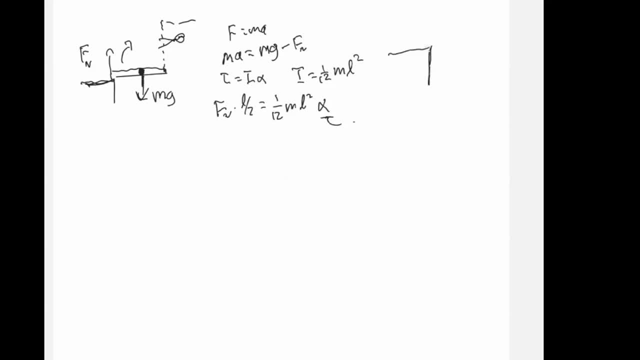 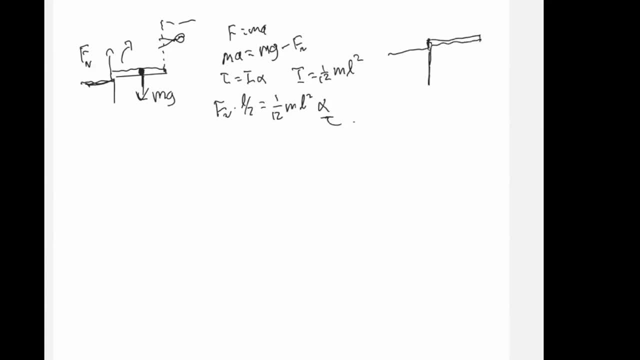 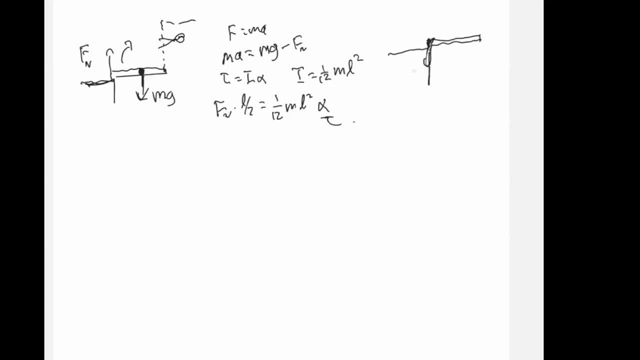 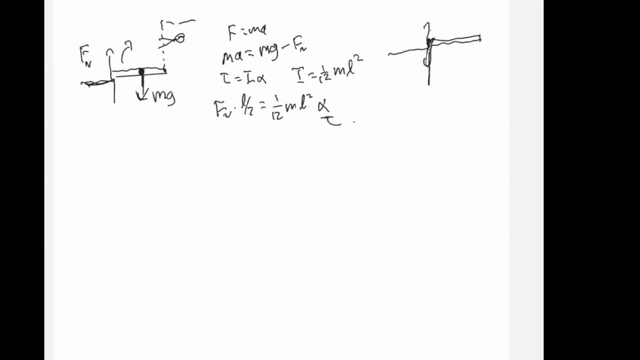 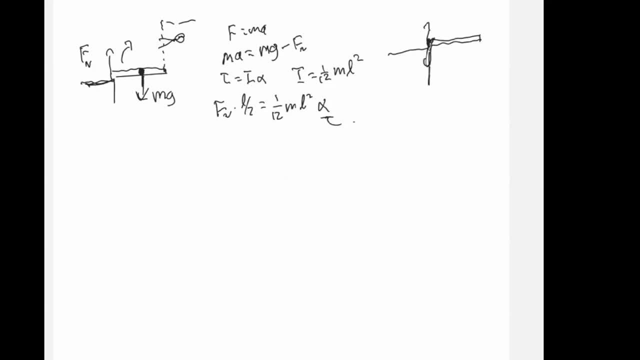 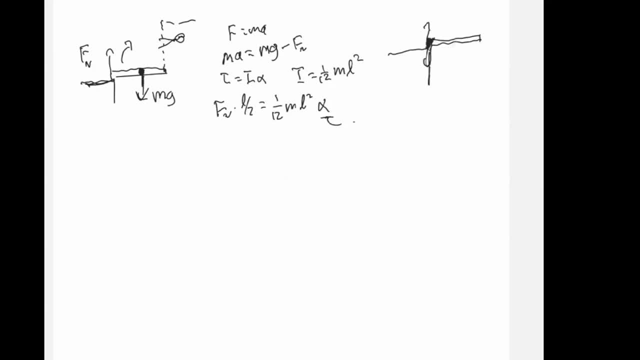 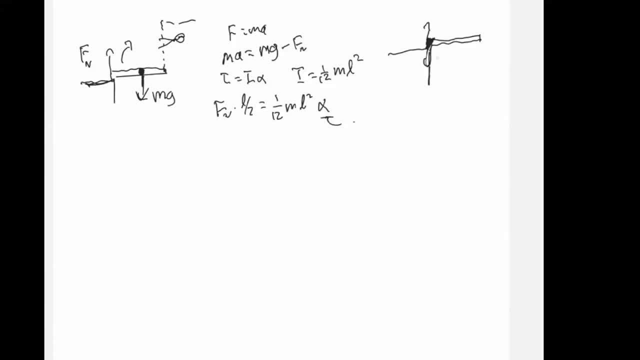 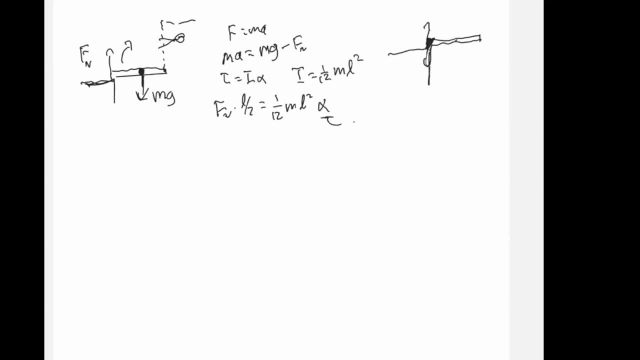 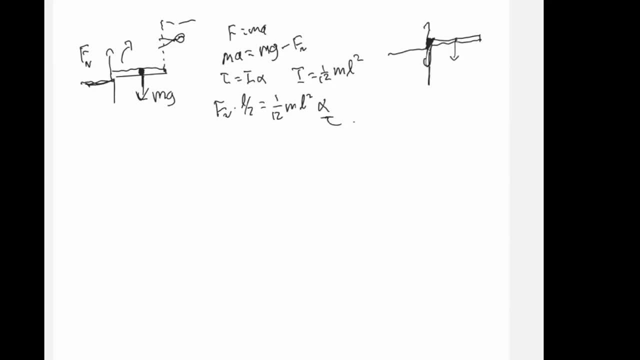 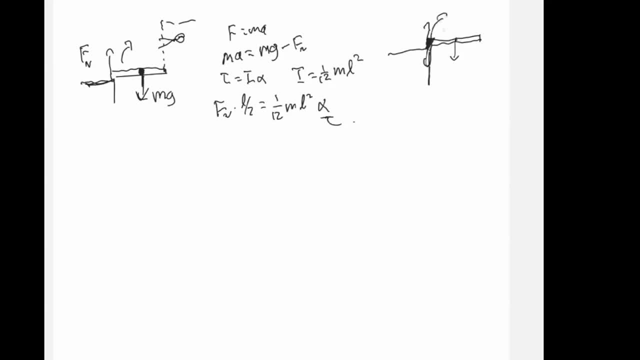 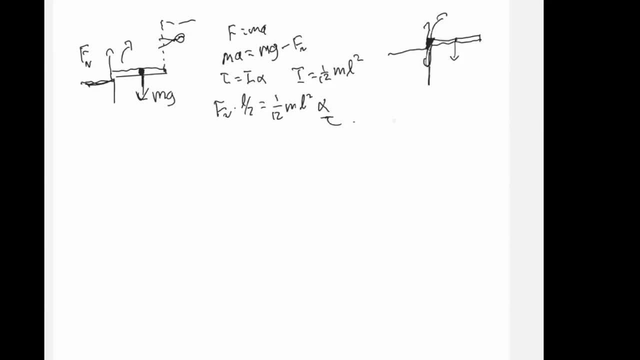 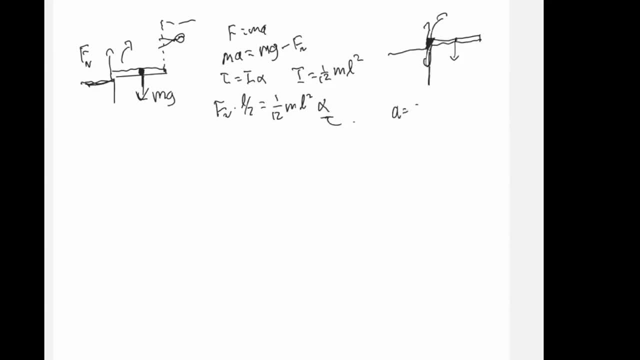 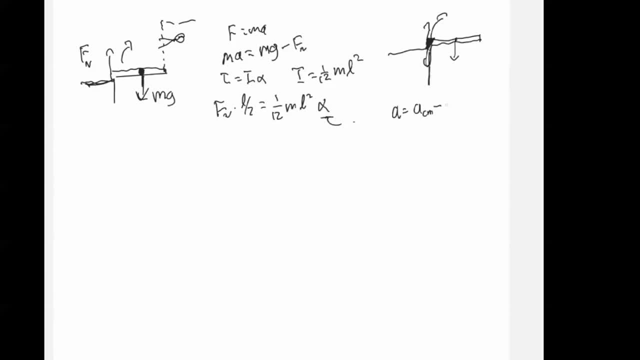 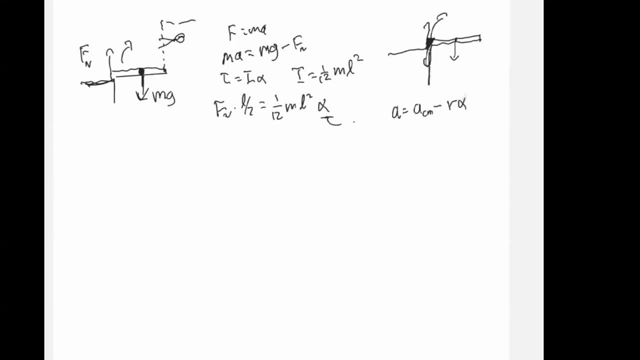 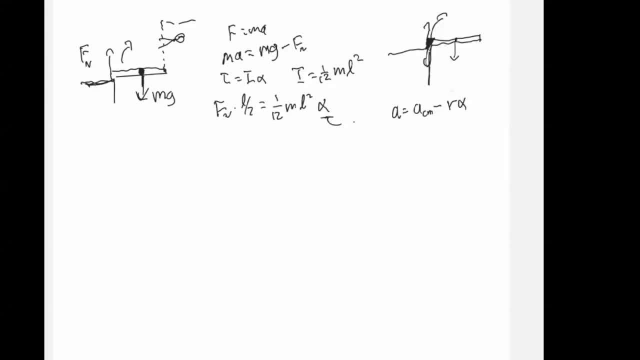 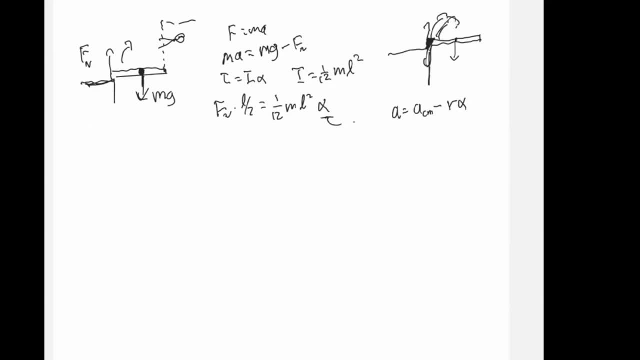 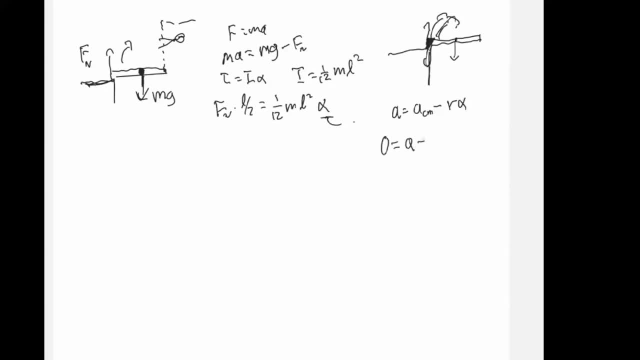 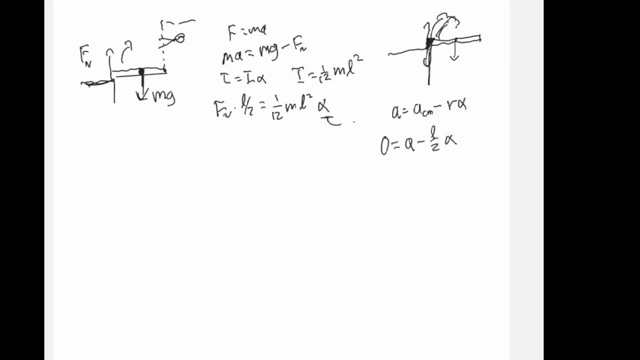 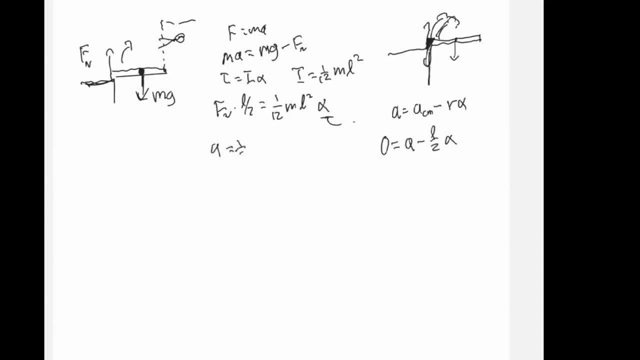 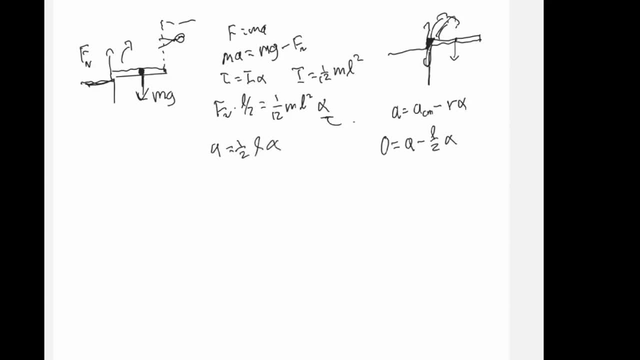 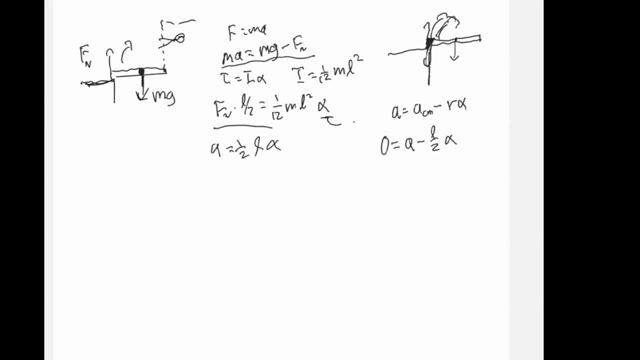 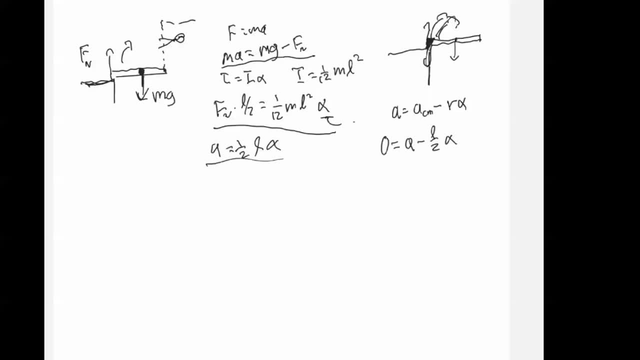 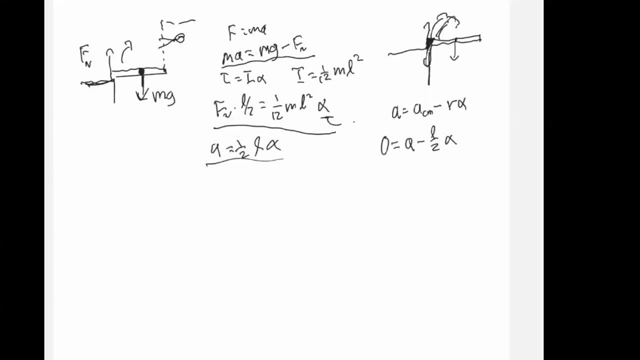 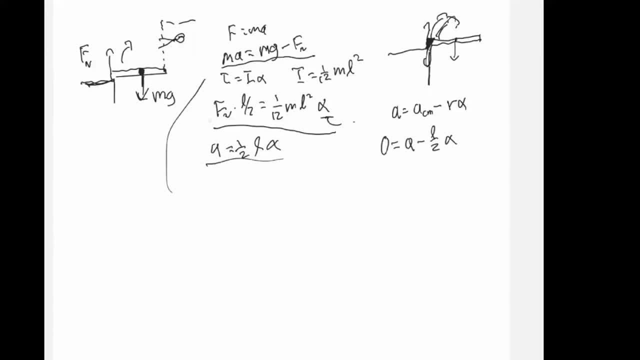 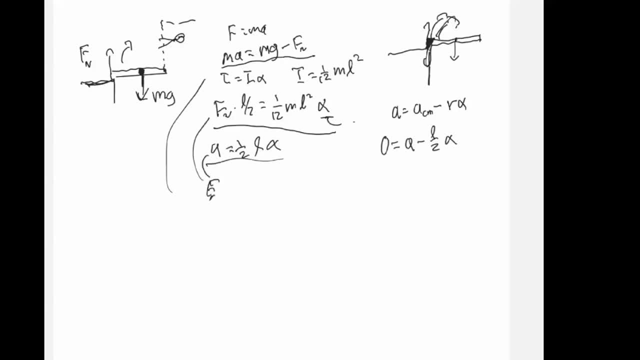 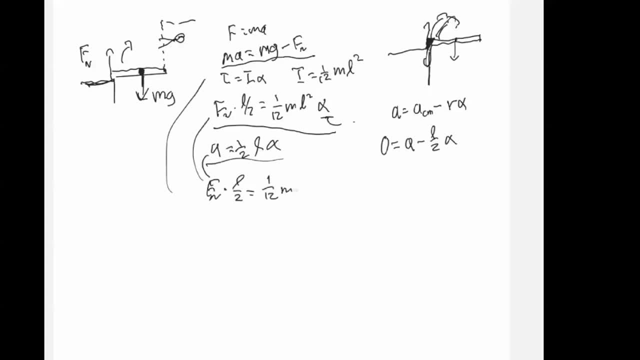 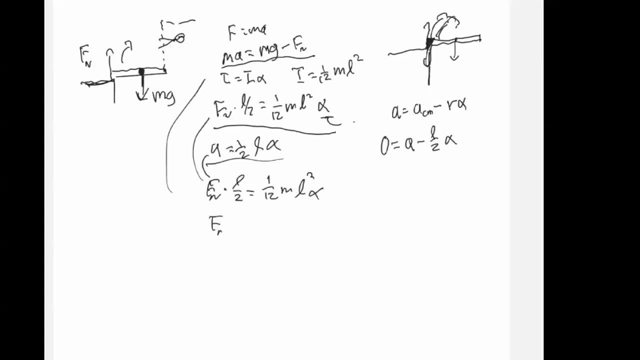 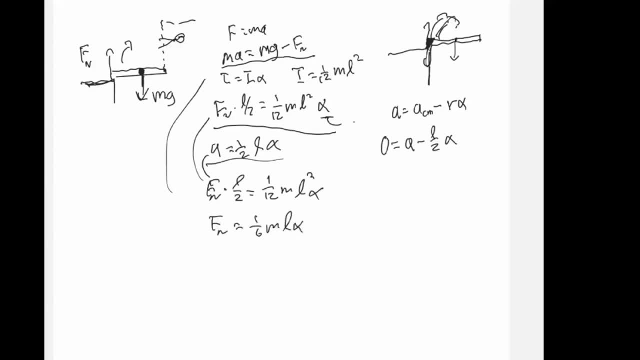 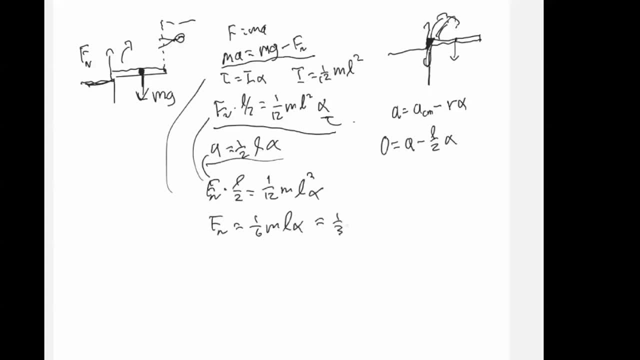 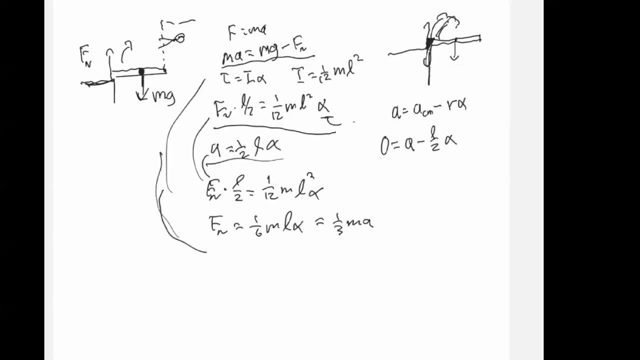 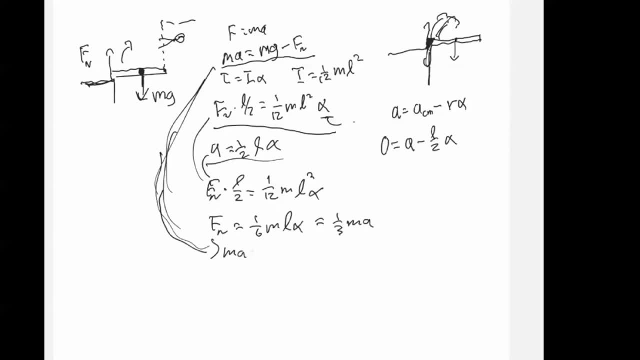 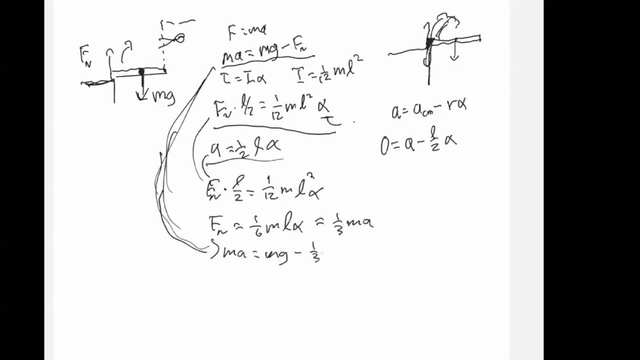 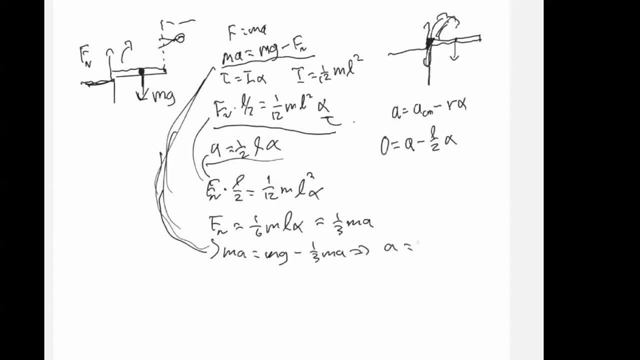 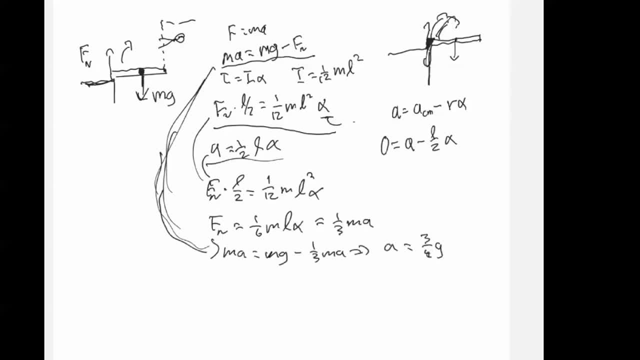 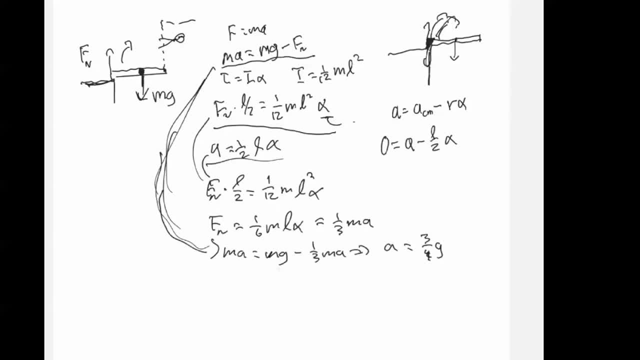 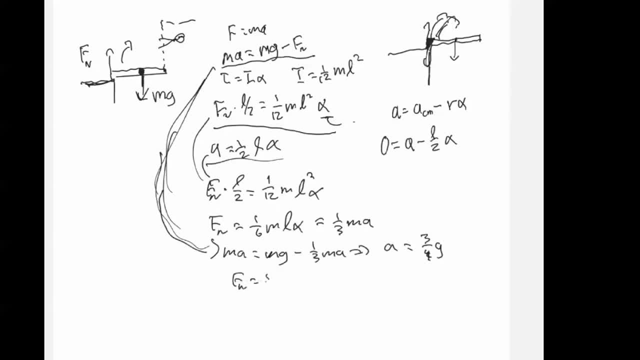 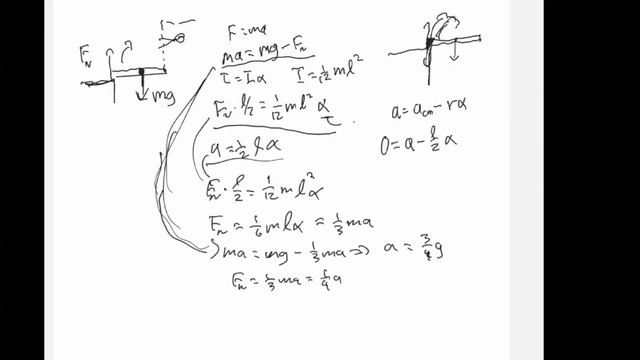 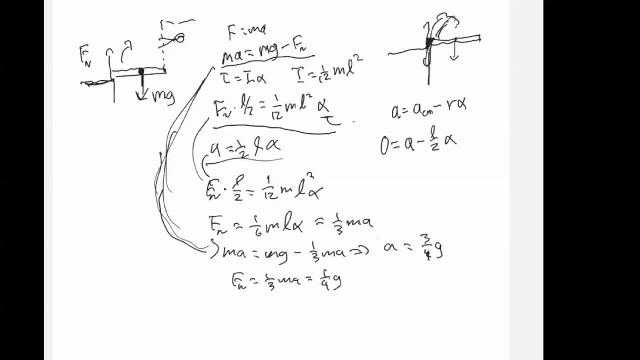 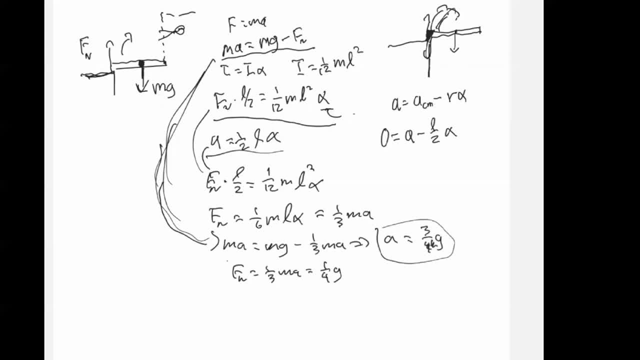 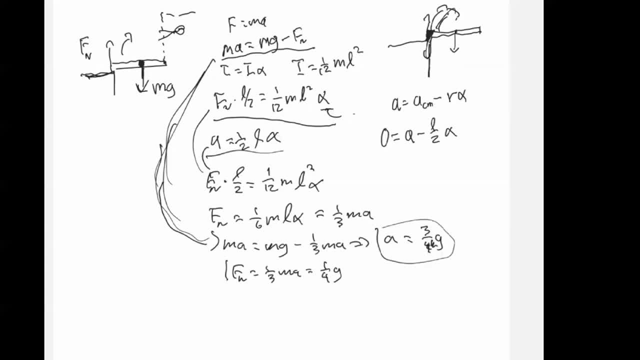 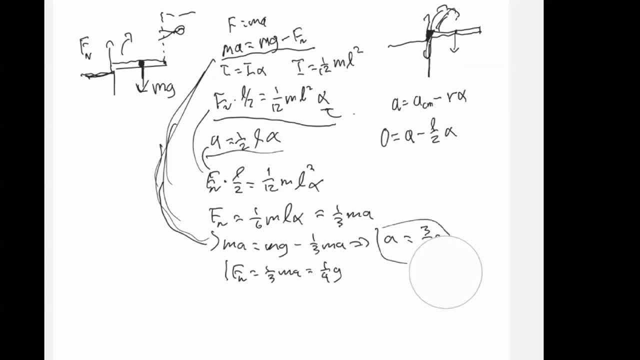 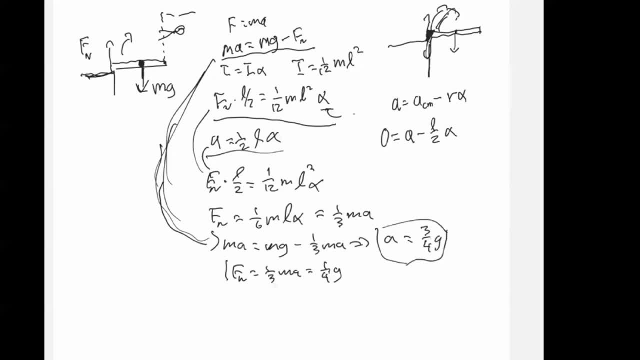 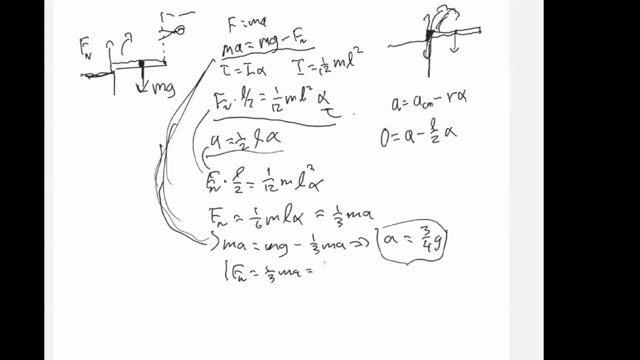 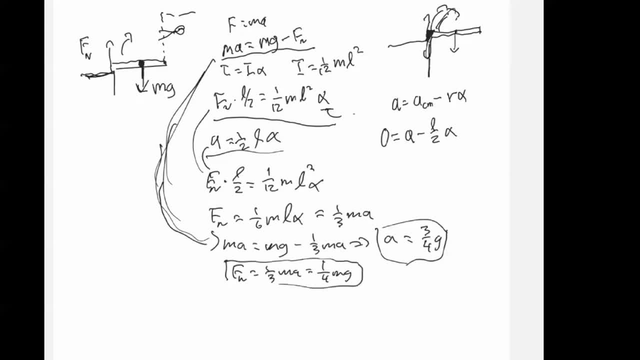 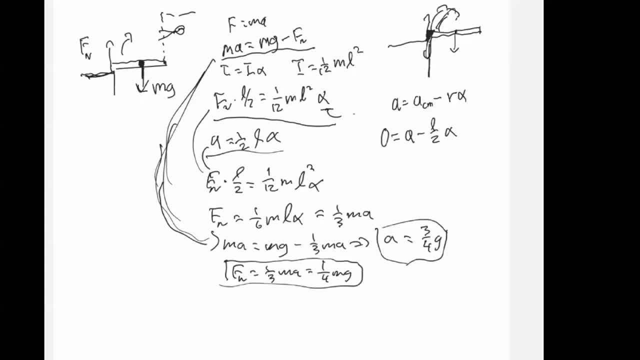 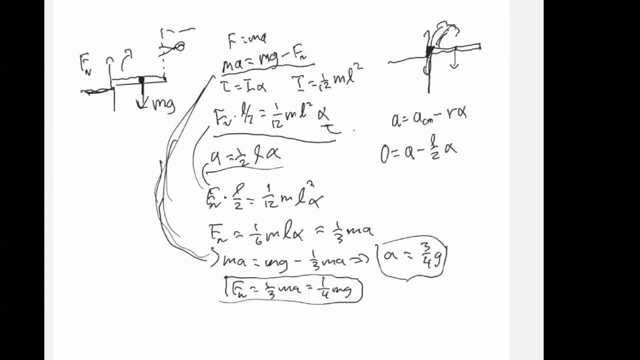 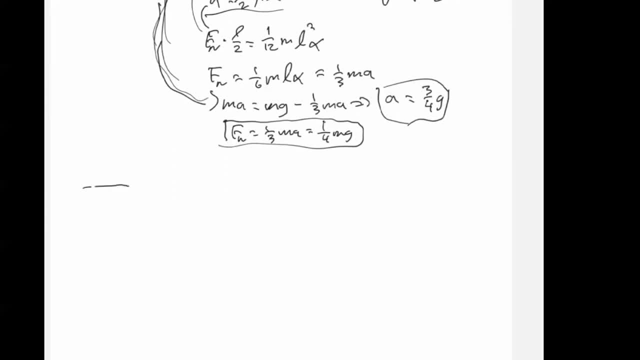 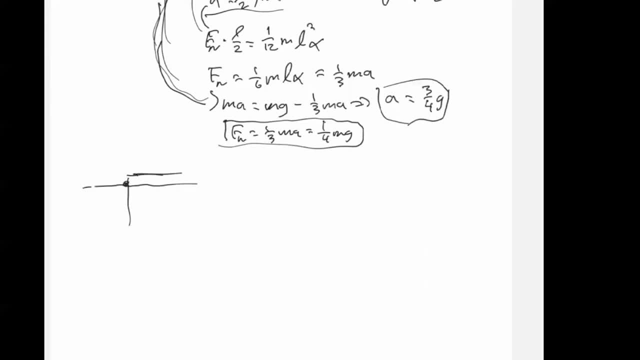 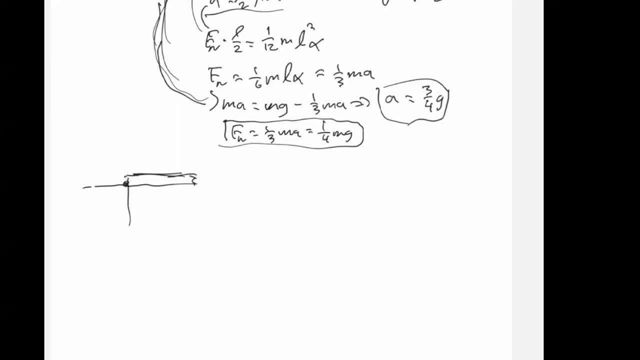 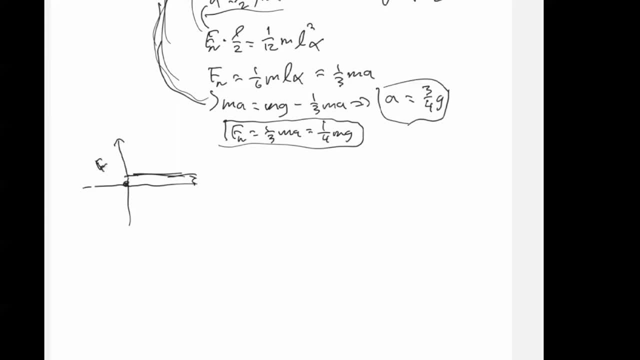 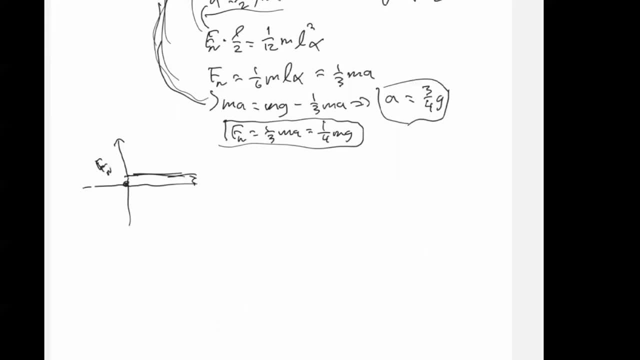 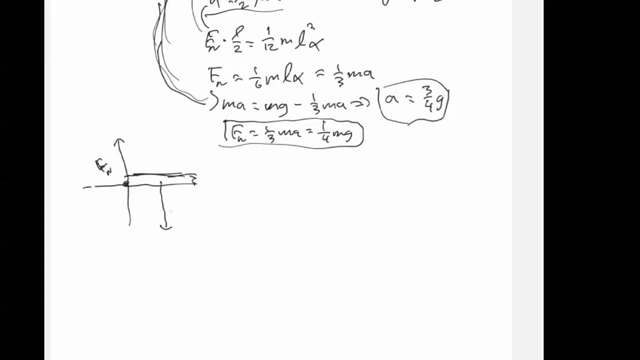 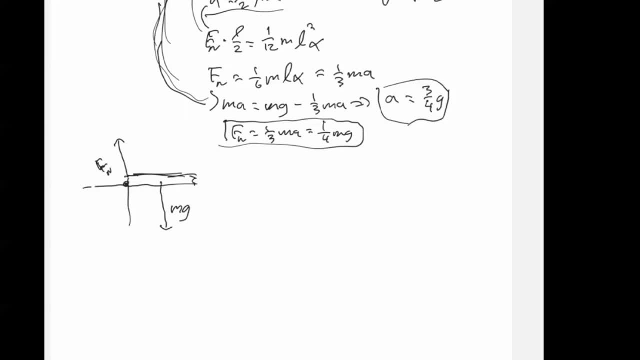 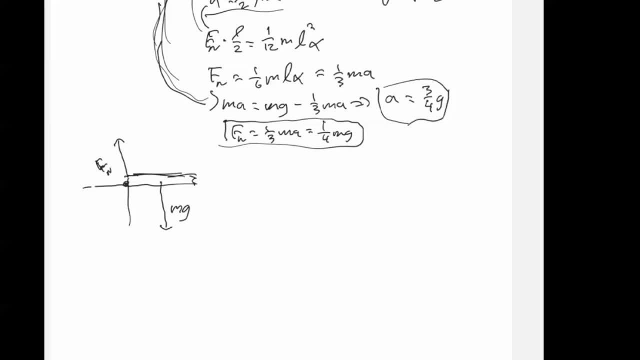 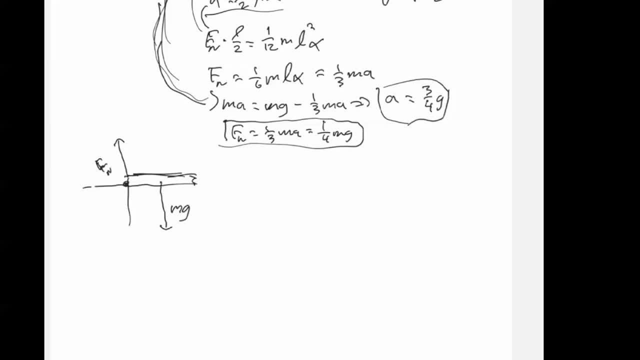 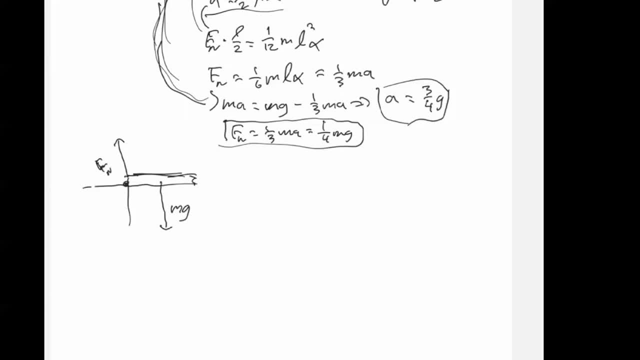 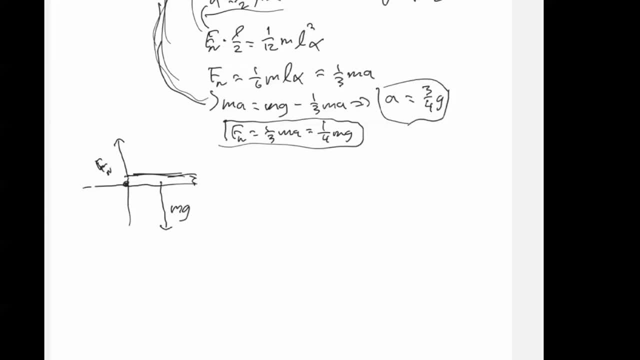 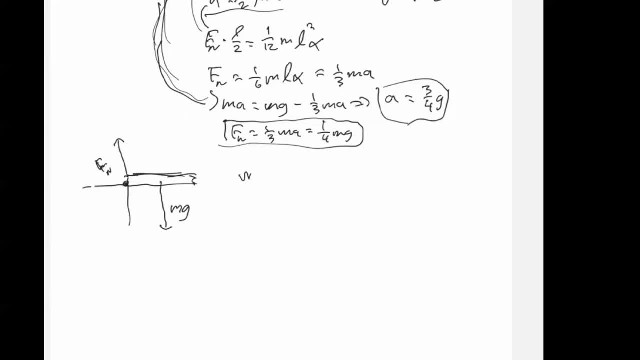 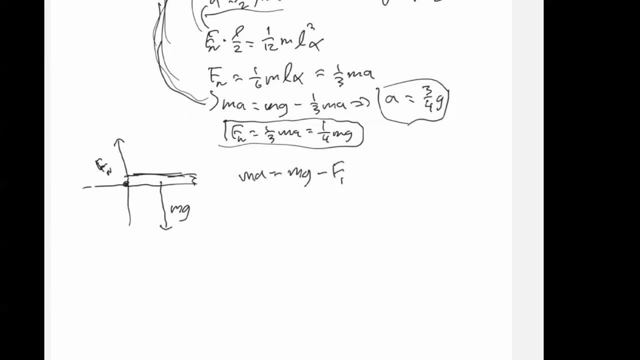 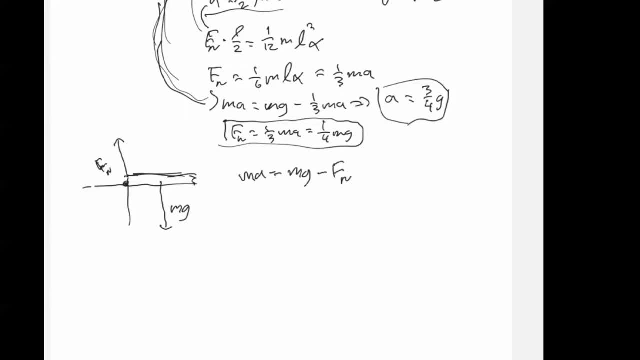 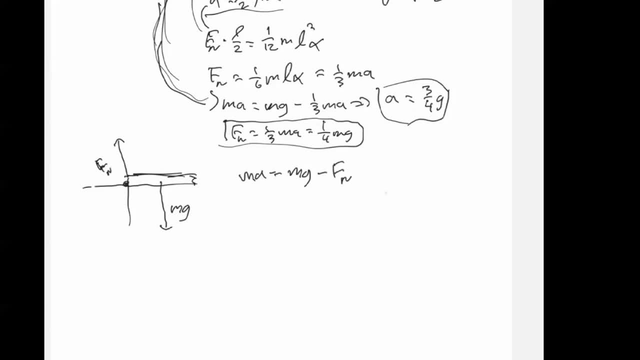 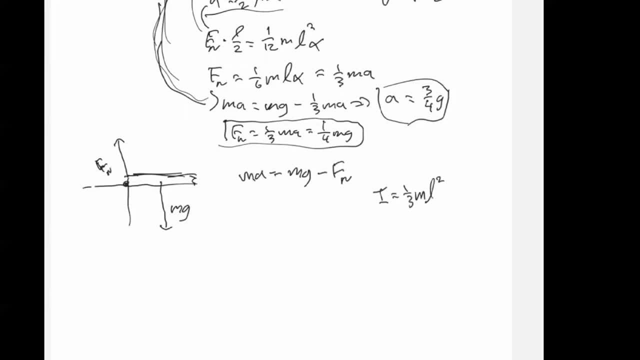 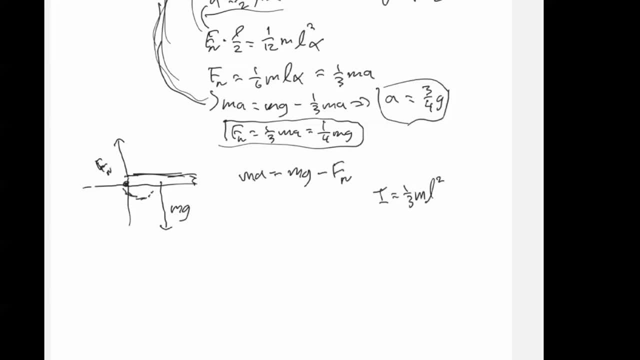 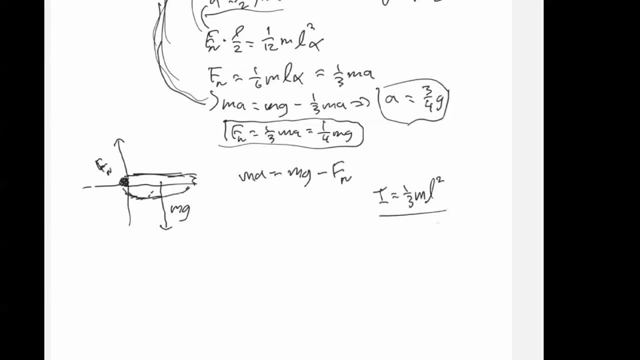 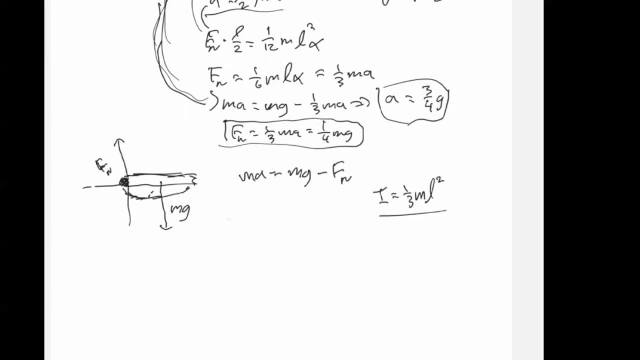 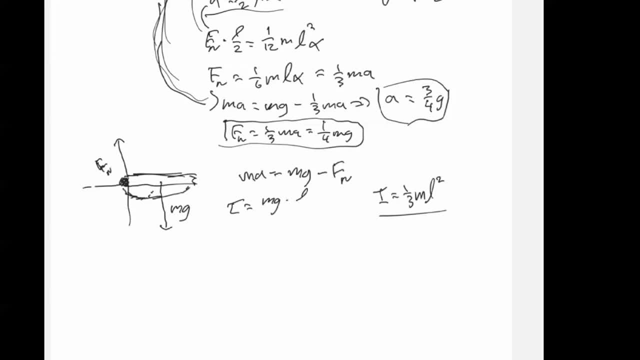 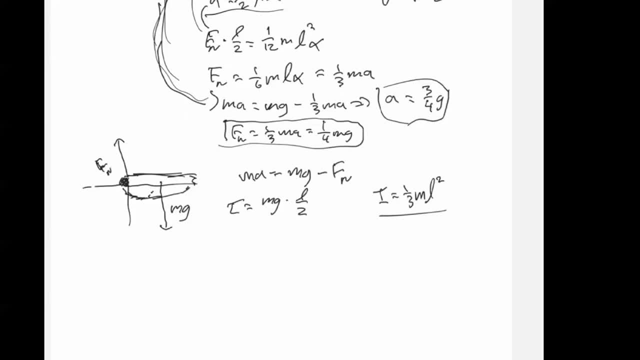 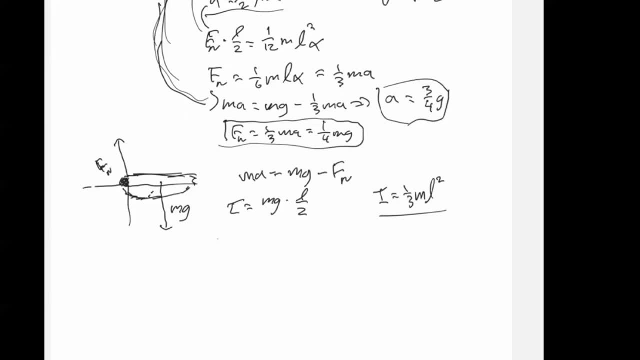 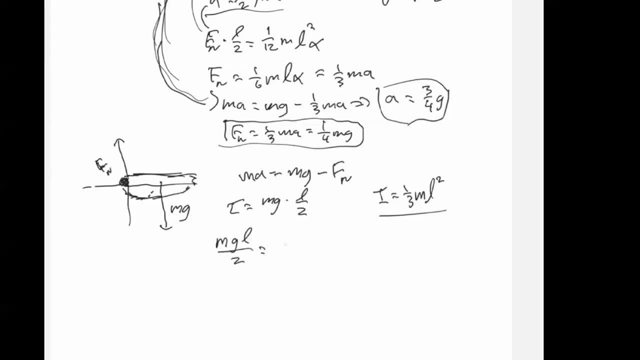 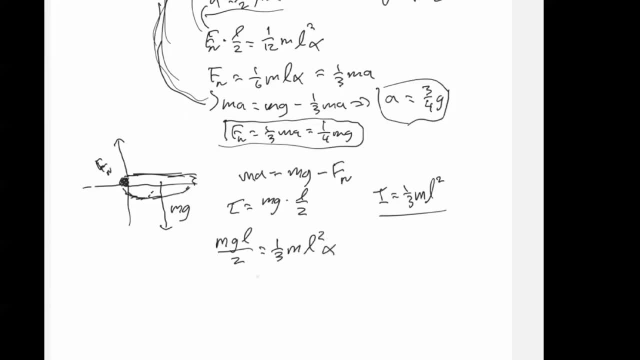 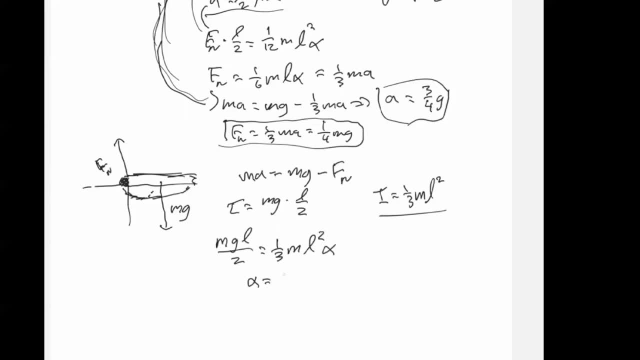 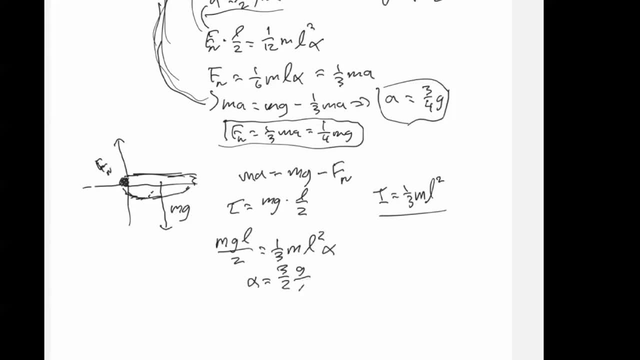 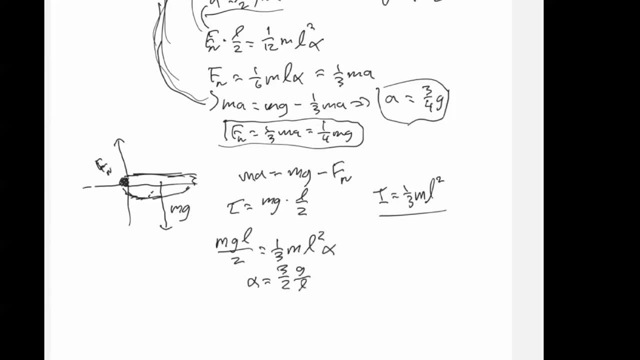 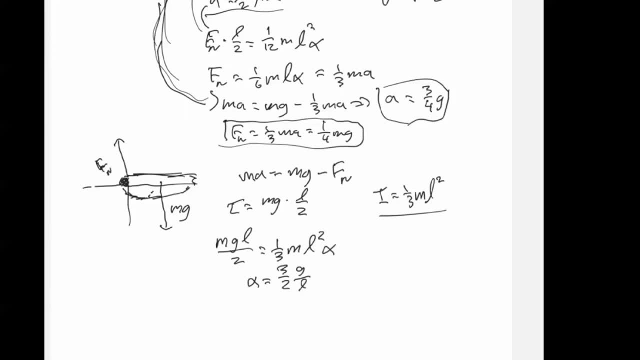 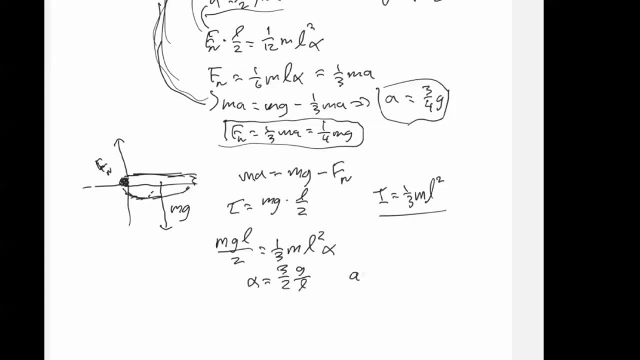 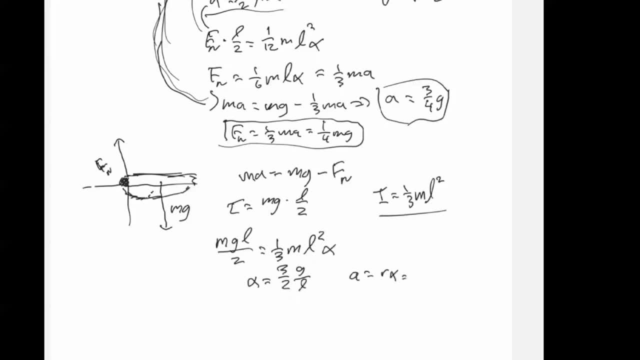 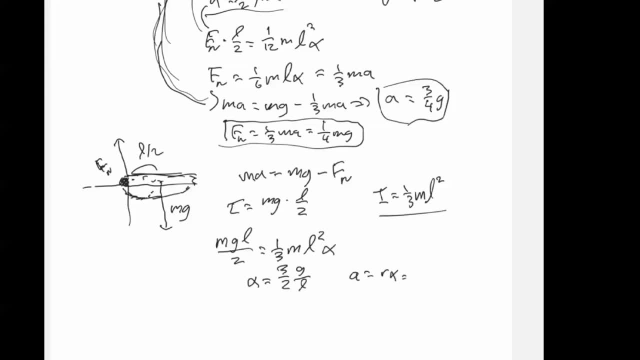 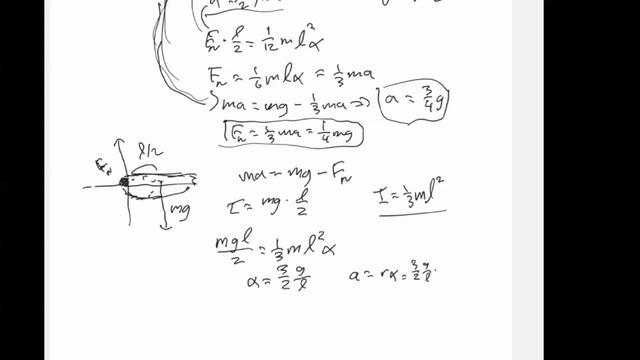 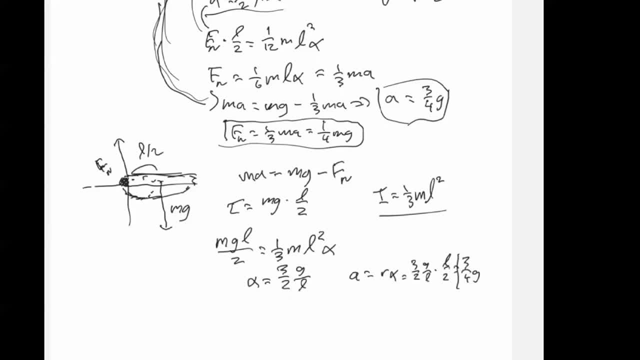 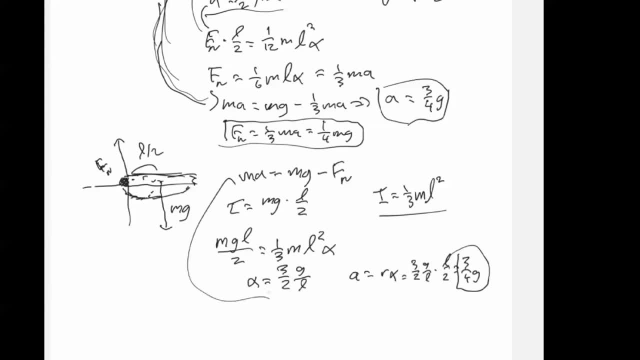 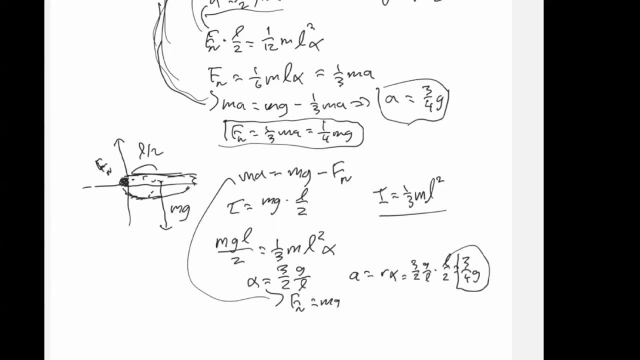 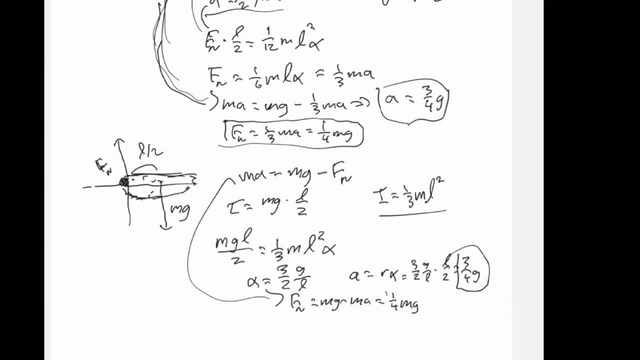 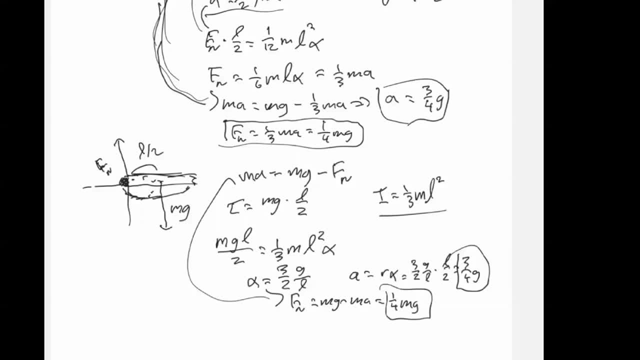 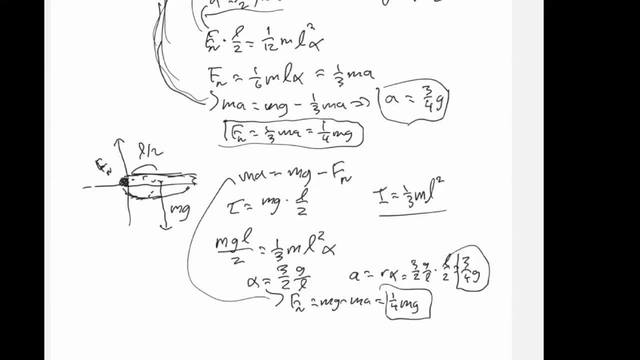 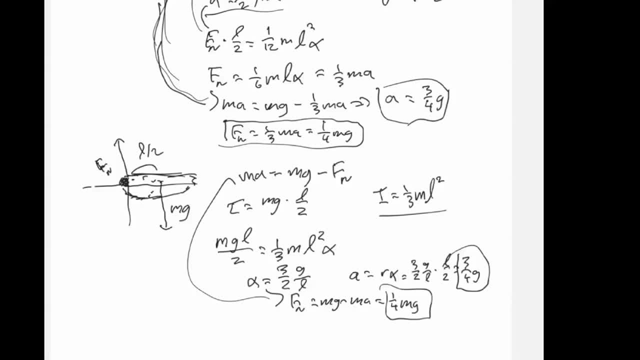 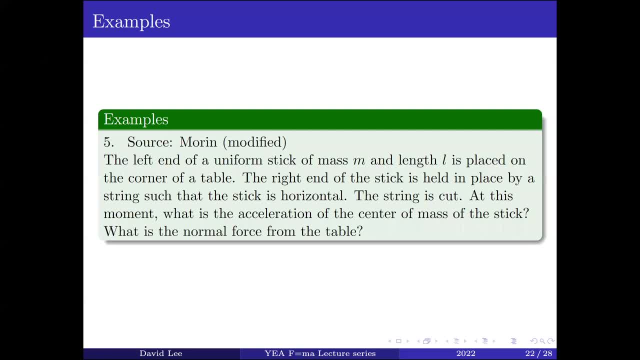 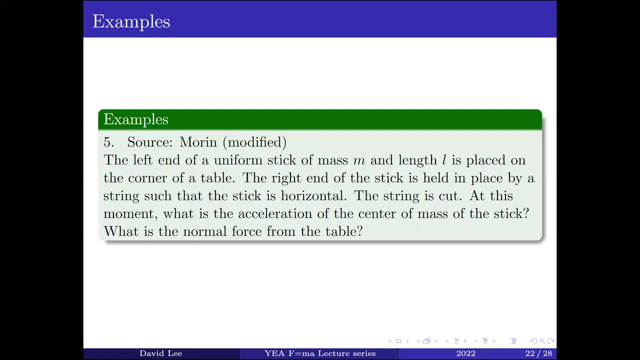 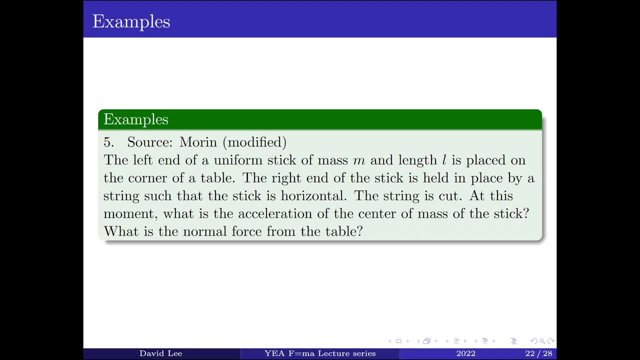 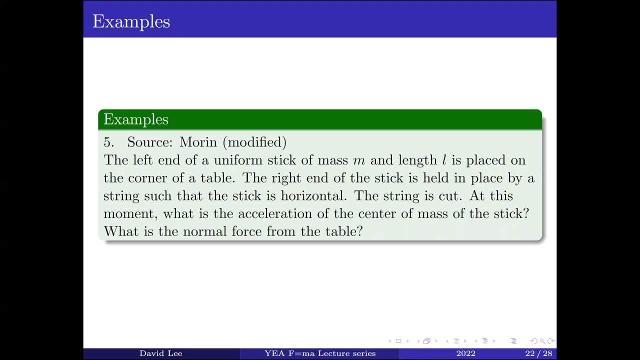 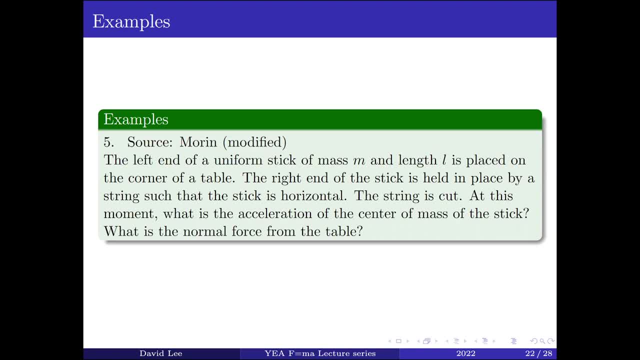 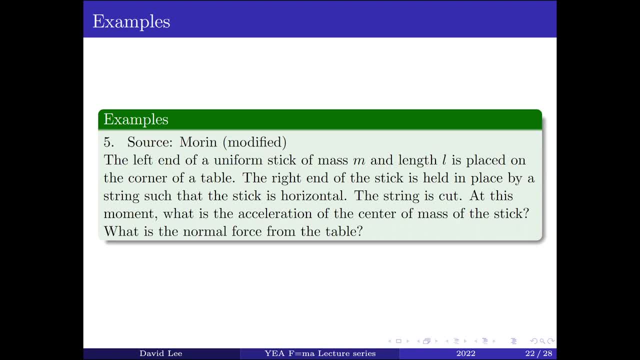 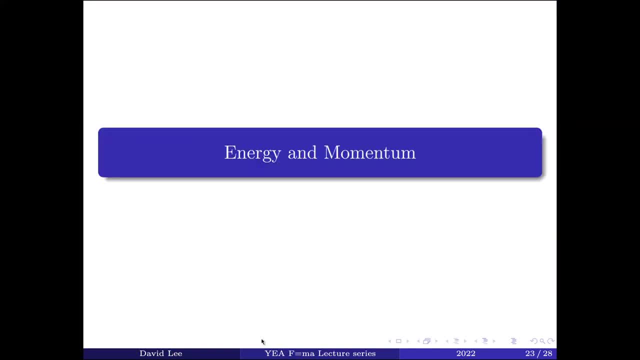 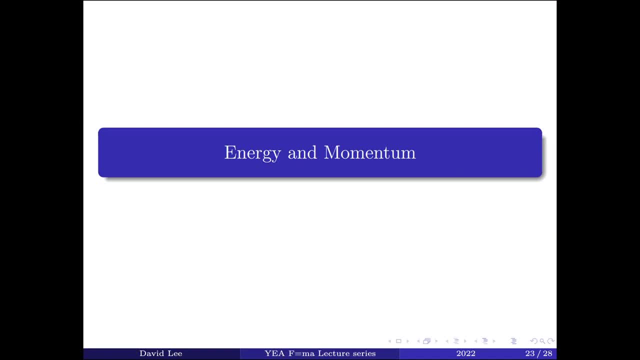 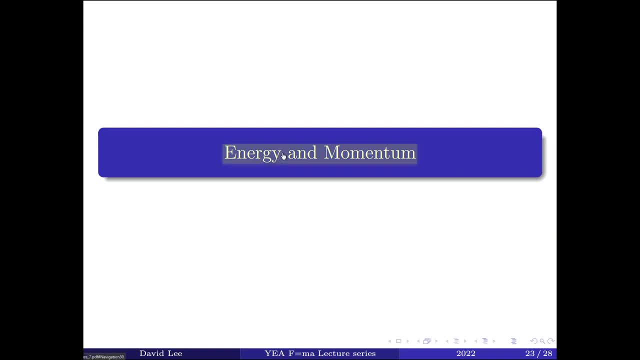 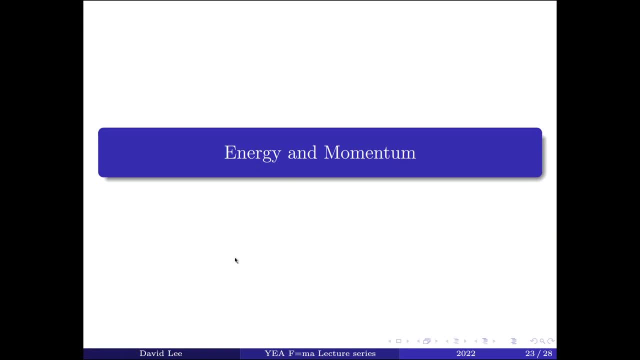 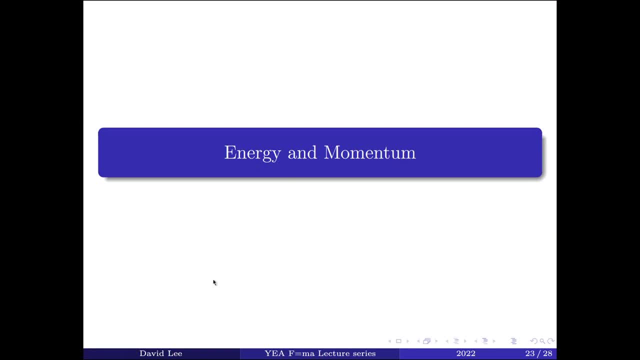 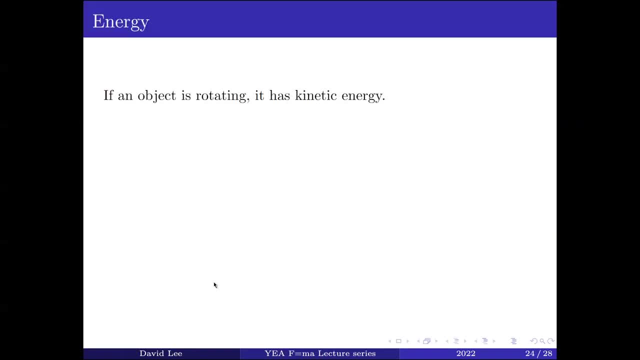 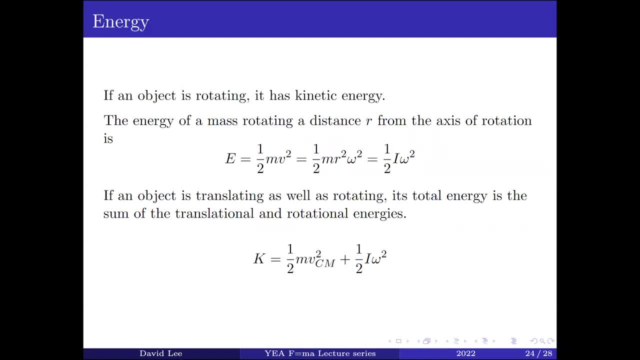 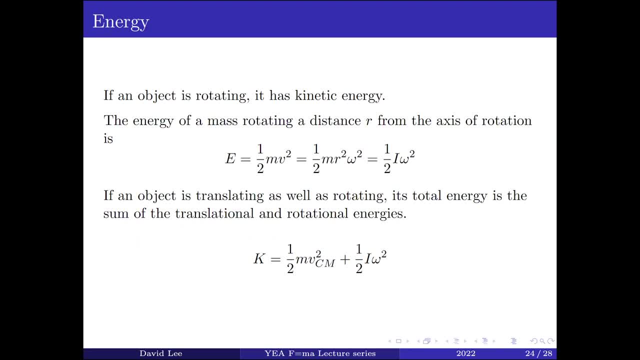 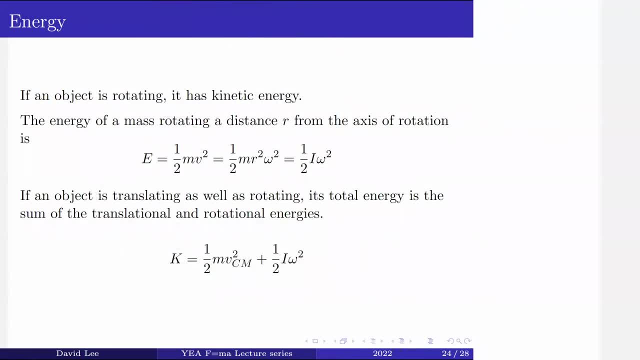 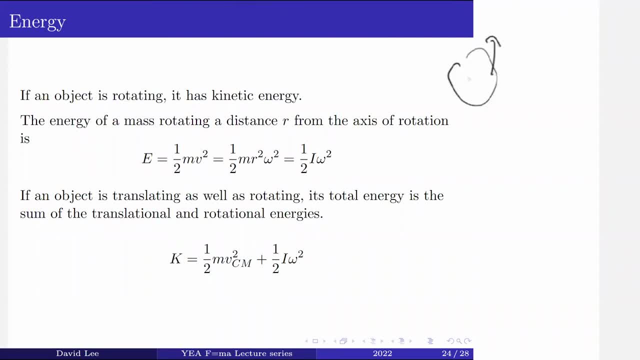 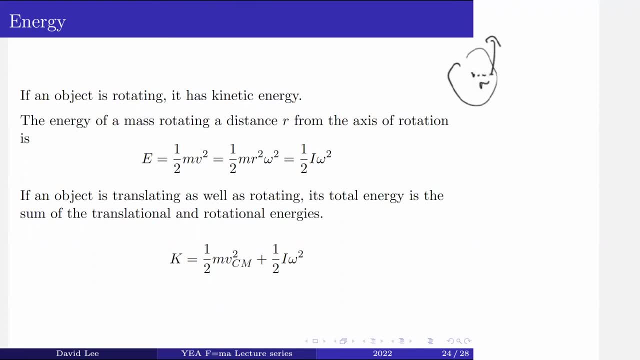 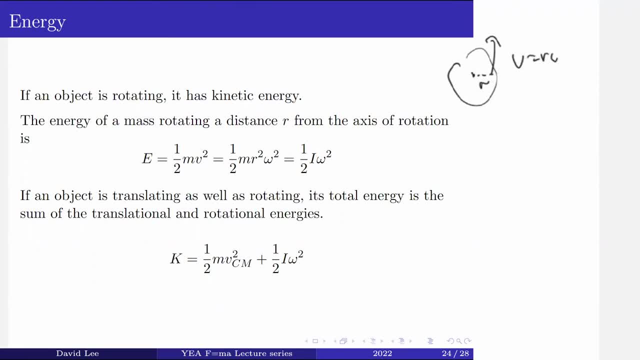 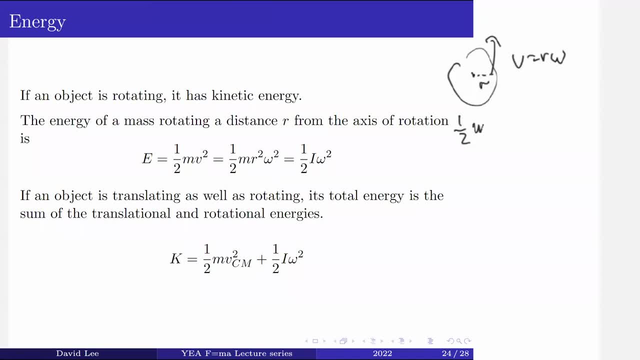 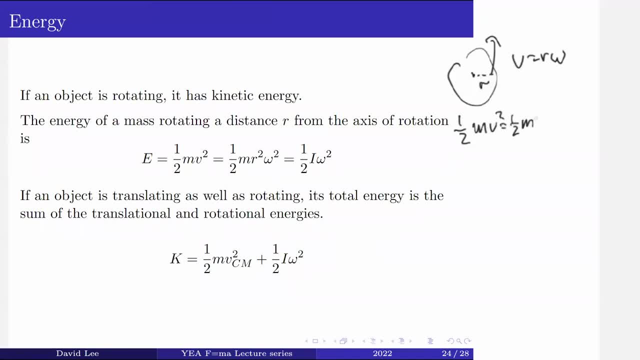 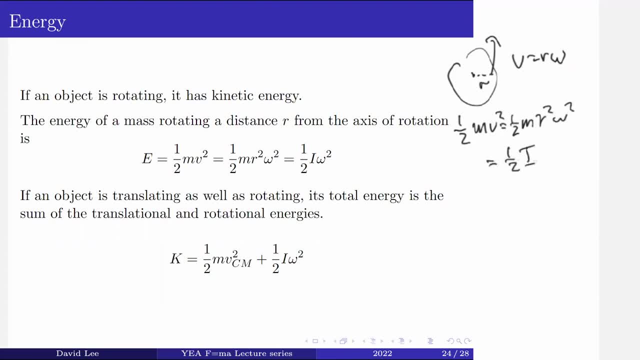 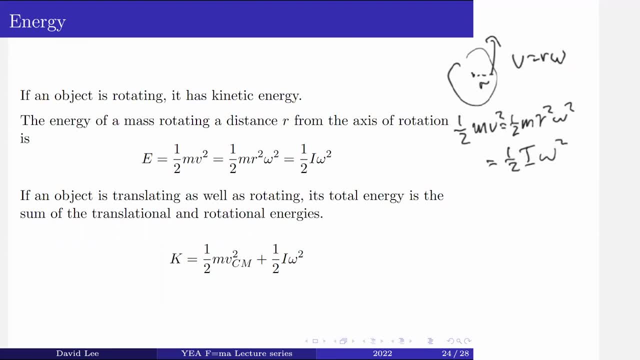 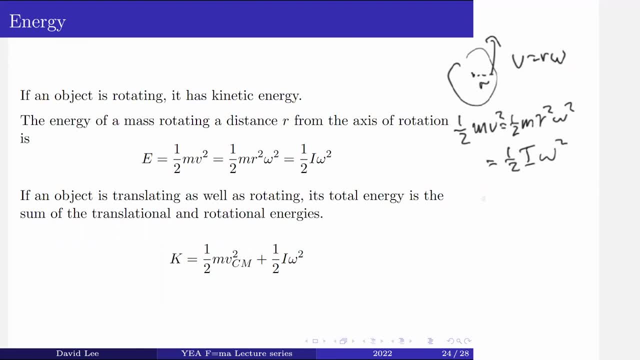 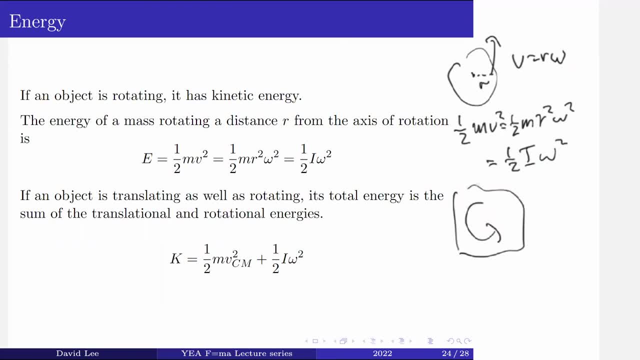 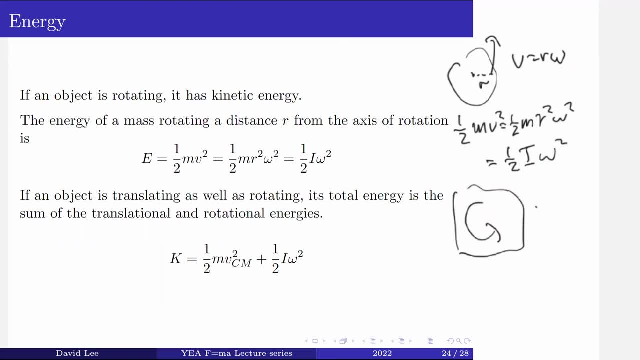 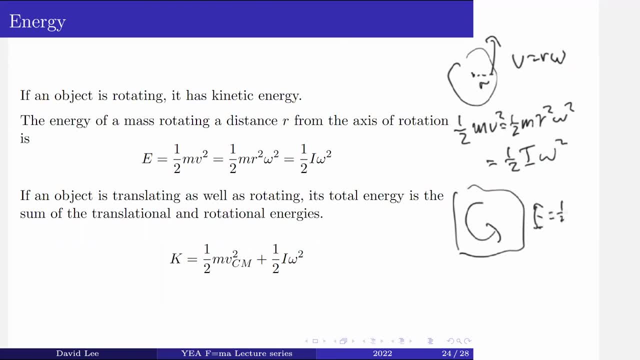 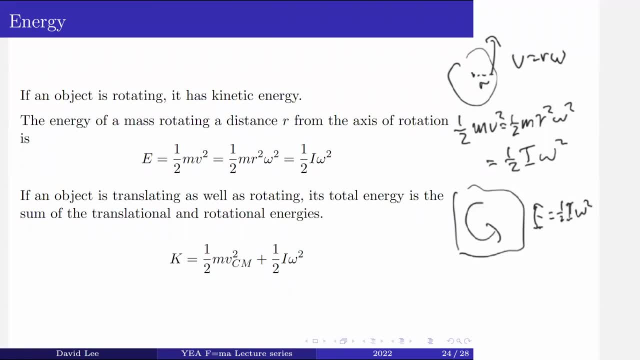 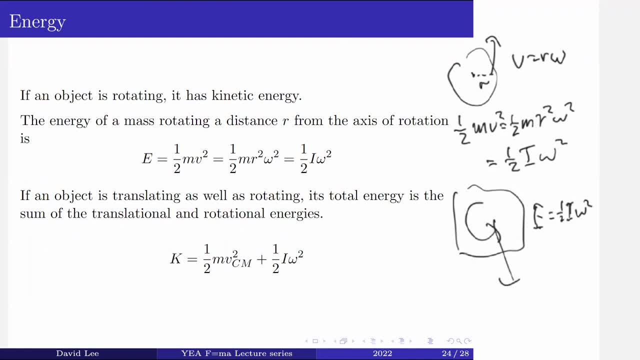 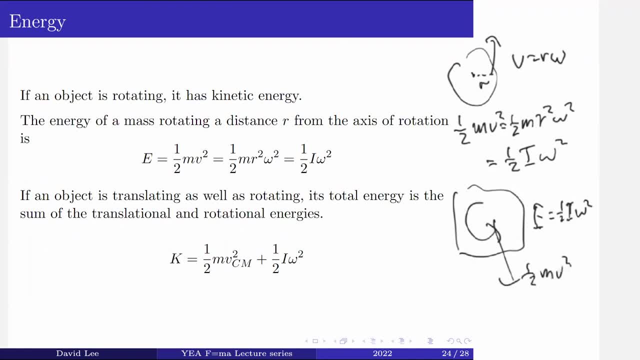 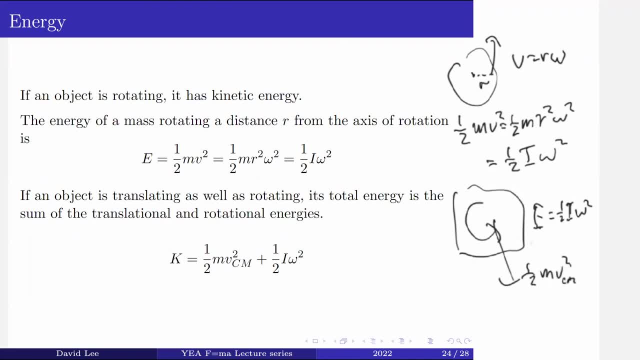 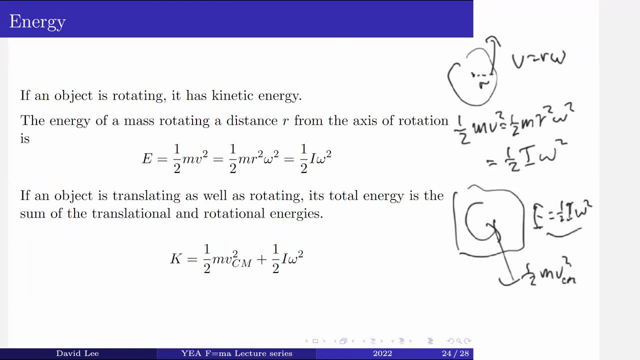 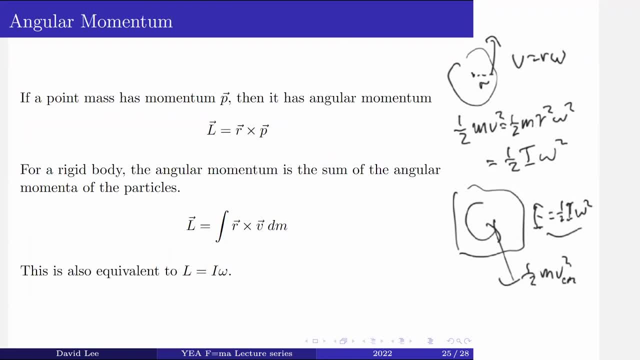 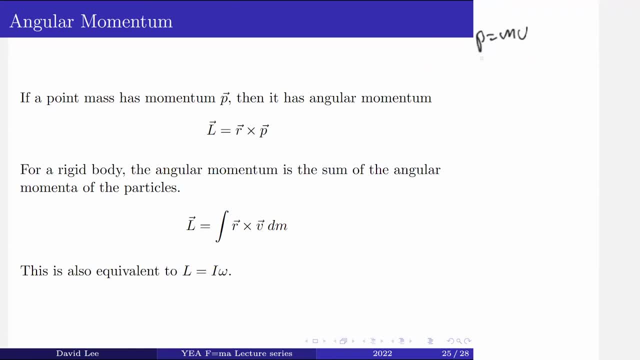 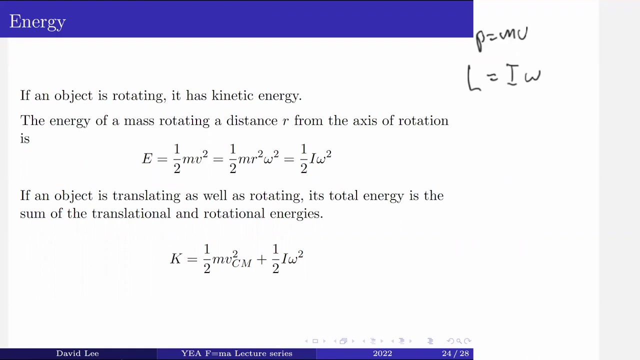 So the translational analog is angular momentum L, which is equal to I, omega. And oh, can I see slide? If you want me to go back a slide, sure, This is just talking about energy. I will review this. This is actually quite easy to remember. 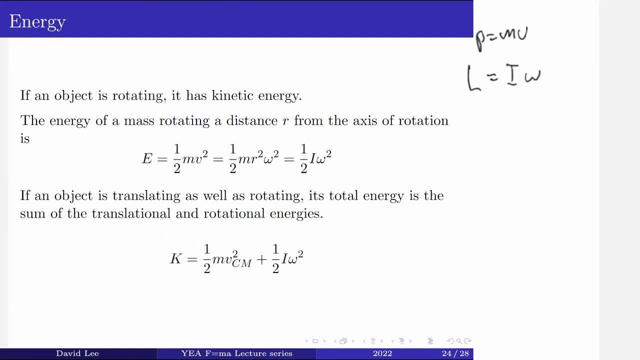 Because, if we think about it, our rotation is similar to translation: We just have to replace some variables. So we saw that X becomes theta and V becomes omega and A becomes alpha, And more recently we defined a torque which is 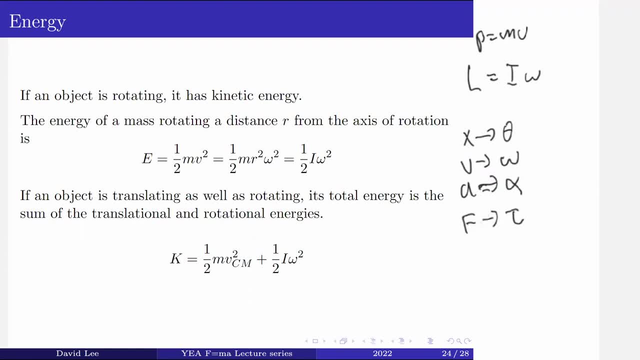 The equivalent of an angular force. And now we defined a mass that's the equivalent of normal inertial mass. This is moment of inertia. So if we see equations like F equals MA become torque equals I alpha, Or like E equals one half MV squared, 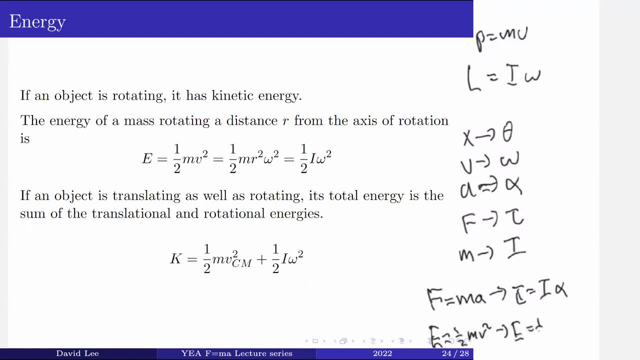 This just becomes: E equals one half I omega squared. So if you remember like what these things represent, then you can normally can easily convert from rotational formulas to or from translational formulas to rotational formulas. All right, Let's go on. 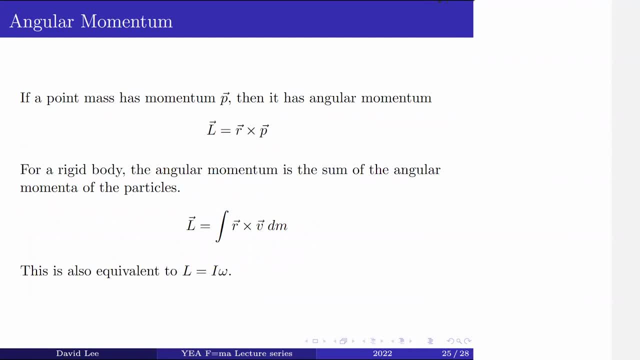 So angular momentum, if we want to define it formally, it is defined as R cross P. So P is our normal momentum And R is just our distance around some point, And this is also a cross product. So angular momentum is also a vector, but like? 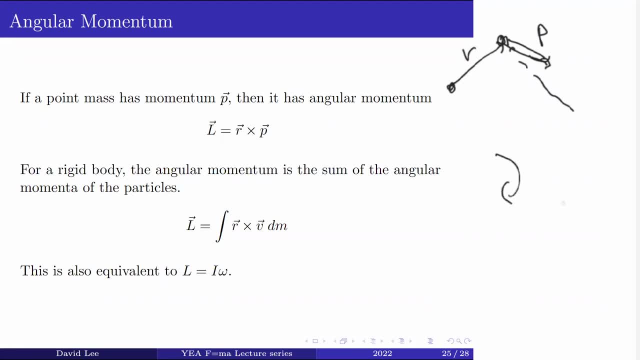 Normally it's either just clockwise or counterclockwise. So just pay attention, of this theta here You might have to multiply by Not that theta, but this theta. You might have to multiply by sine theta or something like that. But yeah, angular momentum is. 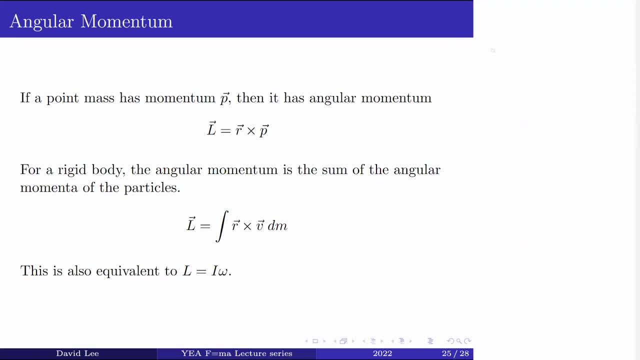 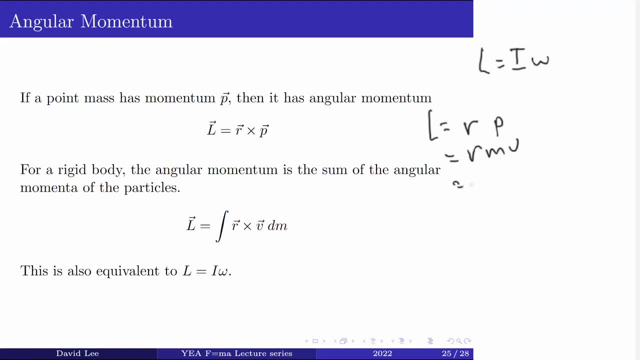 So this is RMV, But V is also R omega Or MR squared omega, And and then, yeah, this is just i omega and you can do cool things with it's also. torque is also d l d t and this is basically the same. 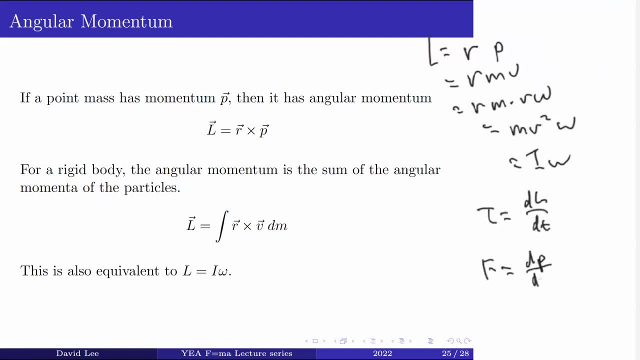 thing as our force equals dp dt. so this is the newton's second law for rotation and just like normal momentum, perhaps the most important thing is that if we have a system of particles and they interact, whatever, normally what happens is that each interaction, well, one one particle exerts a force on the other particle, but by newton's third law that 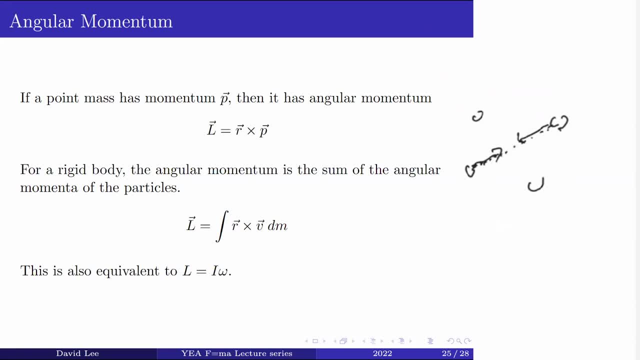 other particle exerts an equal and opposite reaction force. so if we consider the torques, well, the torques are going to be the same with respect to some um reference point, because the forces are the same and also the radius should be like the same, yeah, so 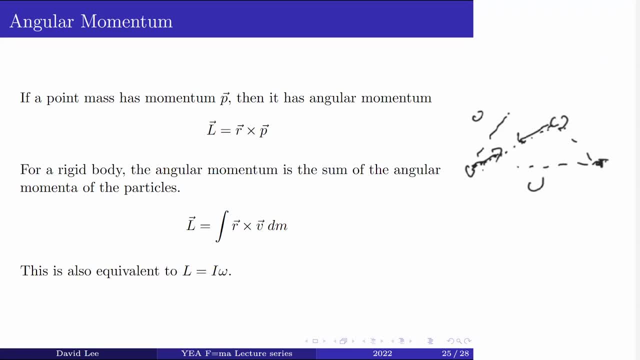 these will end up canceling out and we'll be able to have the equivalent of conservation of momentum for rotation, which is basically just the conservation of angular momentum um. so when there's no, when there are no exceptions of external torques, angular momentum will be µ. 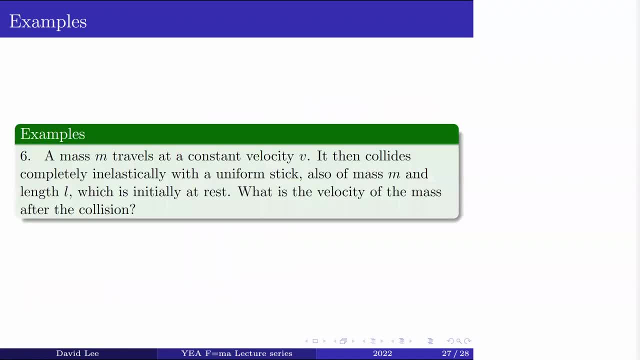 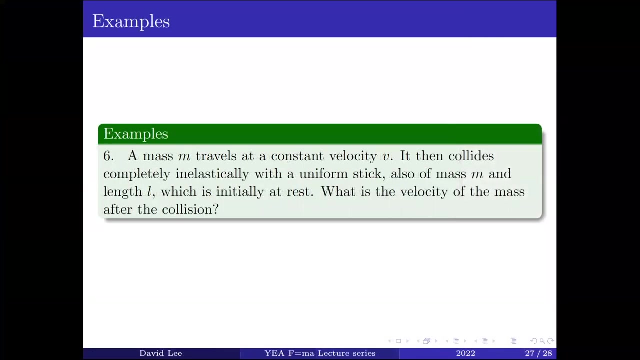 CAD AG DEV. the last problem: it is quite a tricky problem actually add event. i'll give you a few minutes to think about what you want to call what you hope is going to happen in the future. think about this one, Thank you, Thank you. 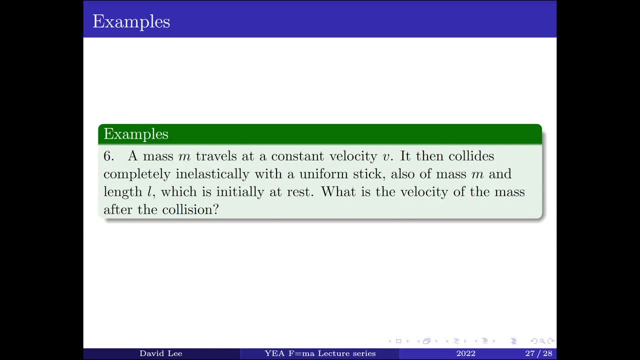 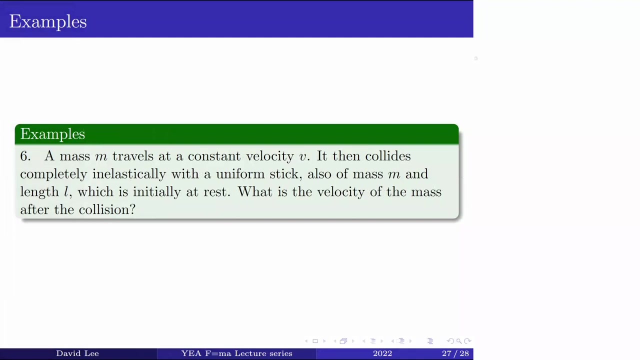 Thank you. We have a mass m here. Initially it's traveling at a velocity of v and it will collide with the end of the stick here and stick to it, and, yeah, the stick will move, but it will also rotate, and so we want the velocity of this end. 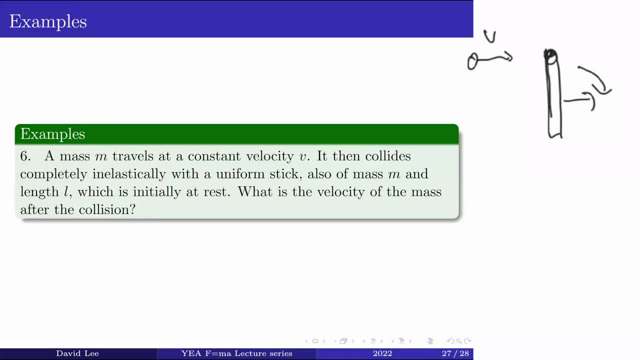 right after the collision. So we're going to see if we can get the velocity of this end right after the collision. So we're going to see if we can get the velocity of this end right after the collision. you, you, all right, it's almost 3: 30, so let me, let me start talking about this problem. 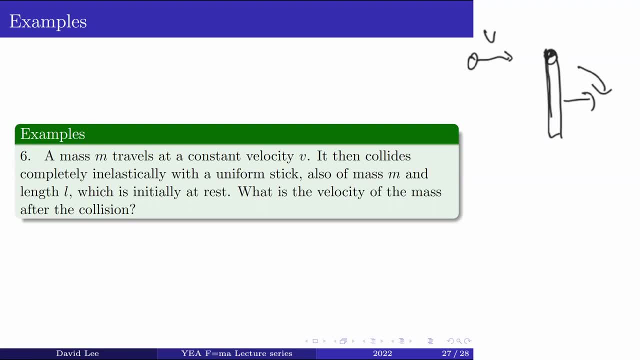 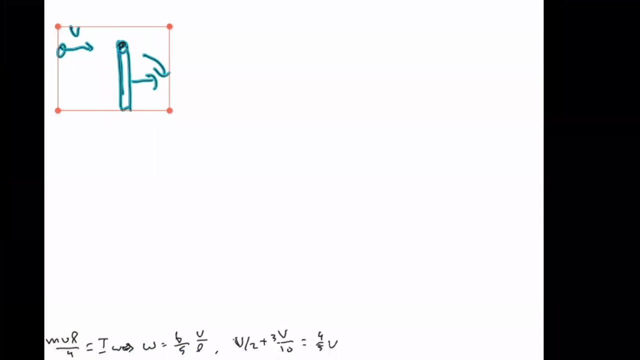 um, okay, so let me move my diagram over. oops, um, here i kind of gave away some of my work. um, so how will we approach this problem? the first step is to choose a good reference point, and here i'm just going to choose the center of mass, because the center of mass it's going to. 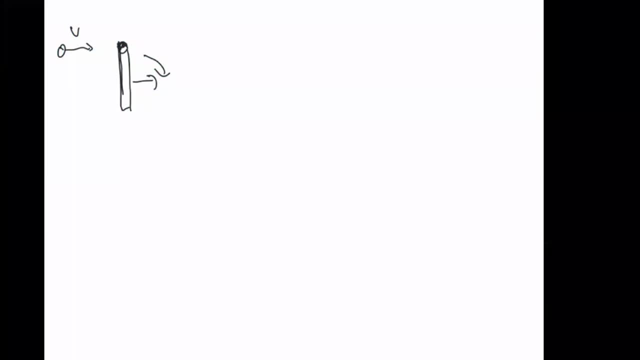 rotate around the center of mass after the collision, right, so it's going to be very nice to choose that as a reference point. so, first of all, we have: uh, after, right, after the collision, what's the center of mass going to be? it's going to be right here. 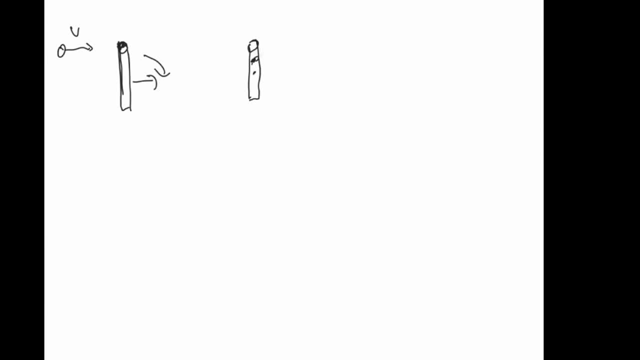 and so let's calculate um, let's calculate the moment of inertia first around this new center of mass. so for the stick we can use the parallel axis theorem and get that i equals 1, 12 ml squared plus this distance. here is l over 4. 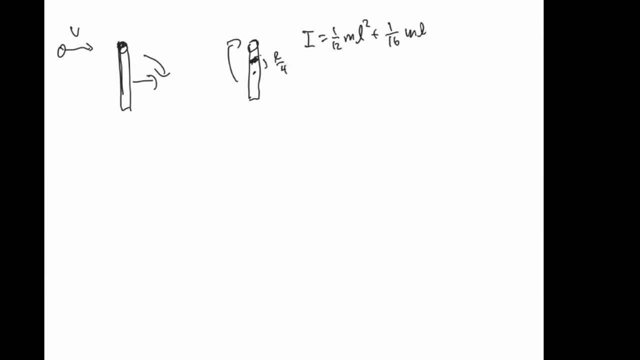 so plus 1, 16 ml squared, and then we also have to add on another 1, 16 ml squared, because this mass is also here. it's the distance l over 4 as well. so after we add this all up, we should get 5. 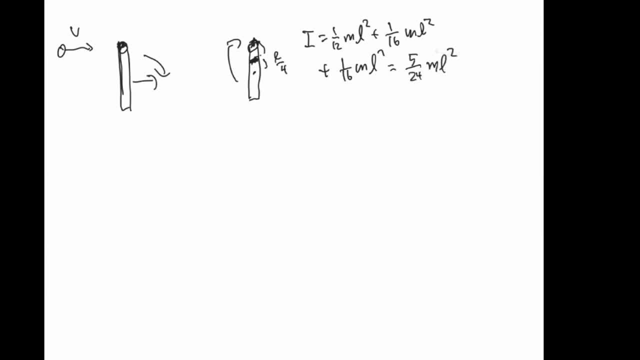 over 24 ml squared. that's our moment of inertia. and okay, we have two equations, i think. first one is conservation of linear momentum. so what that says is that mv, mf, That's our initial momentum. It's going to be 2m times our v final. This is the final velocity of 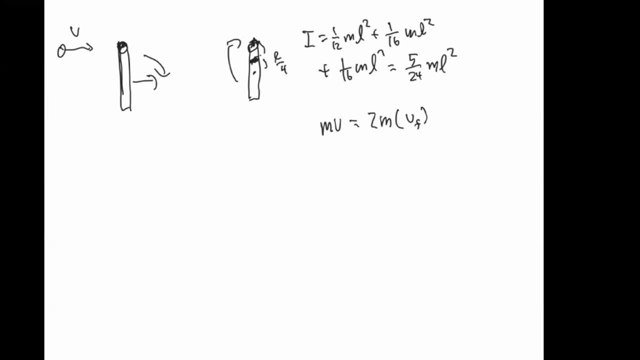 the center of mass, which should move at a constant velocity after the collision. So we'll get that v final is just v over 2.. All right, now we have a conservation of angular momentum, So what's its initial angular momentum? Well, to calculate that we have to use the definition L equals r, cross p. So 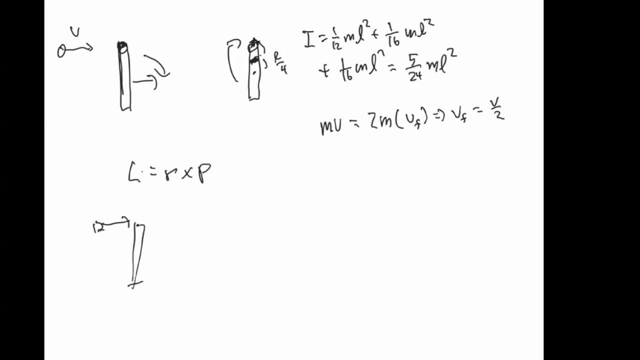 initially, our mass is the only thing that's moving, so it's the only thing that has momentum and it has mv of momentum. And remember, our reference point is right here. So this is our r And so this r cross p is basically just the.